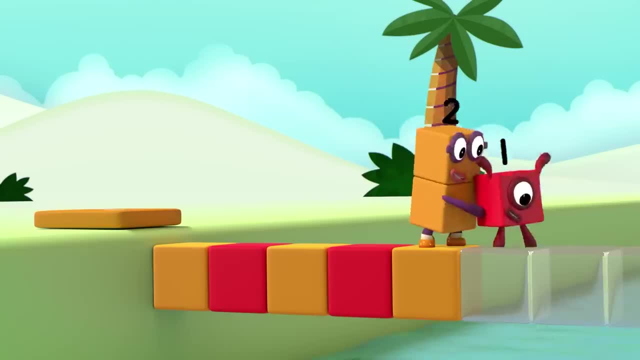 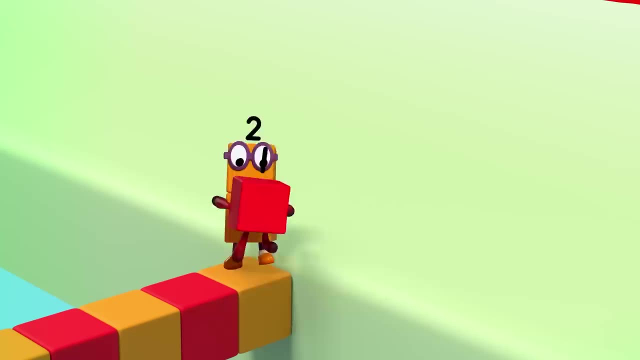 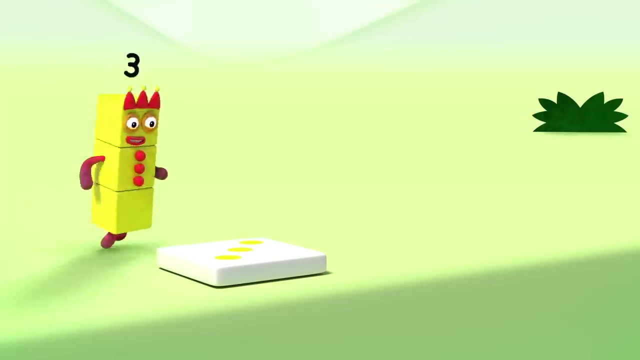 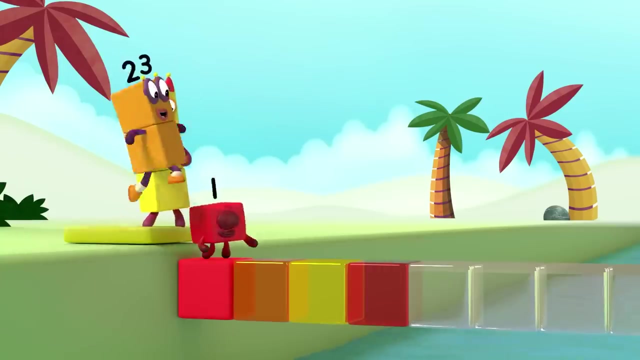 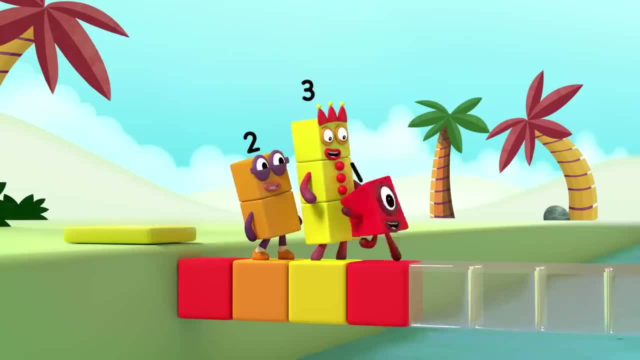 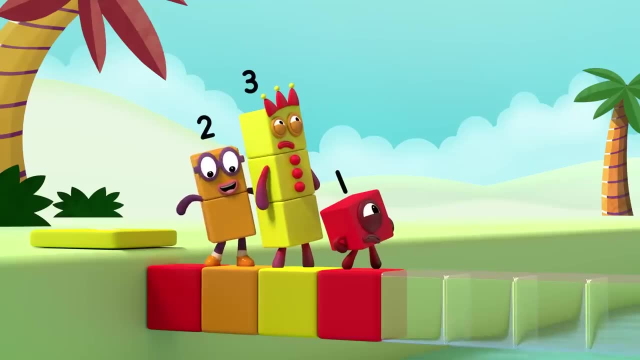 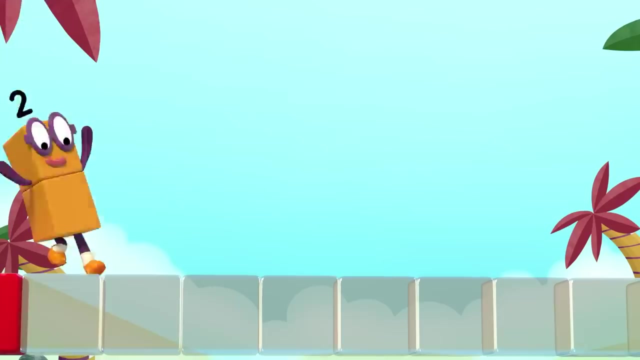 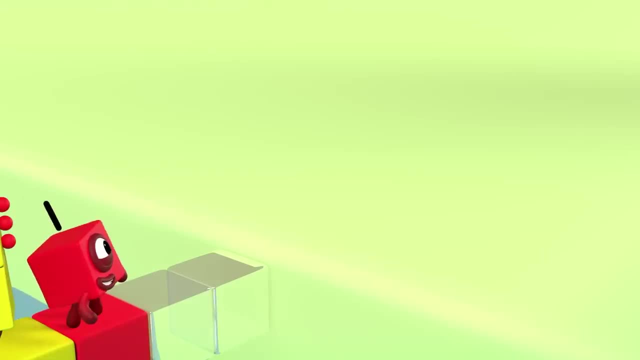 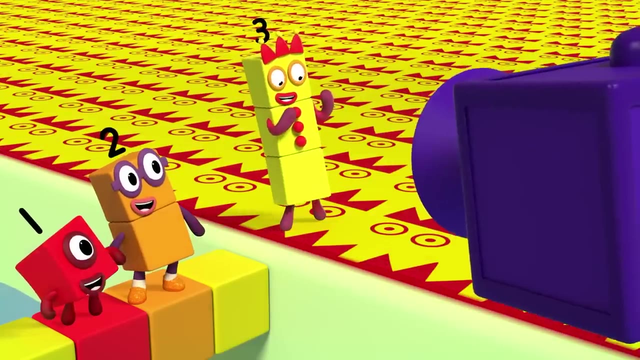 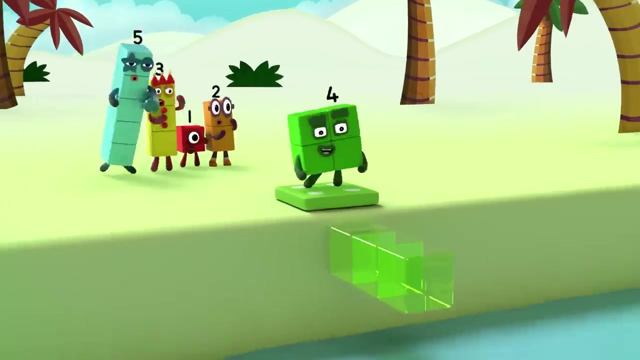 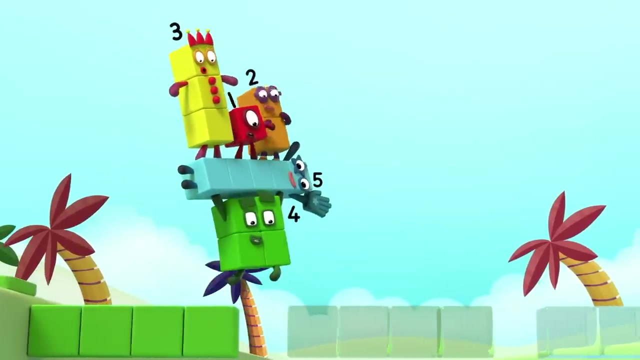 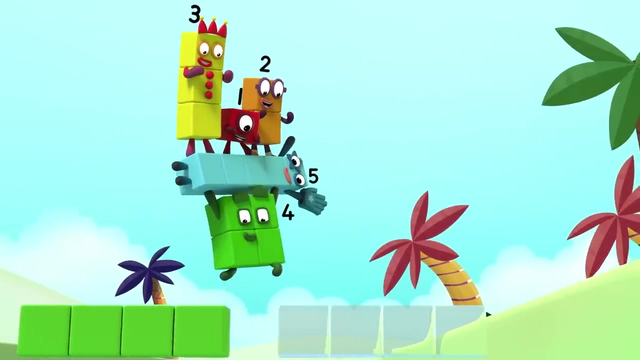 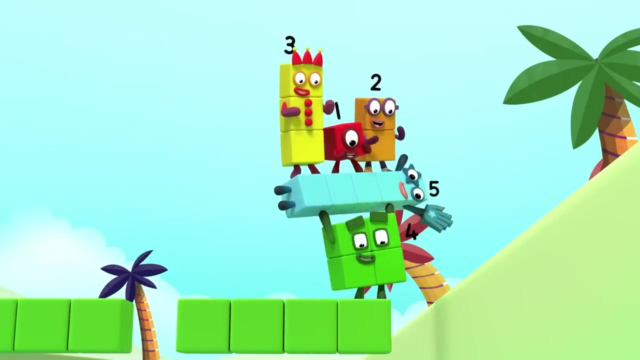 Two kelt, Red, Long Green, Orange, Orange, Yello, Ah, Green, Yellow, Green, Huh, Oh, Tell me the pattern. The pattern is It goes four greens, then a gap and repeat. 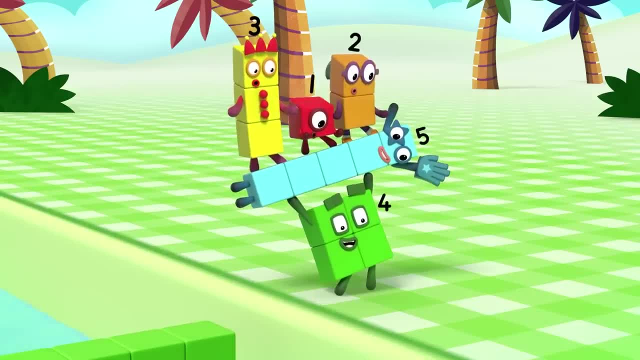 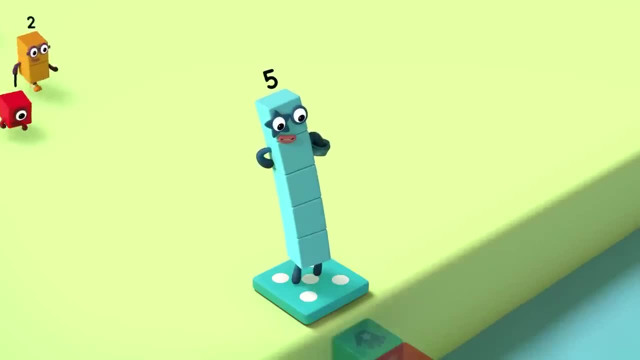 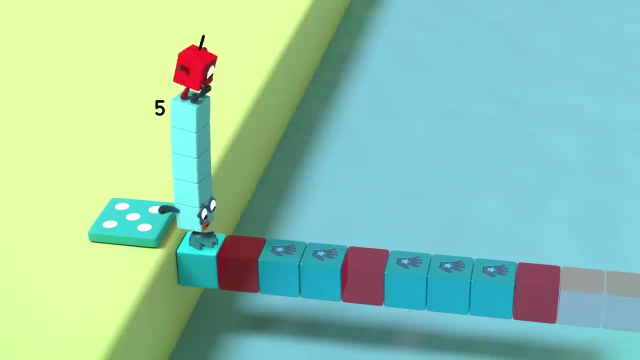 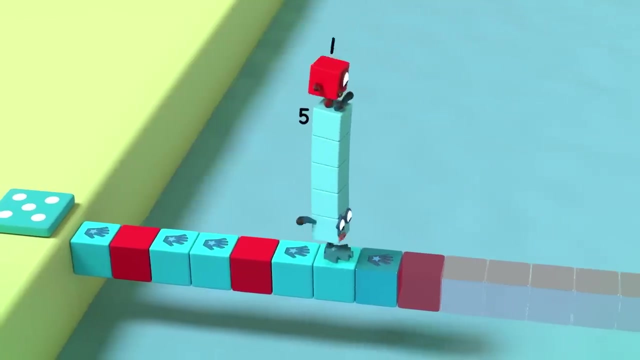 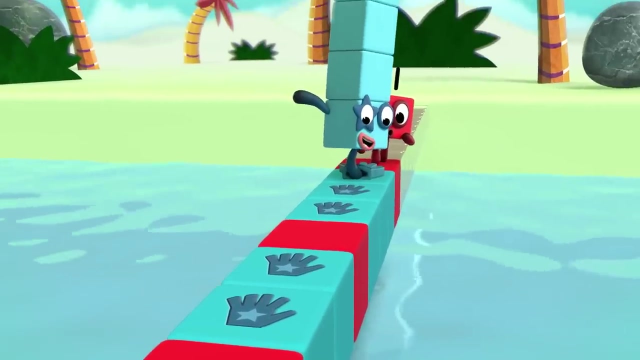 Pattern: unlocked Squares. Oh, Handprints, I love it. Hand Oh Hand Red. Oh Hand, hand Red. Hand, hand, hand Red. Stop, One hand, two hands, three hands Got it. 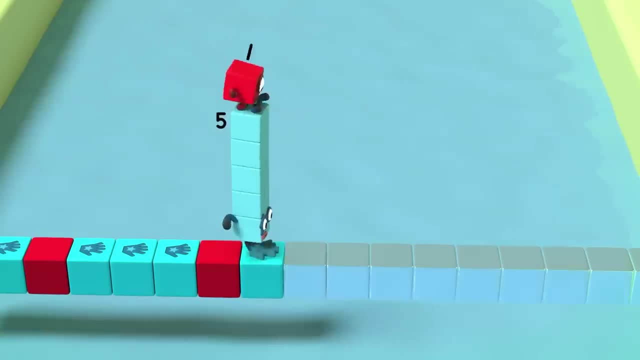 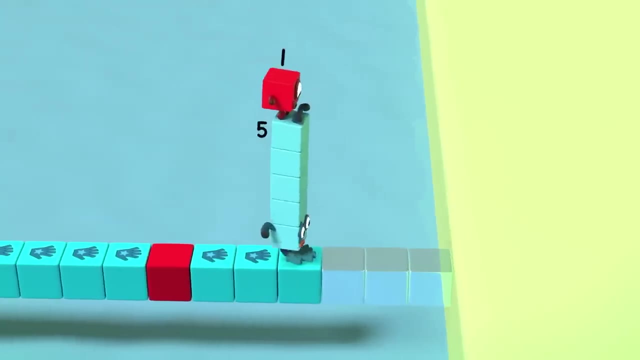 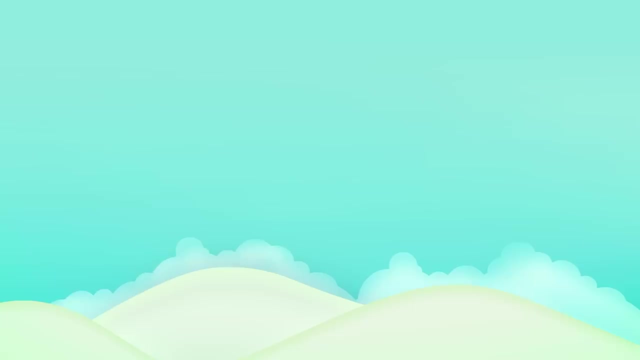 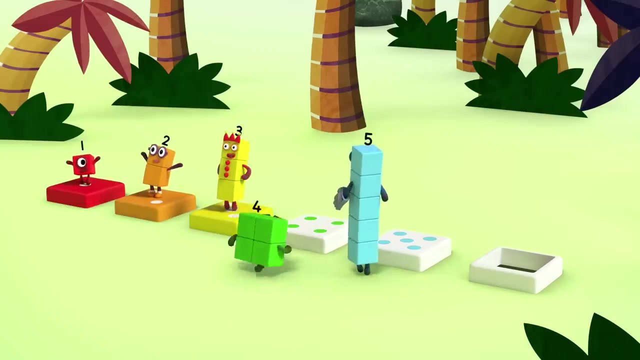 Next comes four hands: Hand hand, hand, hand, And then a red, One more hand each time, And then red Pattern unlocked. Look, we're at the centre. Oh yeah, One, two, three, four, five, six. 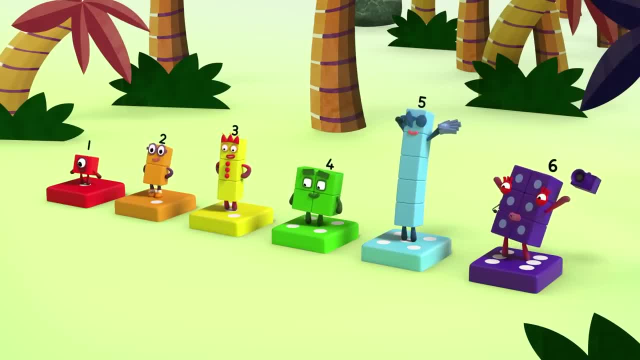 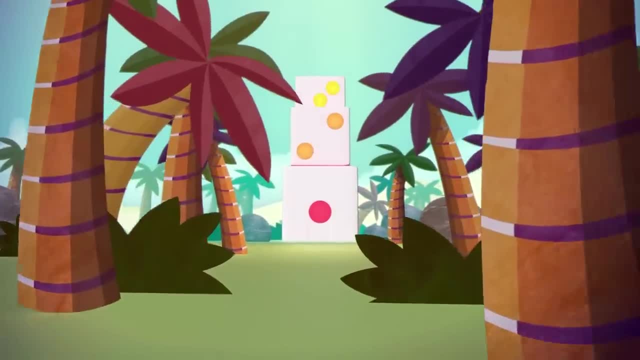 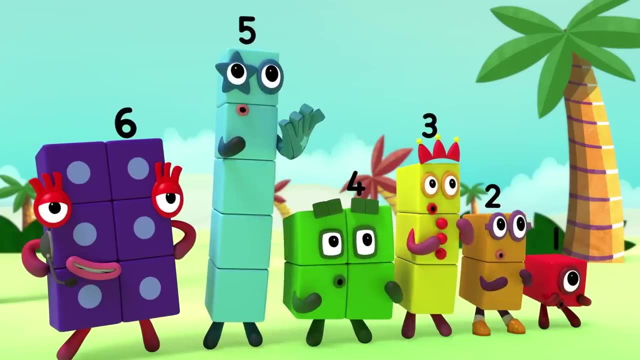 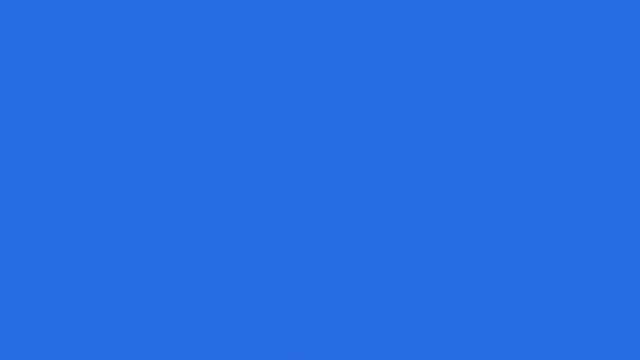 Pattern unlocked. You got across my pattern paths. Well done everyone. Now step into my pattern palace and let's all have some fun. Whoa, Whoa, Pattern palace unlocked. Woo-hoo, Yes, MUSIC PLAYS, Ahem. 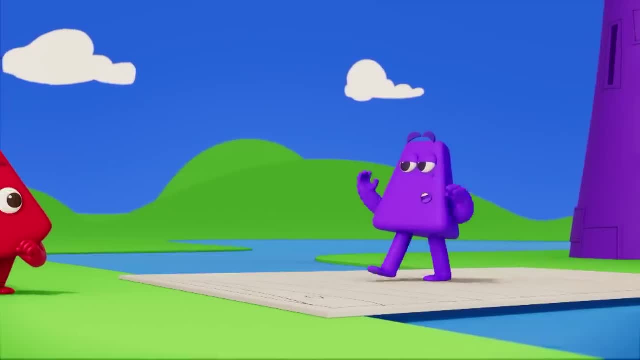 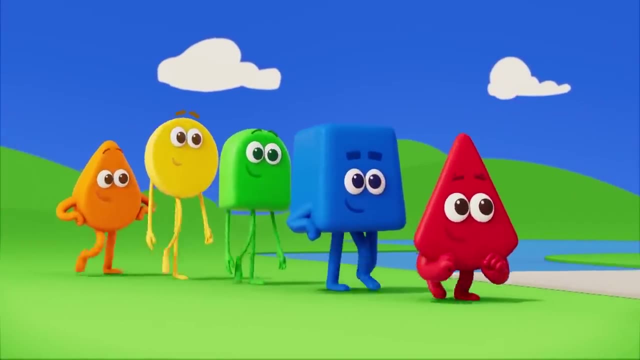 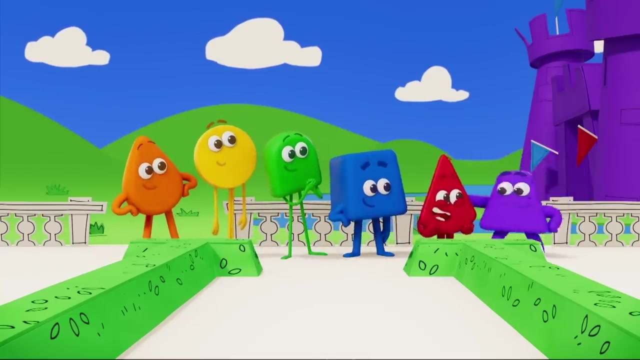 Welcome Colour Blocks. I imagine you're wondering why you're here. I, Purple, have had an amazing idea. You can all help me decorate my castle garden. I've made a little practice space for each of you to invent a wonderful new pattern. 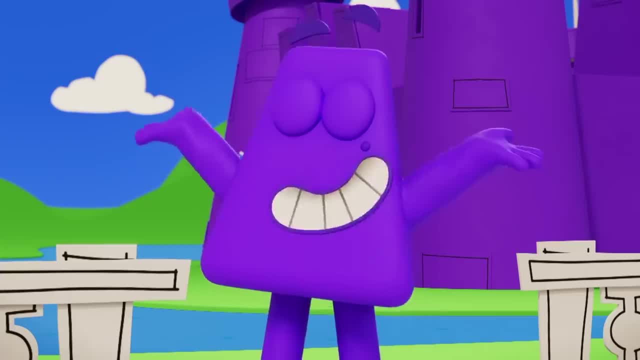 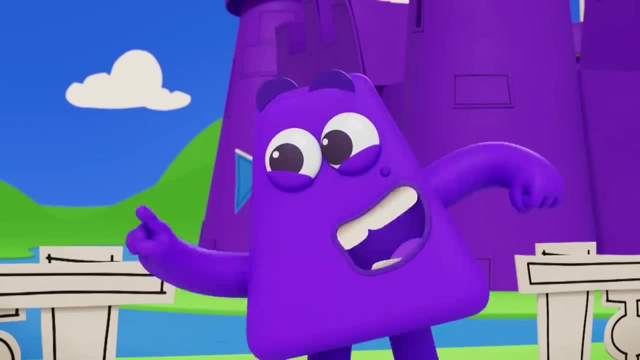 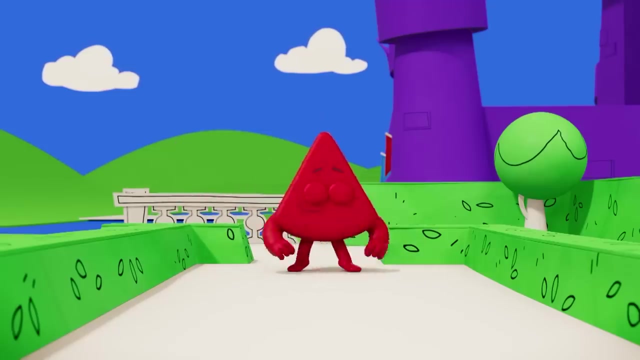 Whichever one I like the most, I shall use to decorate my gardens. It's a competition, Cool, Let the pattern competition begin. Oh, Yay, Time to make an awesome pattern, Exciting, Ha-ha-ha. Wait, what is a pattern? 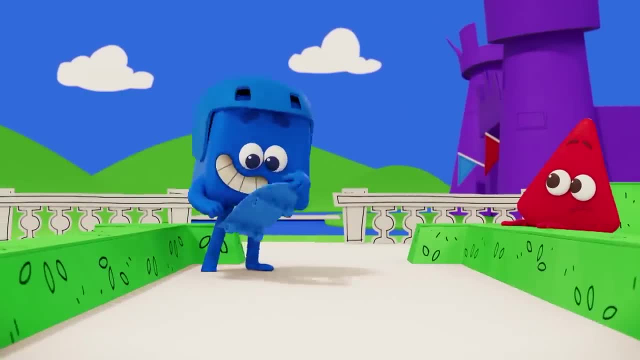 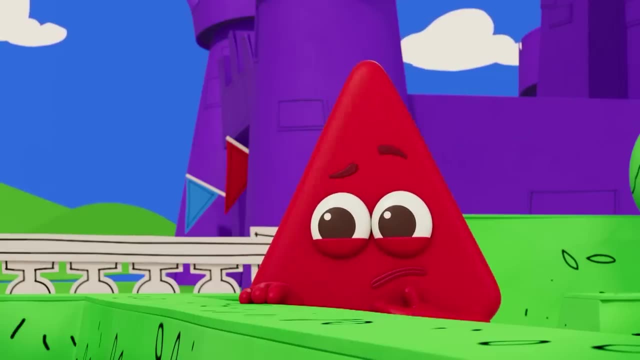 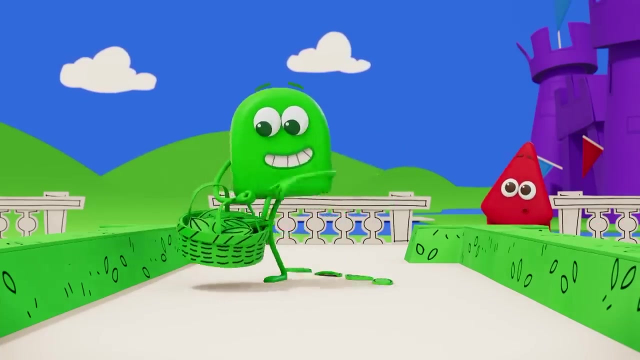 Um Check this out: Red Blue Stripes, Stripes, Stripes. I've got an idea for a pattern. Huh, Green, I can make a pattern. Zig Zag, Zig, Zag, Zig Zag. 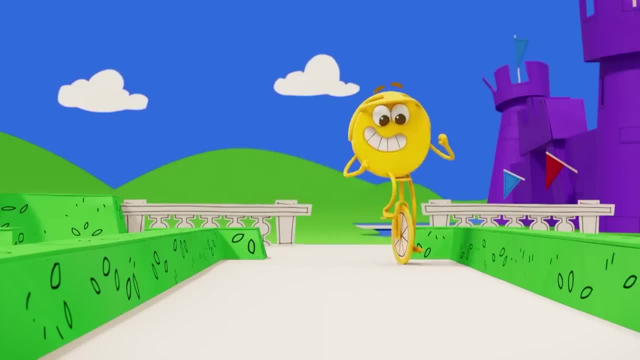 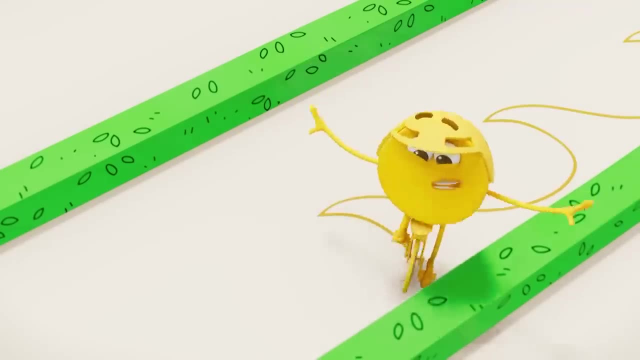 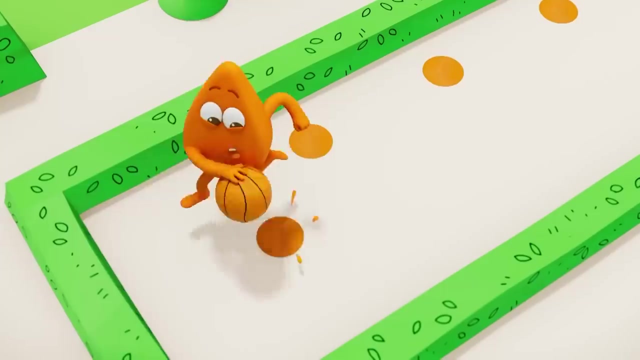 Zig Ha-ha-ha. Yellow Wave. Wave Wave Ha-ha-ha- This makes me happy. Wave Wave Ha-ha-ha. I'm making a high-energy, spotty pattern, Spot Gap. 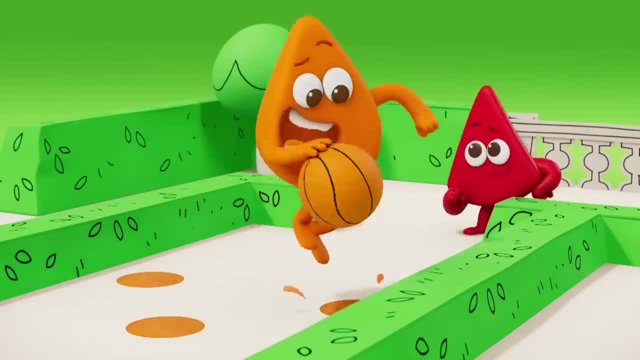 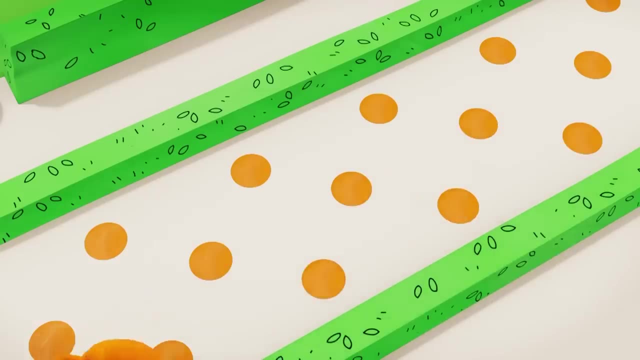 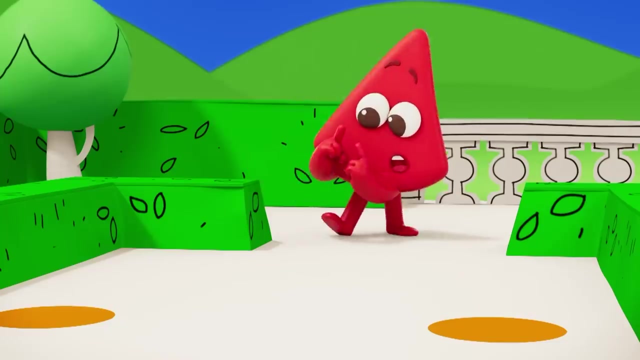 Spot, Gap, Spot. Hmm, Again and again. Spot, Gap, Spot. Ooh, I get it. A pattern is the same thing again and again: Making something that looks nice In a spotty pattern. you repeat the spots. 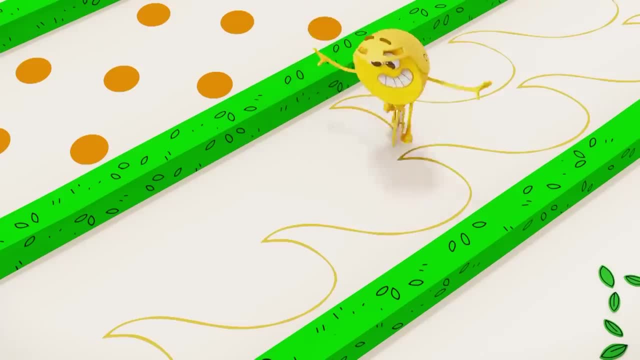 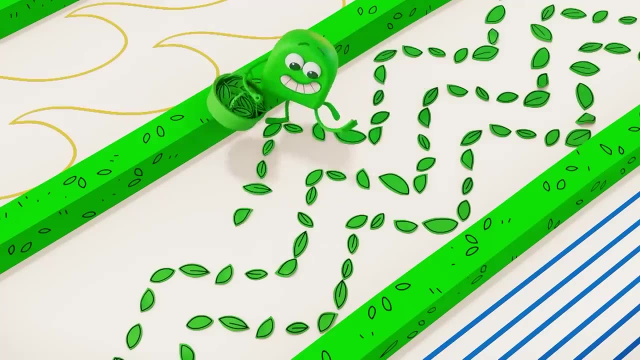 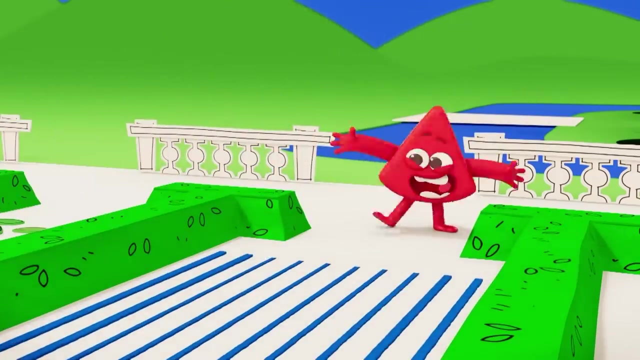 And in a wavy pattern, you repeat the wave Ha-ha-ha. The line zits and zags, And so does the next line and the next. They repeat Stripes. Again and again, the stripes repeat Ha-ha-ha. 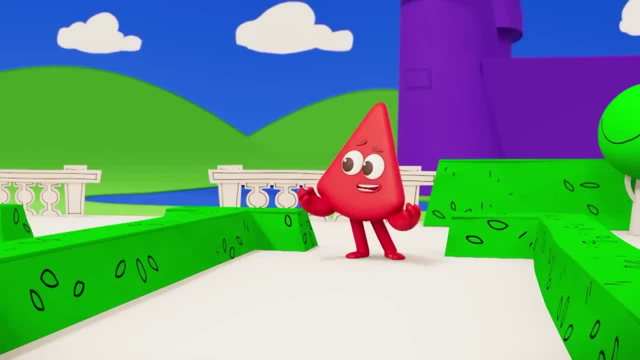 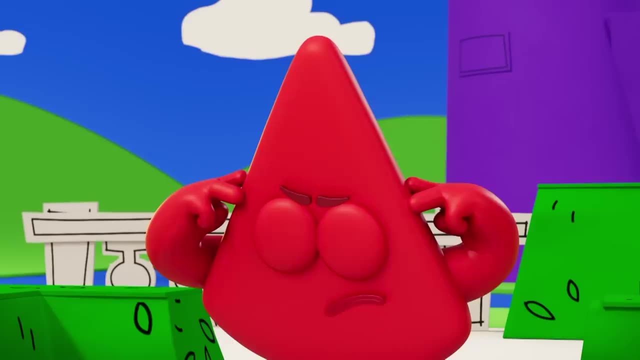 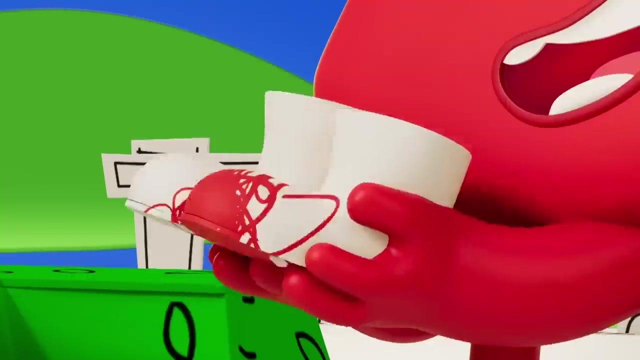 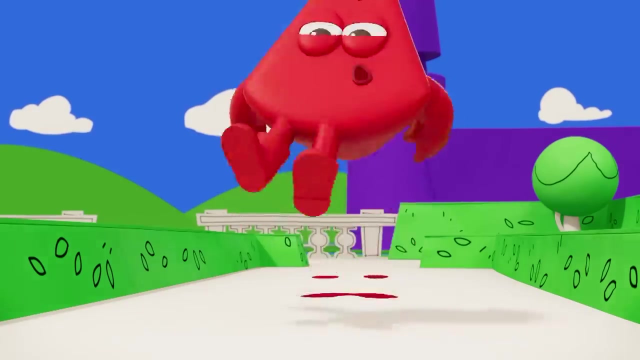 Hmm, Everyone's already got such exciting patterns. What type of pattern should I make? Think, Red, Think. I know I'll make a splat pattern: Red Ha-ha, Big splat. Two splats, Big splat. 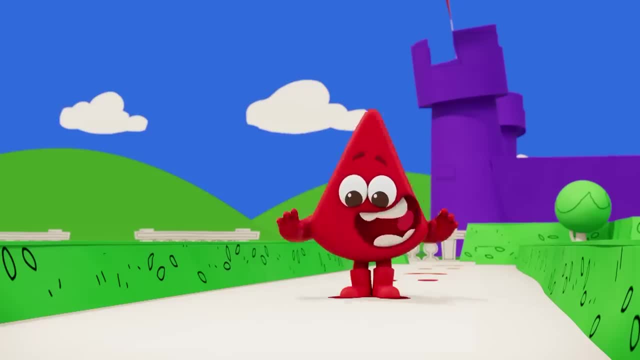 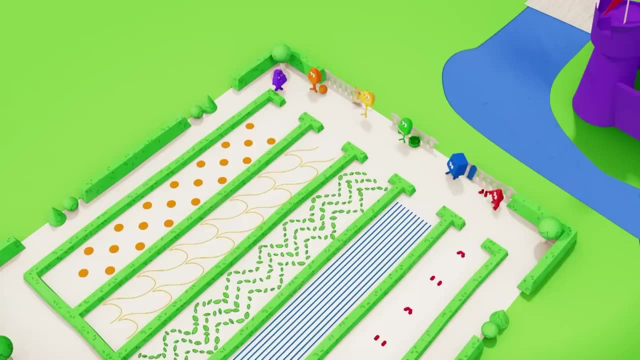 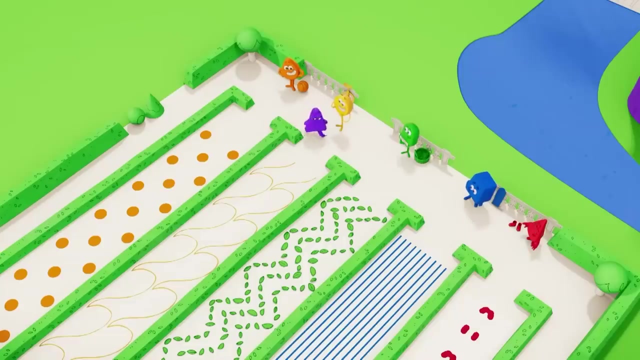 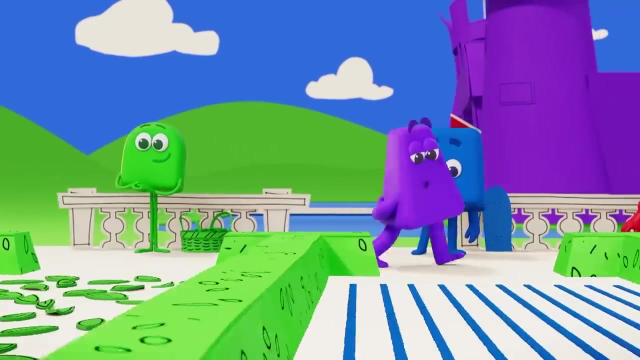 Two splats, Big splat Ha-ha-ha. Repeat: Two splats Ha. Time to judge your patterns. Hmm, Yes, Ooh, Yes Ooh, I like that one. Ooh, You followed the brief well. 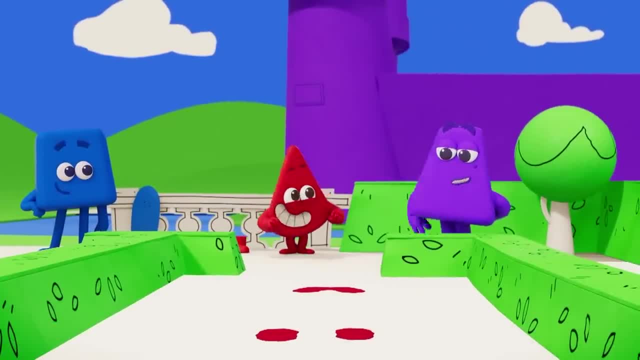 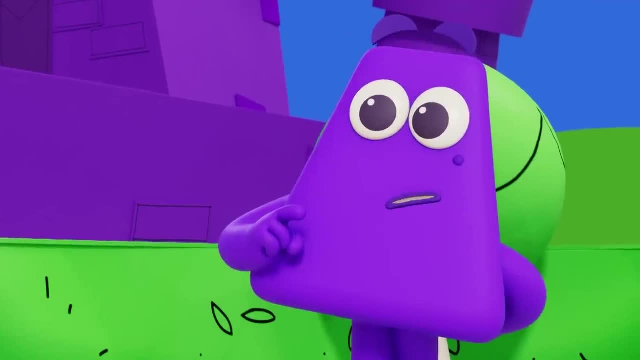 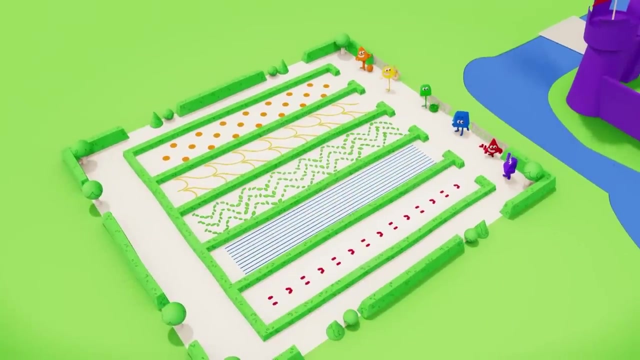 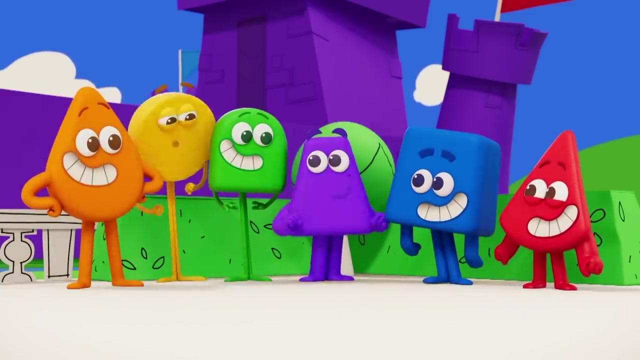 Hmm, Nice, Ha-ha, I have finally decided which pattern I like best. My favourite pattern is all of them, All of them. That's right. They're all wonderful, So why don't we put them all together? What? 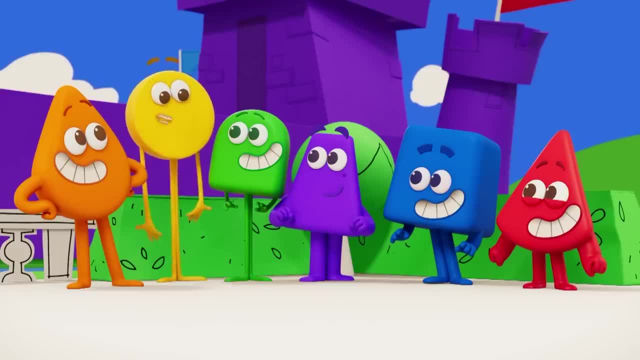 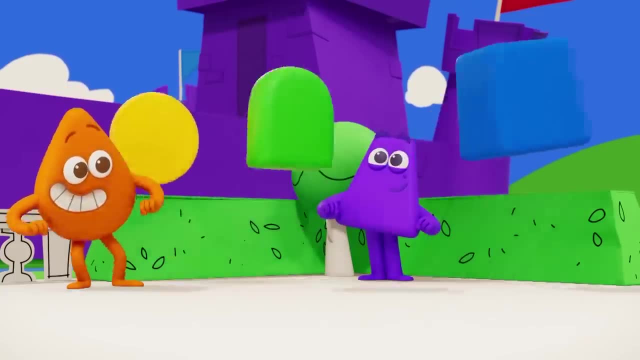 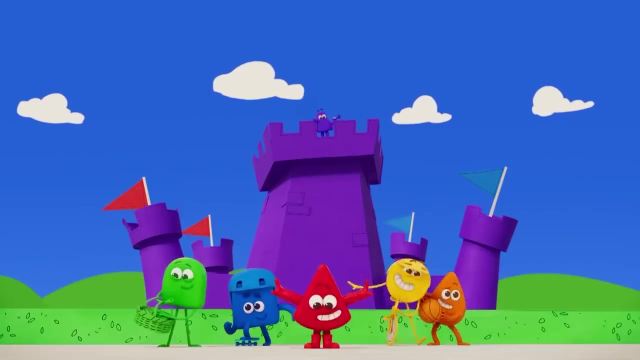 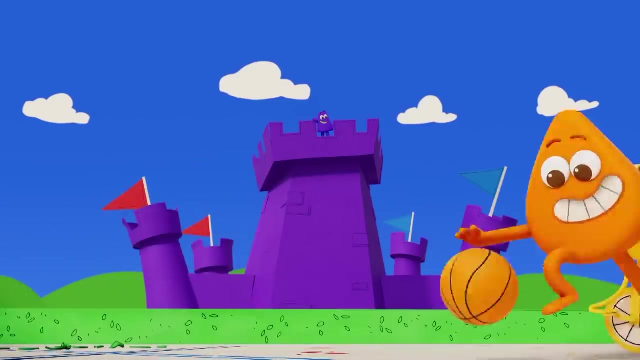 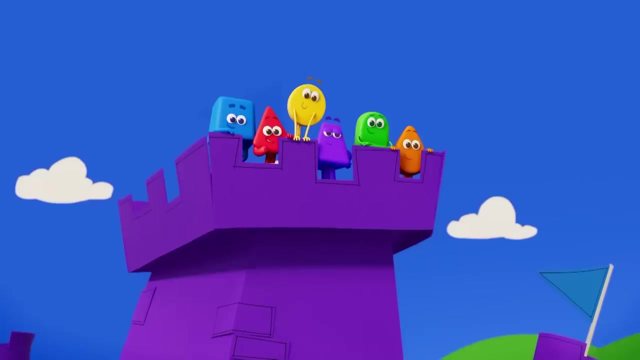 Make one big, super-duper, mega pattern. Wow, I think that's a great idea. Let's make patterns. Hoo-hoo, Sounds like fun. Ooh, jurisdictions are coming to fund us. You were right, Purple. 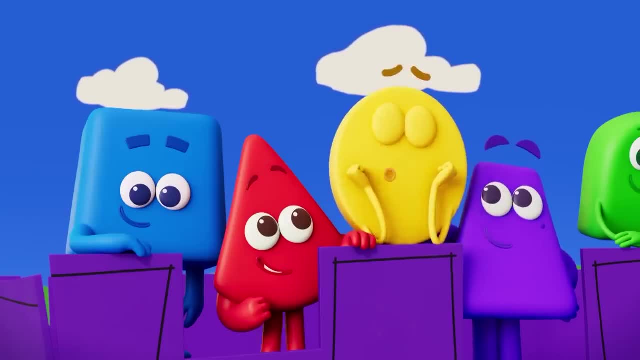 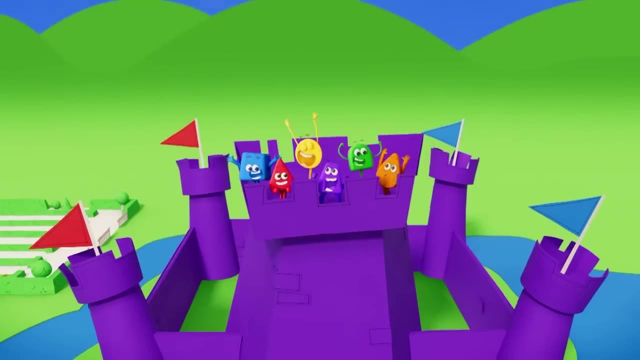 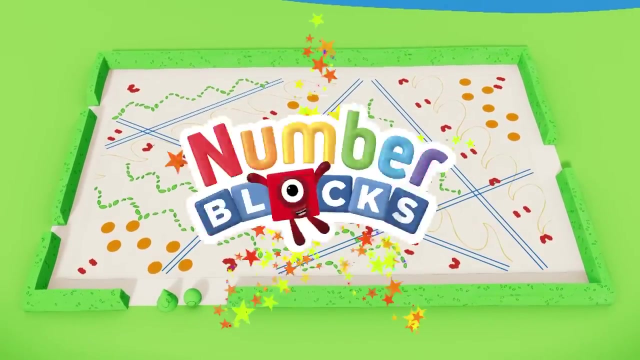 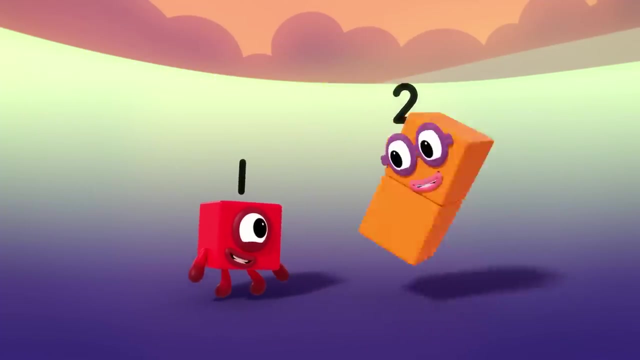 this really is the best pattern ever, And there are lots more. we can invent One, two and again One, two. Your turn One. I can't do it. What was that? That way? Come on, Wait, Looks familiar. 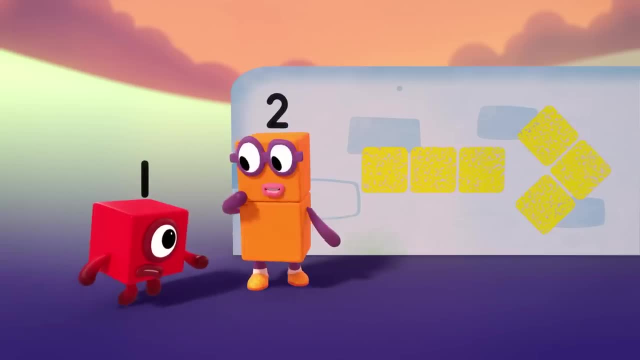 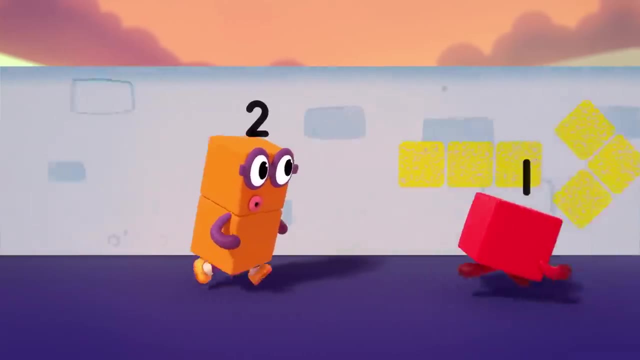 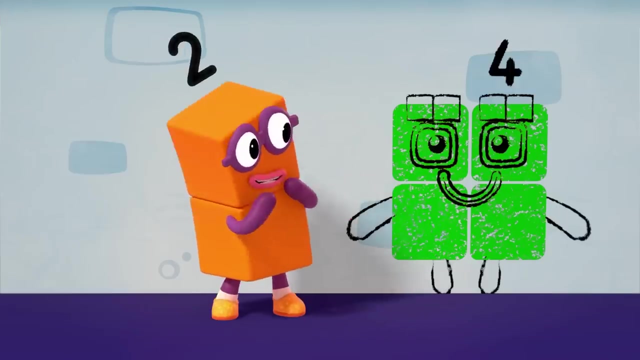 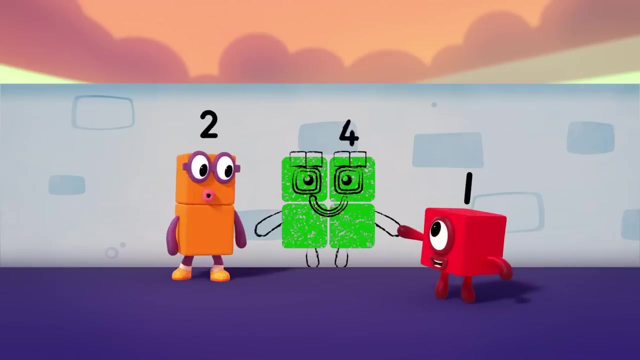 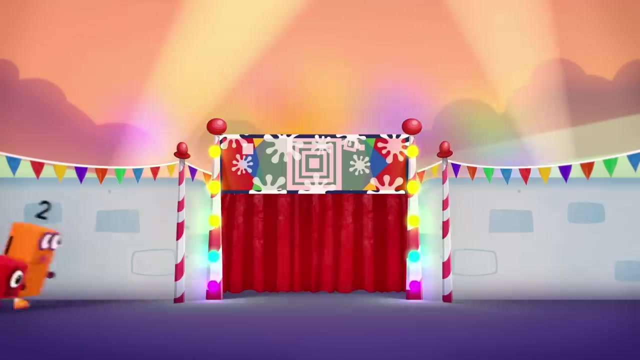 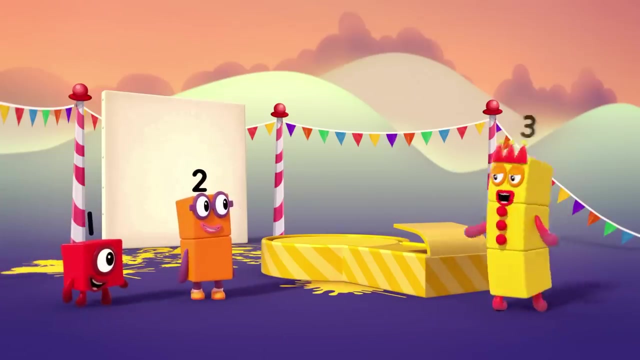 It's pointing to the sounds. Quick, Hey, it's four, Four, Four. Okay, Four, Four. What are we playing? musical statues? A painting, A painting of four. I knew that. But what's that? Welcome, welcome, welcome to my new Stampoline Park. 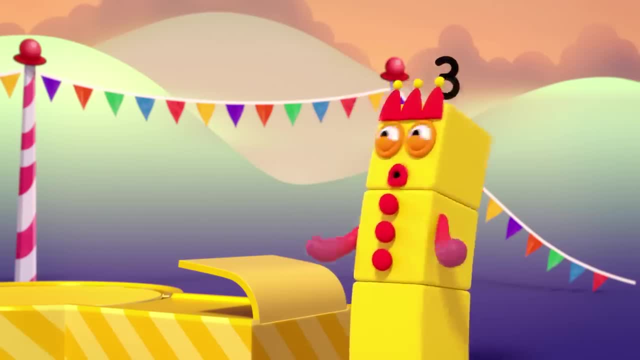 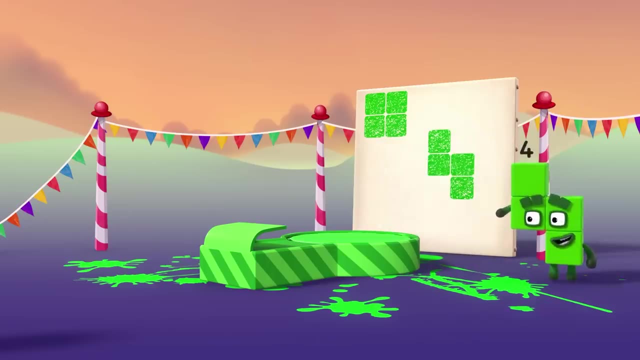 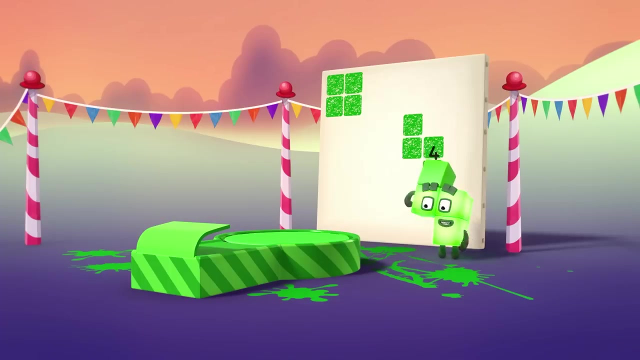 Don't you mean trampoline? No, no, no, Look, Whee, Ooh, that was fun. Four Is that you? Of course, it is One, two, three, four, Four blocks, See Whee. 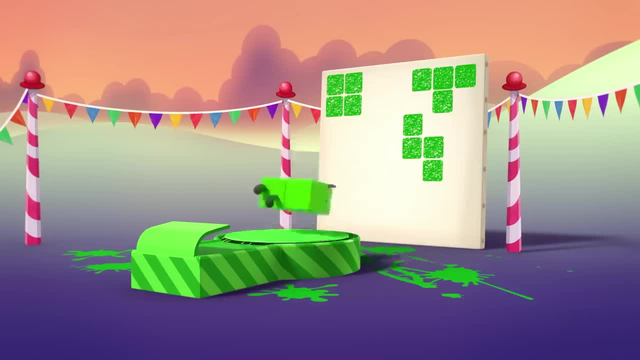 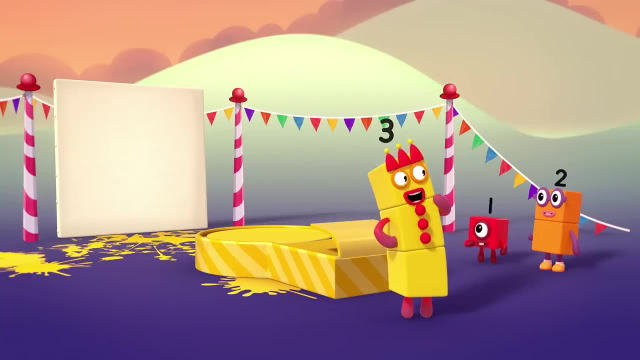 Whatever way round I go, I'm still four. Whee, Look at me, Whee, I'm still three. Whee, Ba, ba, ba, Ooh, Not bad. You think that's amazing? You should see five. 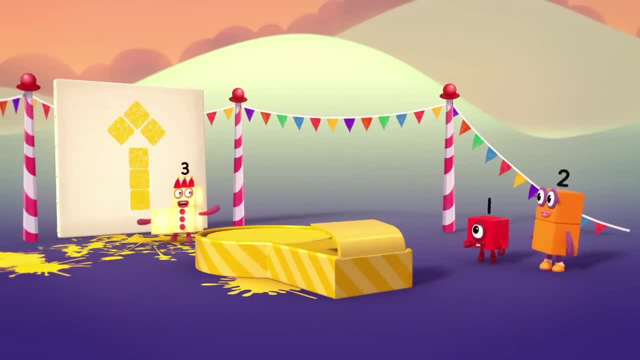 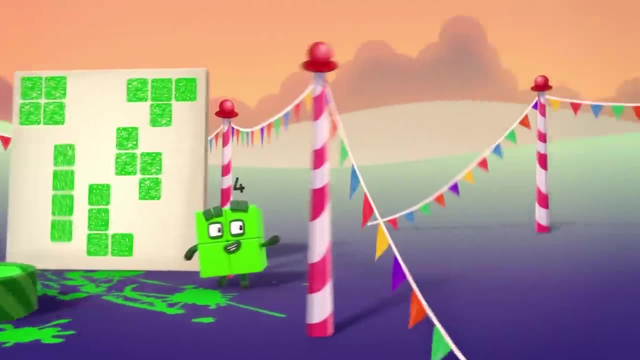 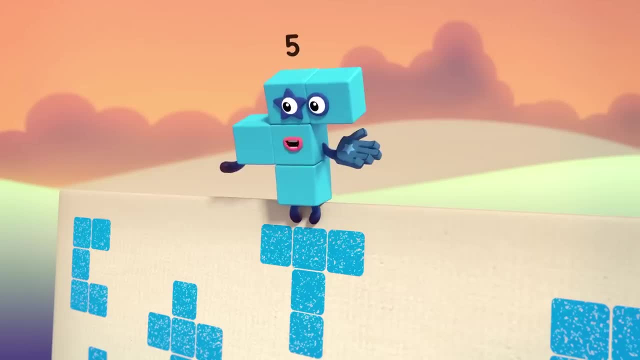 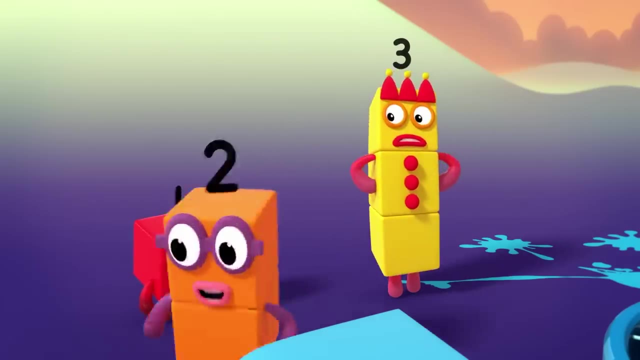 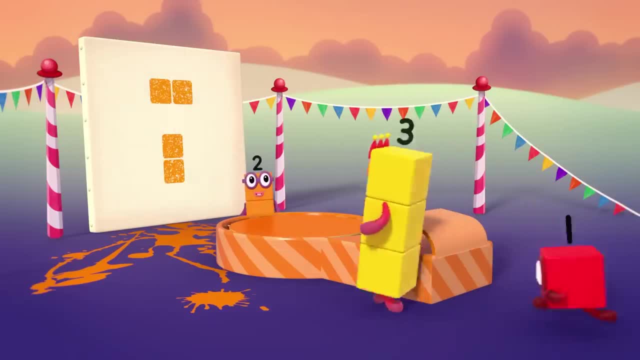 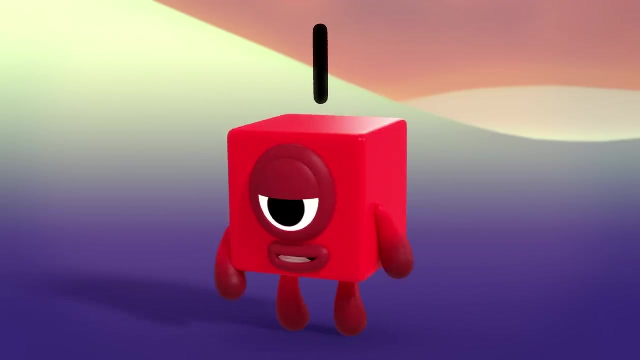 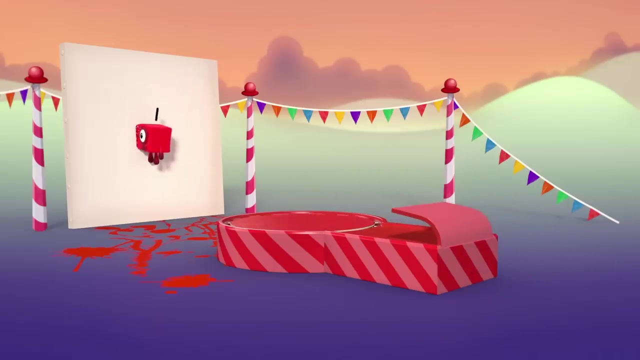 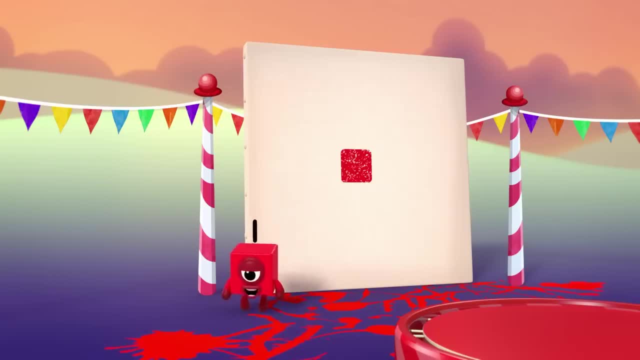 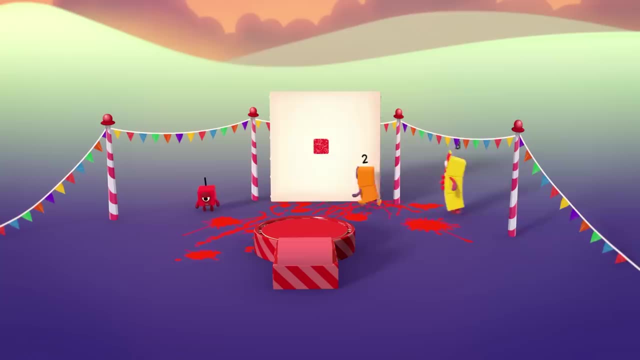 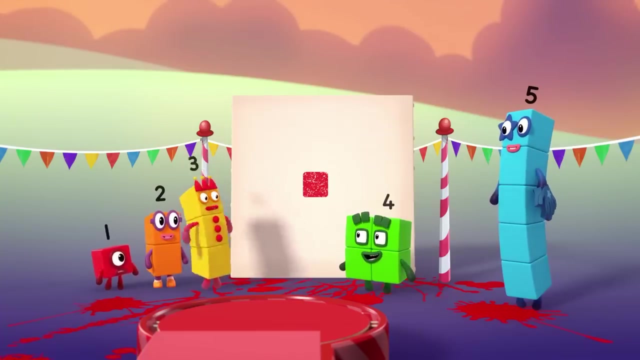 Not very exciting compared to all of you. Now, now, now You're forgetting something. One, two, three, Boo, Hey. One plus one plus one plus one equals four. Every big shape is made up of lots of little ones. 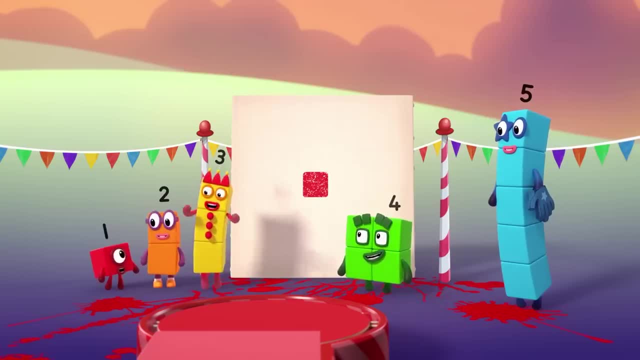 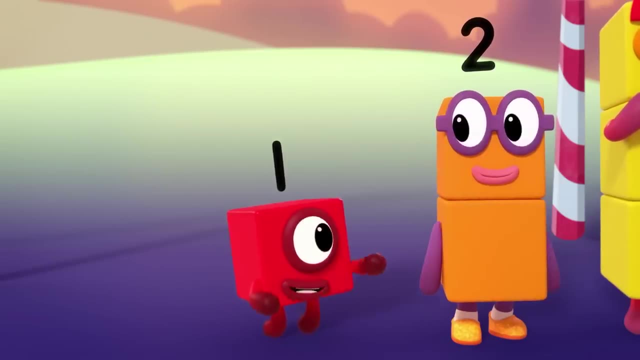 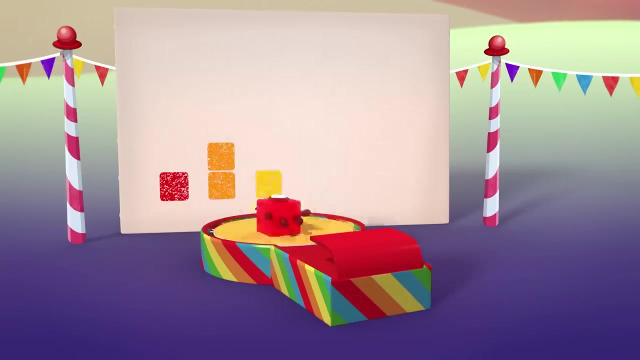 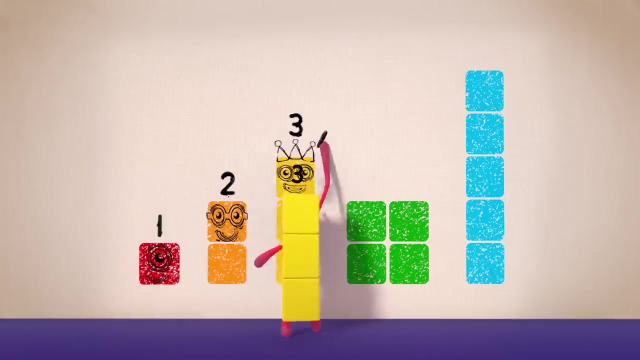 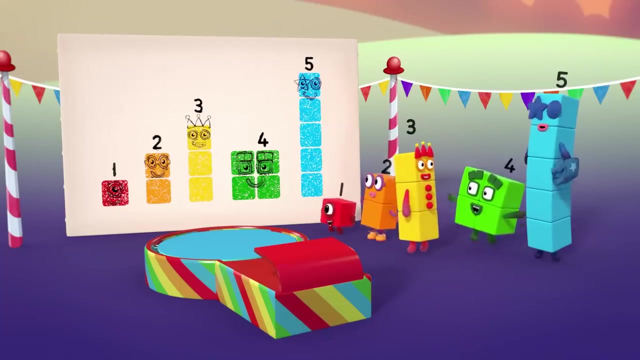 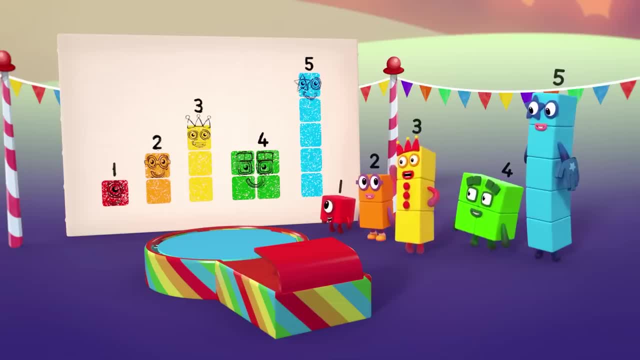 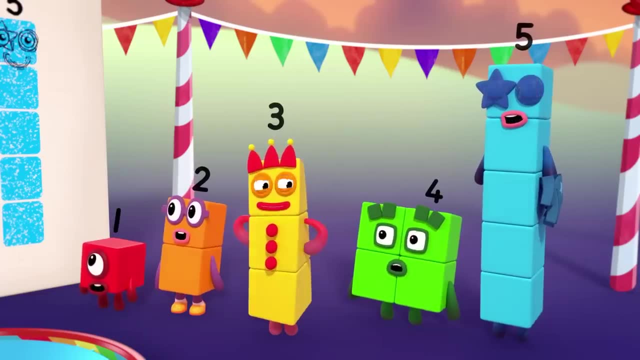 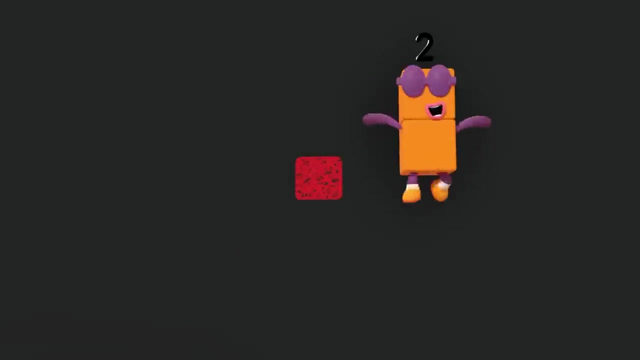 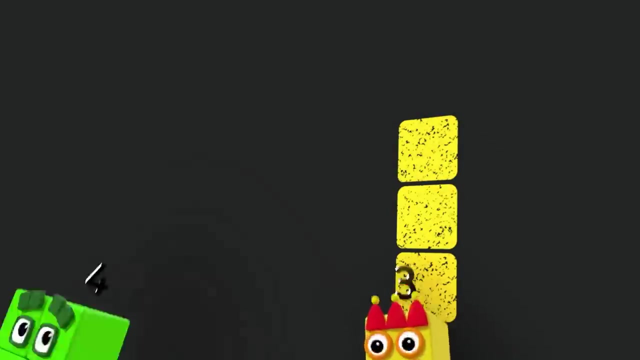 And just in time for the grand finale, What better way to celebrate opening my new park than with fireworks? Ooh, May I present the Sky At Night. Whoo Hooray, Hooray, Hooray, Hooray. 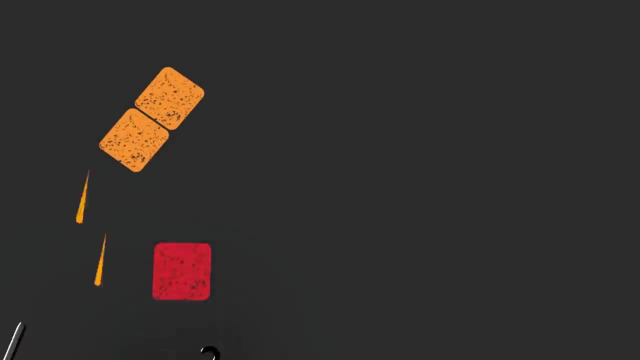 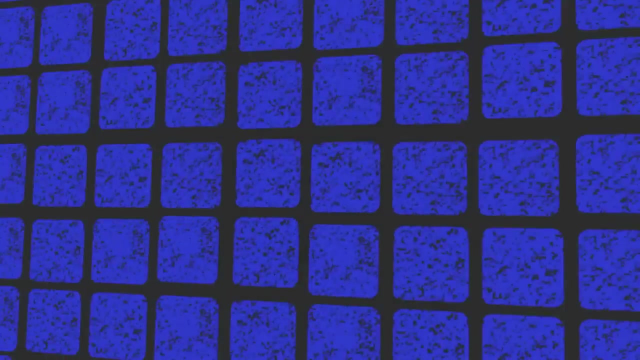 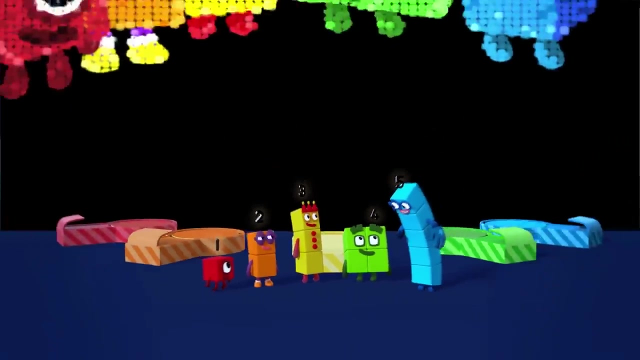 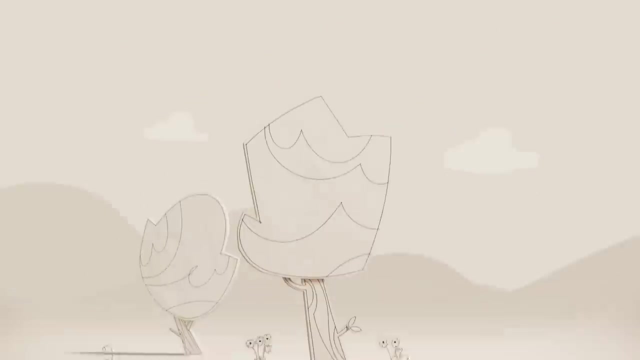 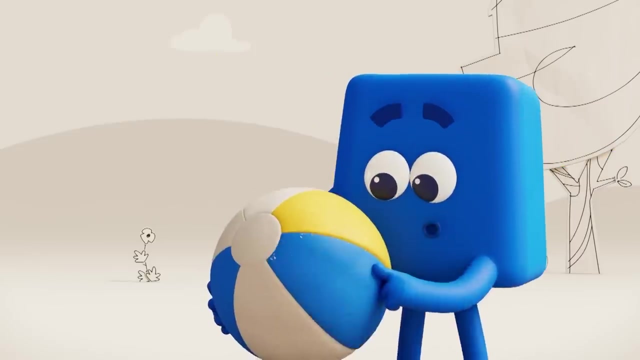 Yeah, Yeah, You see one. When we all work together, the sky's the limit. Hooray, Hooray, Hooray, Hooray, ho hooray. Yellow, Blue, Cool, Yellow. 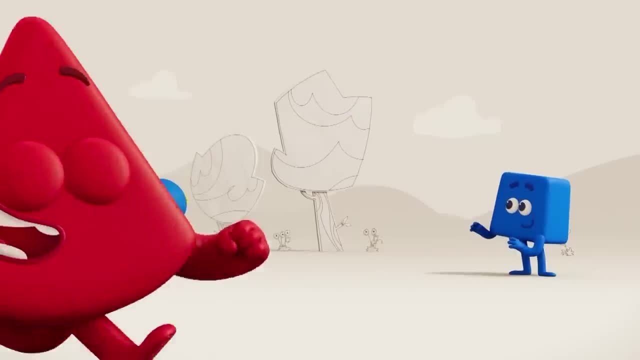 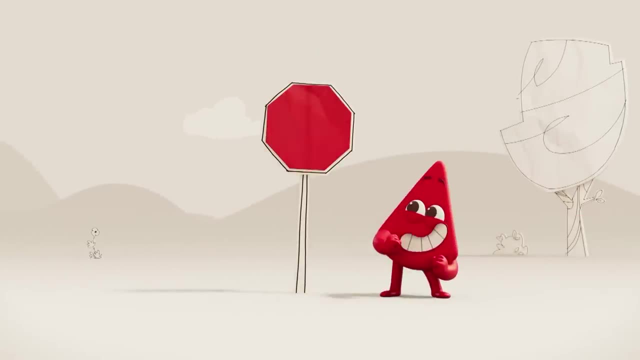 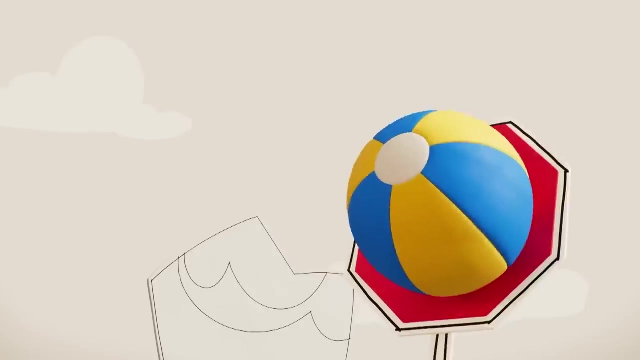 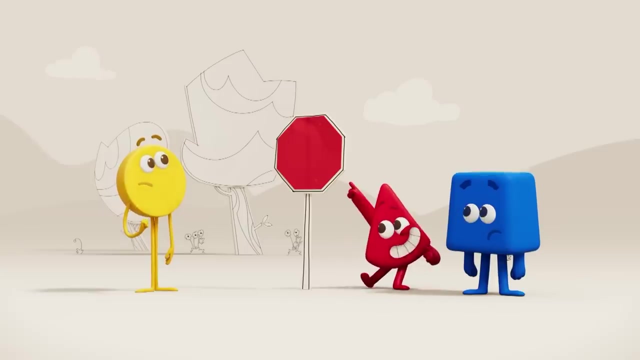 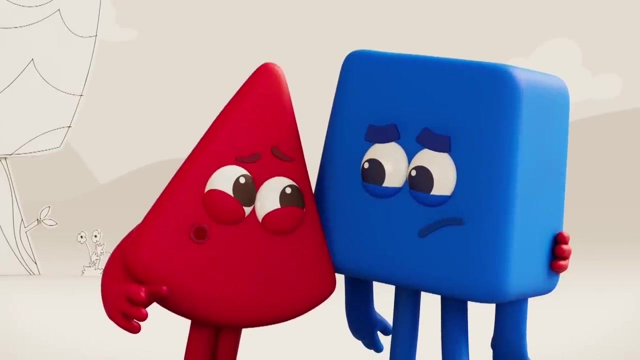 Blue, I'm red. Ooh Red, Stop, Huh. Red means stop. When you see a red stop sign like this, you have to stop. So we have to stop our game, Not cool? Oh sorry, friends. 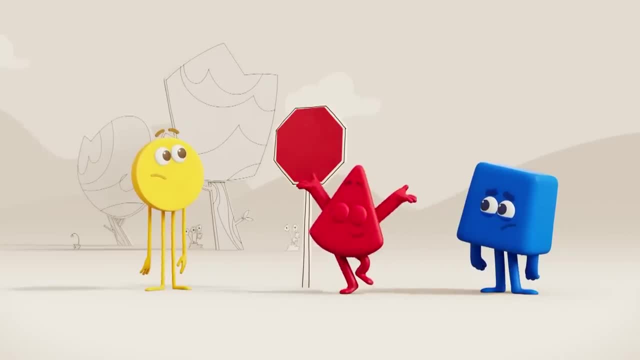 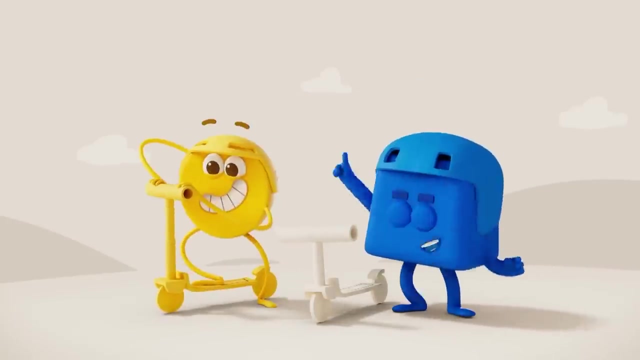 I can't help myself. Red means stop, Never mind Blue, I'm happy to play something else. Oh look, Scooters. Yay, Yellow, Blue, Let's play, Let's go, Woo-hoo-hoo. 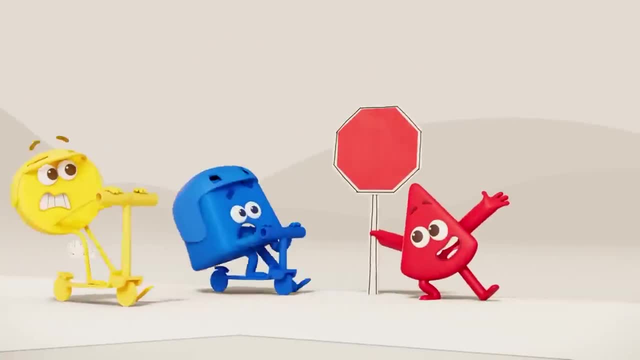 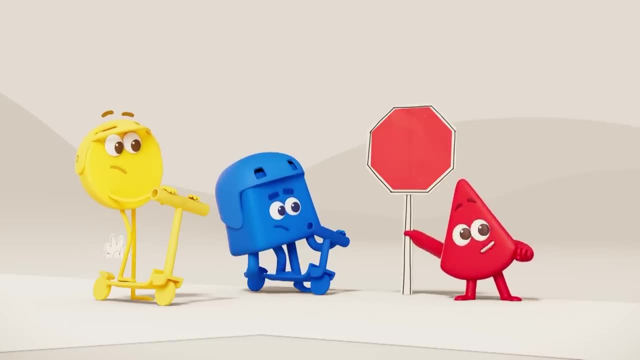 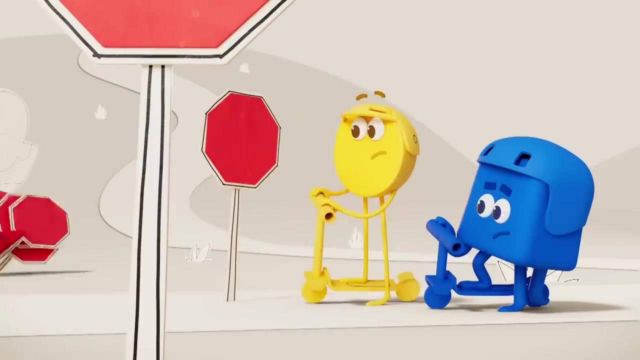 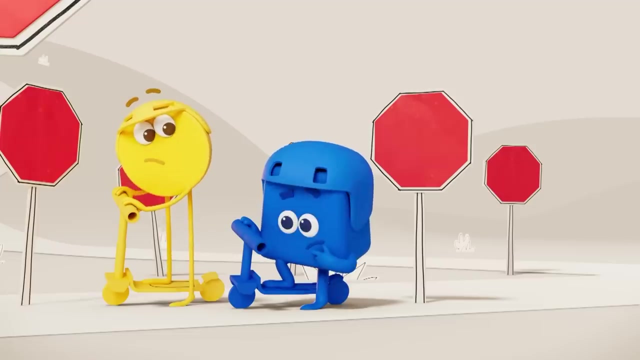 Woo-hoo-hoo, Whee. Red means stop. Uh, not again. Sorry, Can't stop myself And I've got lots of these to put up today. Bye, Oh dearie. Hmm, Time to put a stop. 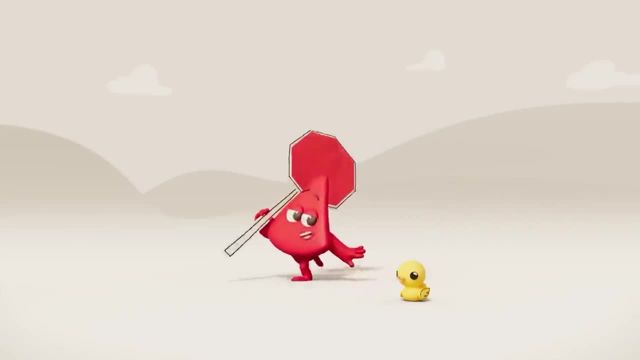 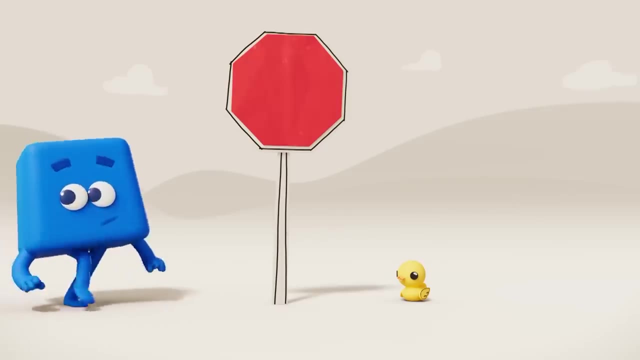 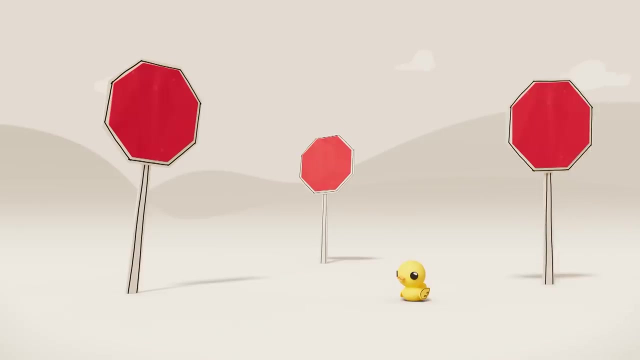 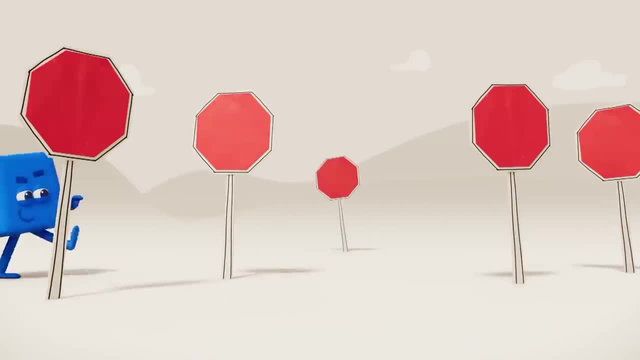 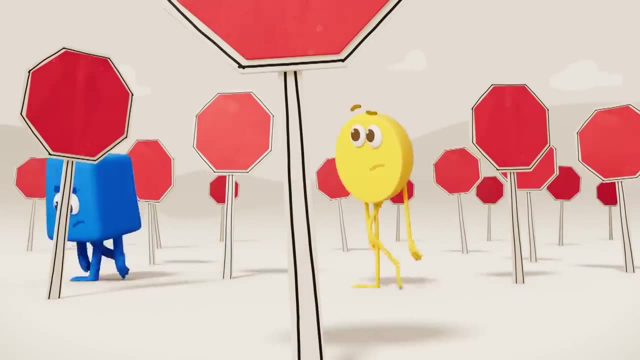 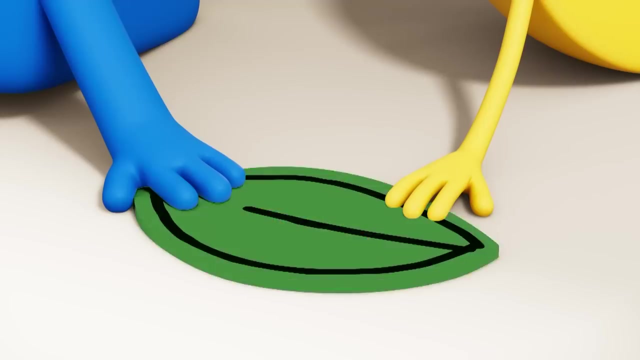 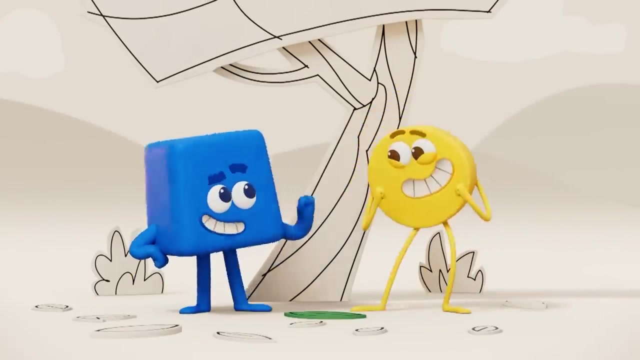 Red, Red, Red, red, red, red, red. Looks like we can't stop red. Oh well, Huh, Look what happened when our colours mixed. Oh, do you think, Shall we Blue and yellow mix to make green? 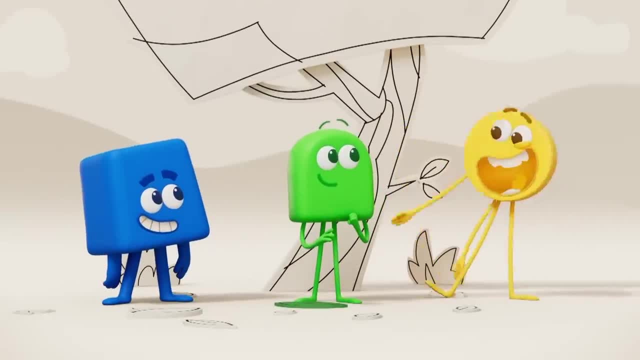 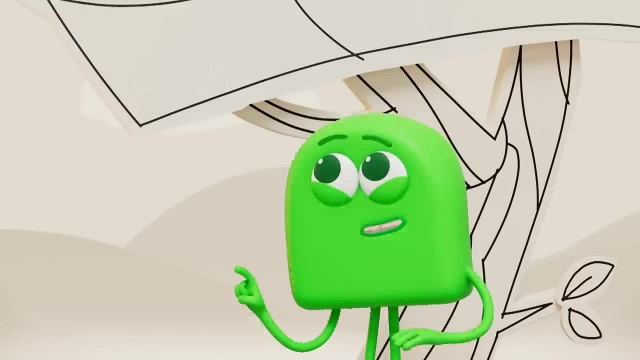 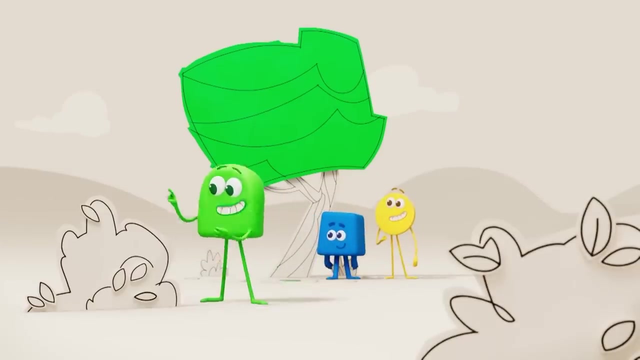 Wow, I didn't expect that, And I didn't expect me other colours. So tell us about green. Green is in growing things, Naturally. I like nature. All these plants are green, Oh, and this frog, Frog, Green. 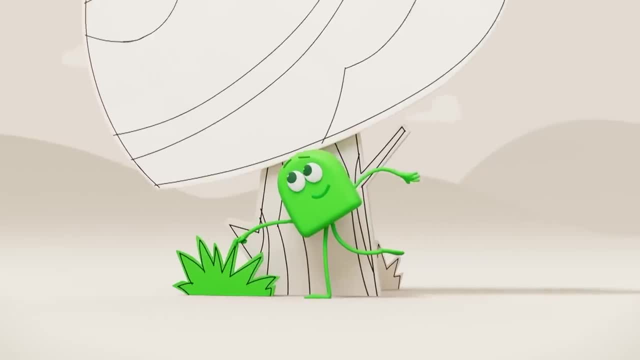 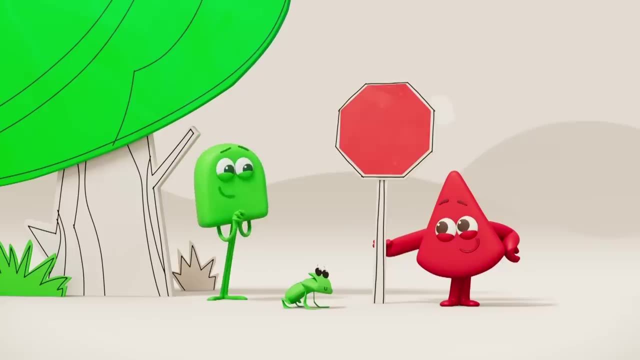 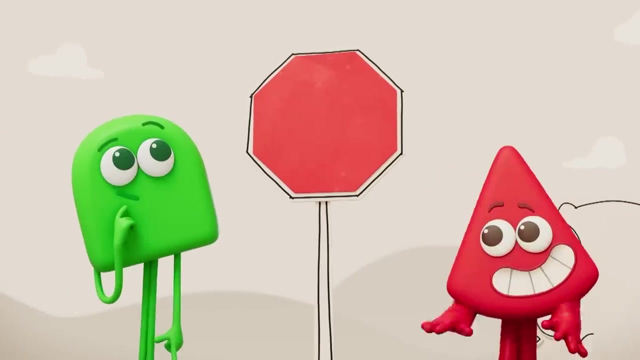 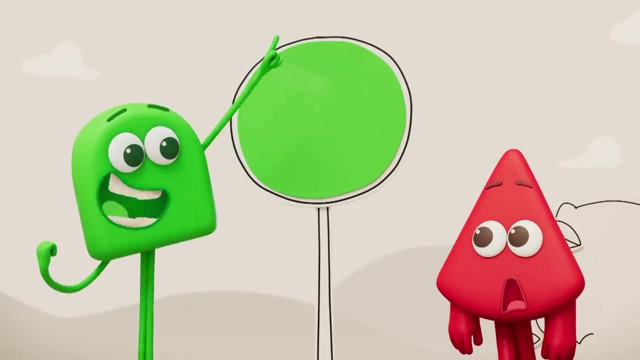 Green. Red means stop. Oh right, Pleased to meet you. I'm green, I'm red, And this means stop. And now it's green, Which means it's a go sign. Green means go, Go frog. 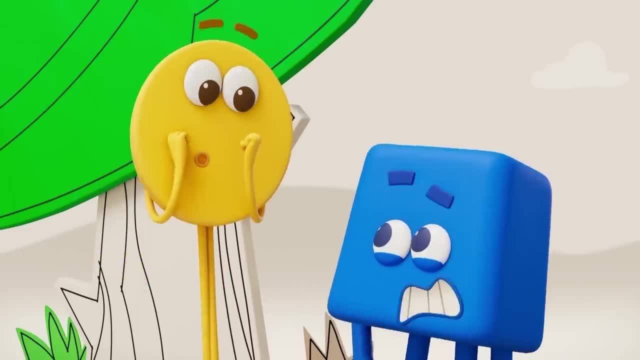 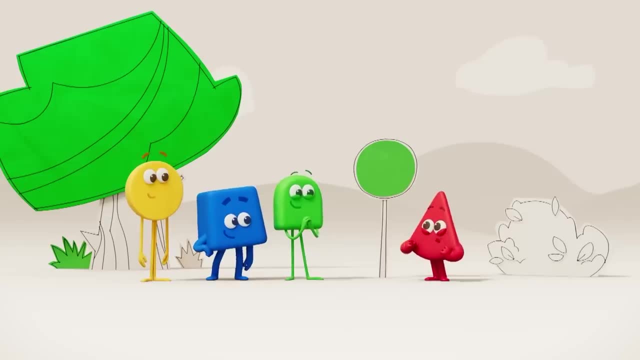 Go frog. And now it's green. Green means go, Oh, Oh, Oh, Oh, Oh, Oh. Brilliant, It's given me an idea for an exciting new game. Green means go, Haha, Yay, Ha. 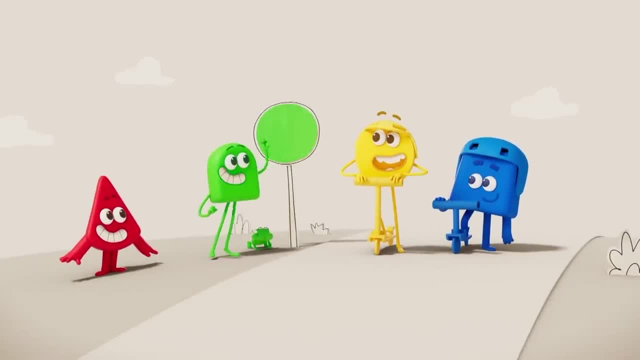 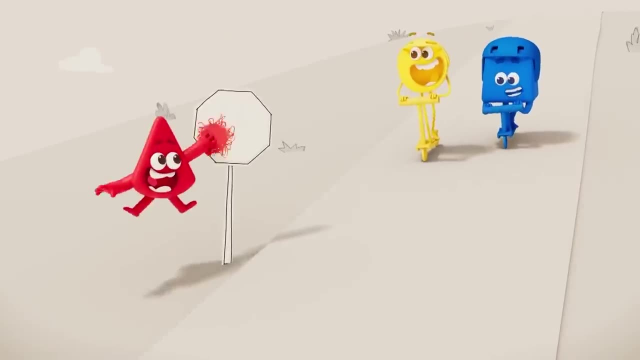 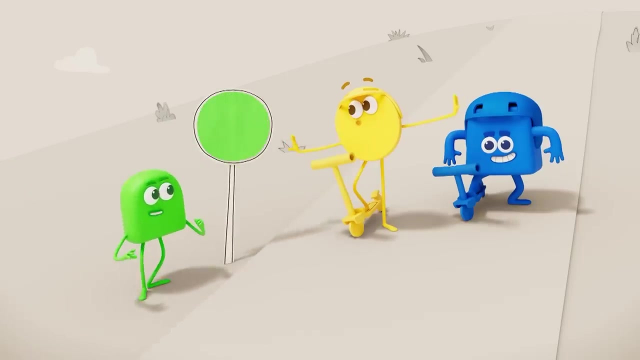 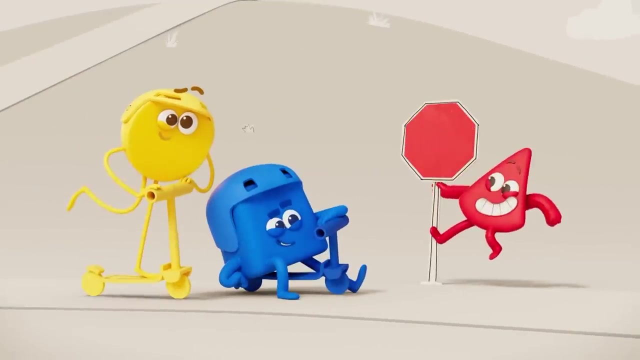 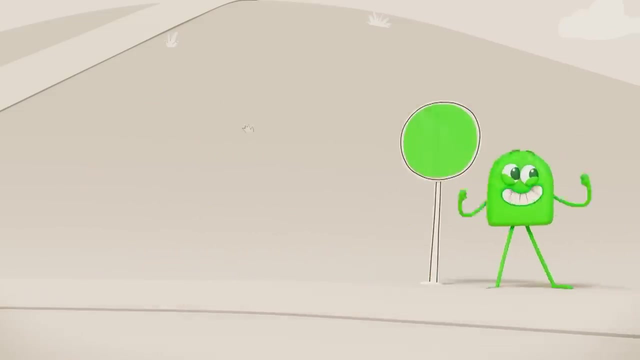 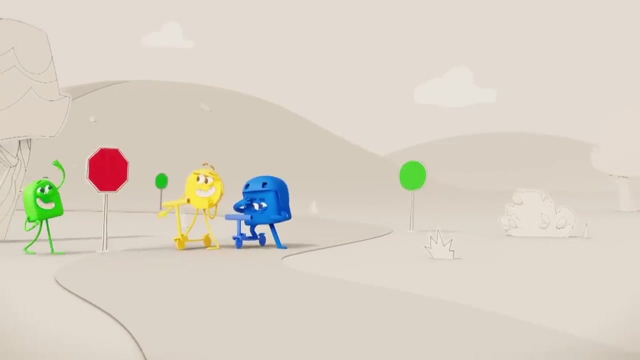 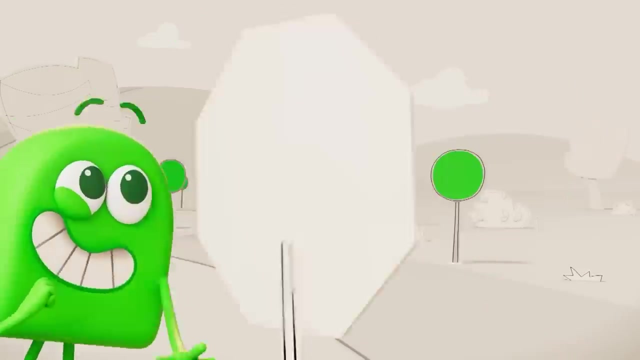 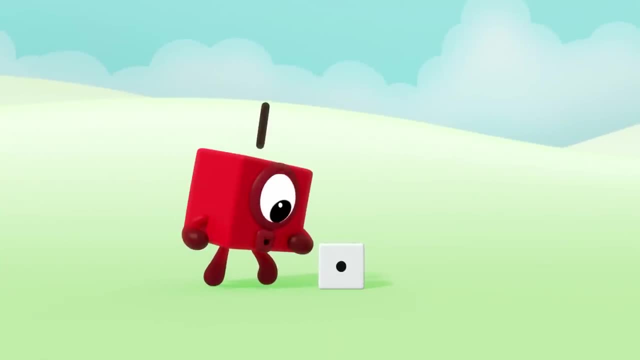 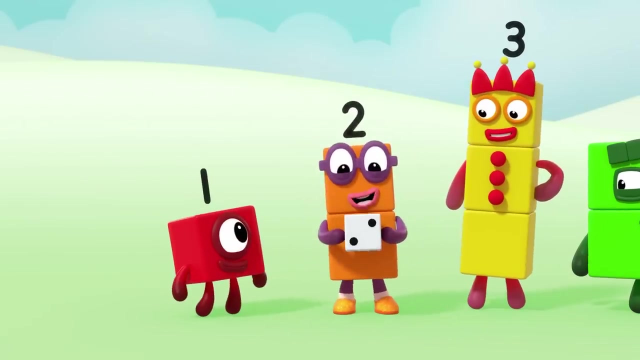 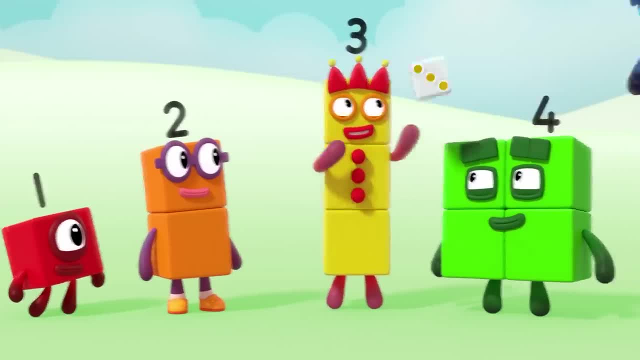 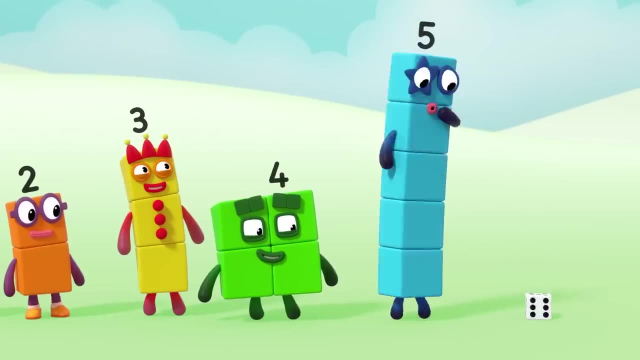 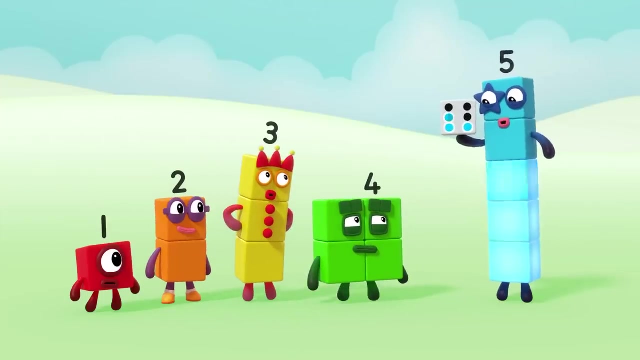 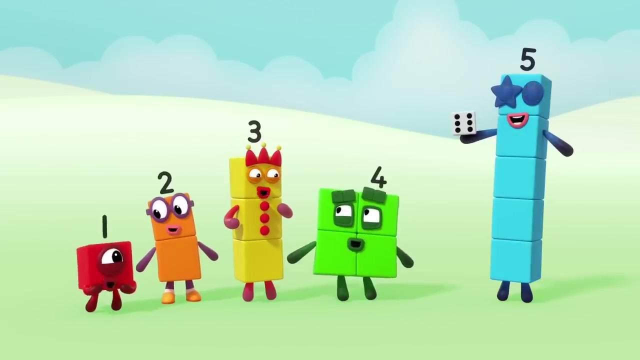 Let me see Three dots, Four dots In a square, Five dots- Oops, How many dots is that? One, two, three, four, five and one more, One more than five. You know what this means, Ready. 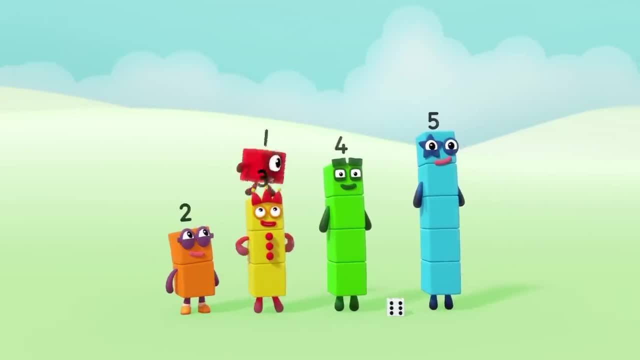 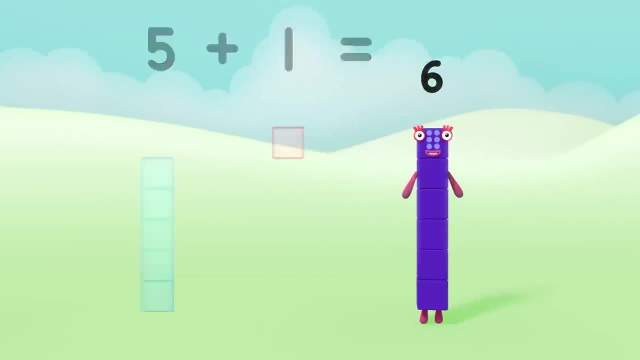 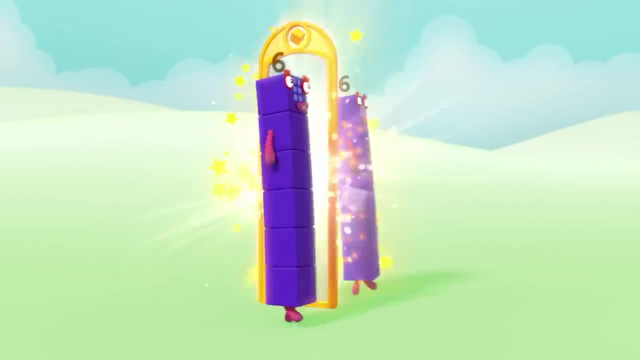 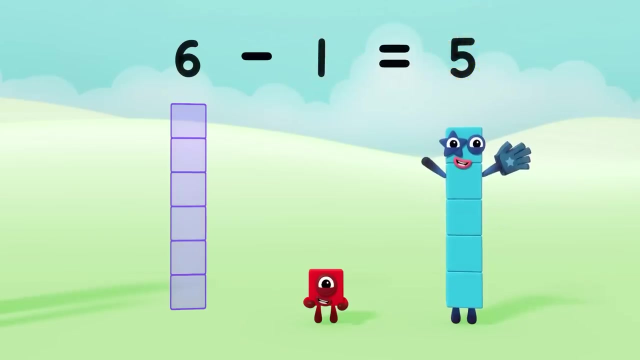 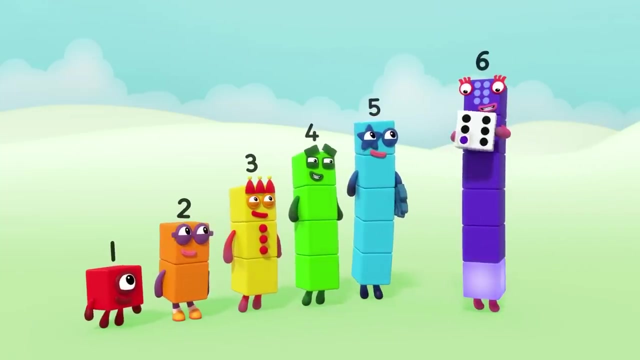 Ready. Five plus one equals six, And and six Time for some tricks. Six minus one equals five. Hey, One, two, three, four, five, six, six spots, just like me. What is it? This little block is full of tricks. It's got six faces, one to six. 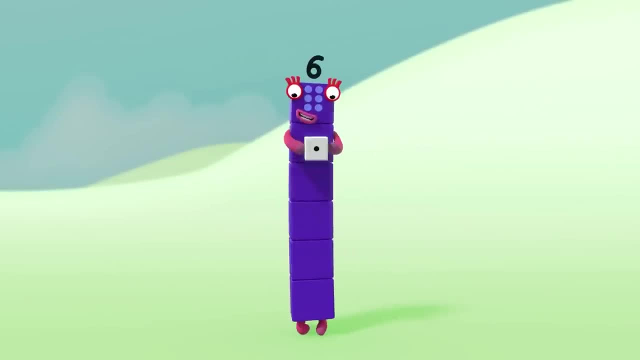 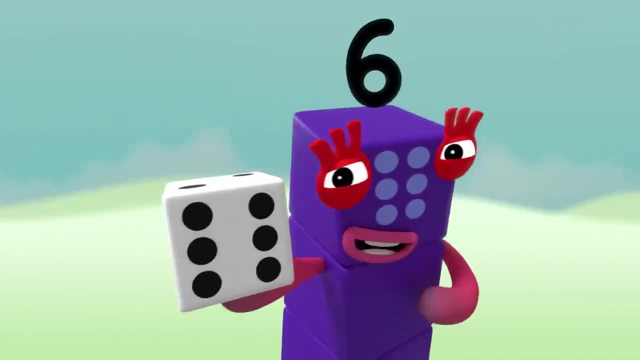 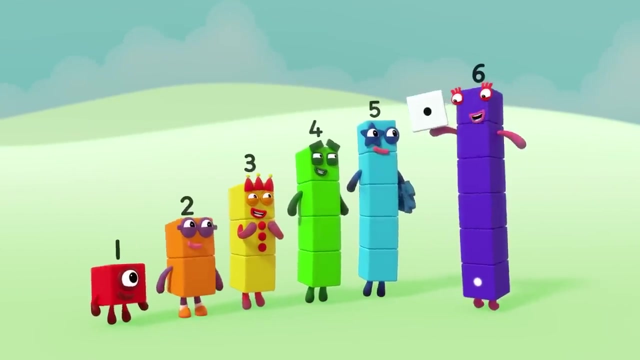 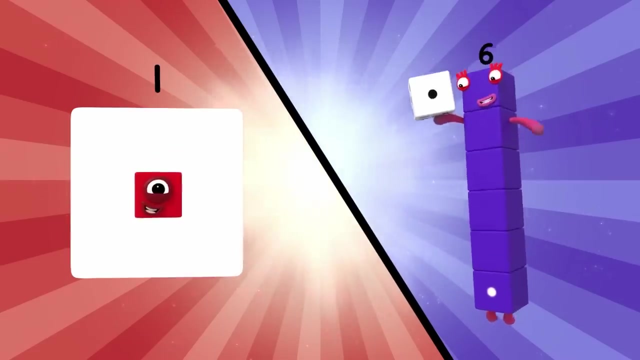 It's called a die. it's called a dice, Dice or die. both names are nice. What's it for? Let me explain. Want to know more? Let's play again. And this game goes like this: When you see a number, make the shape. 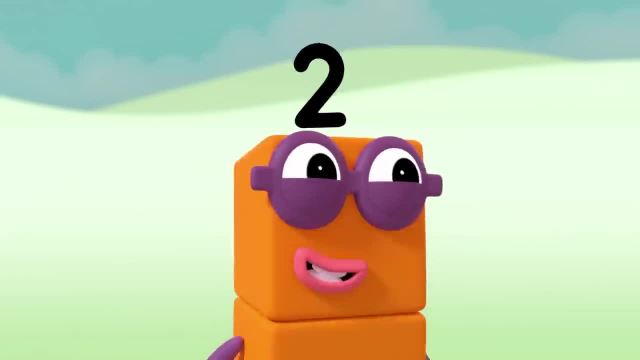 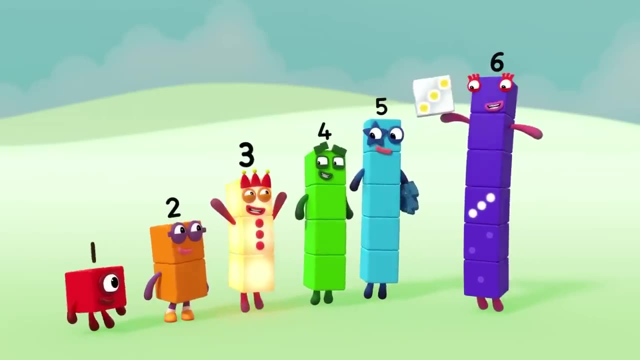 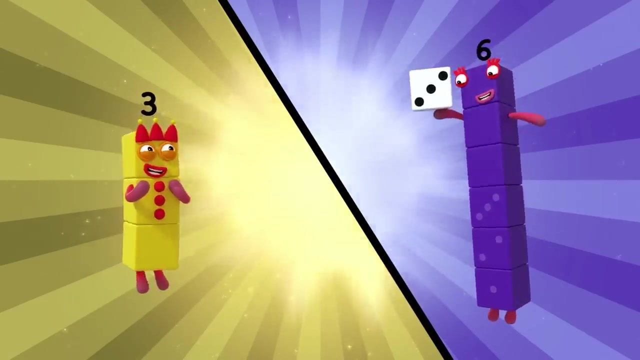 One. one spot on the dice. Make the shape One. One, two. two spots on the dice. Make the shape Two: One, two, three. Three spots on the dice: Make the shape three: One, two, three, four. 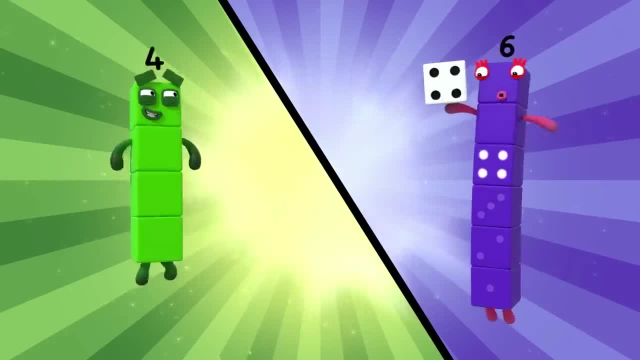 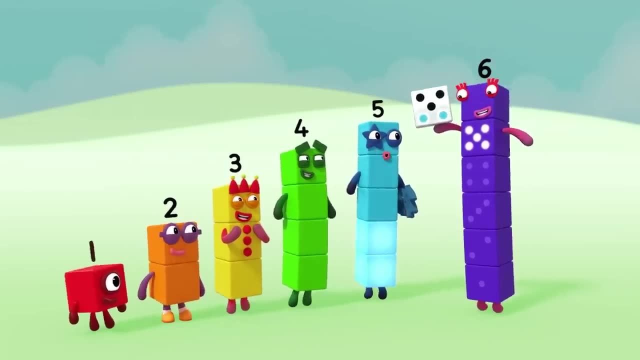 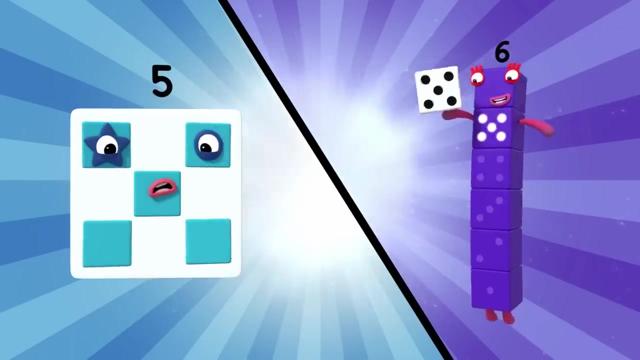 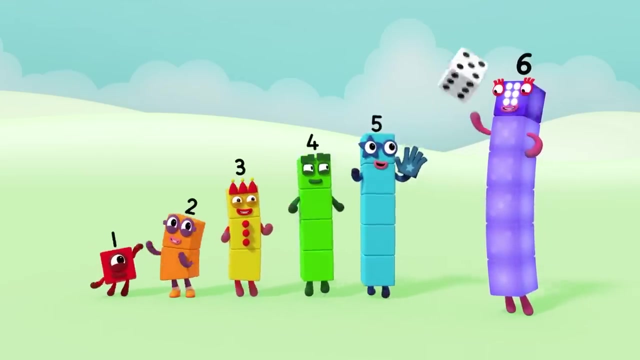 Four spots on the dice: Make the shape four. It's a square One, two, three, four, five, Five spots on the dice: Make the shape five. One, two, three, four, five, six, Six spots on the dice: Make the shape six. 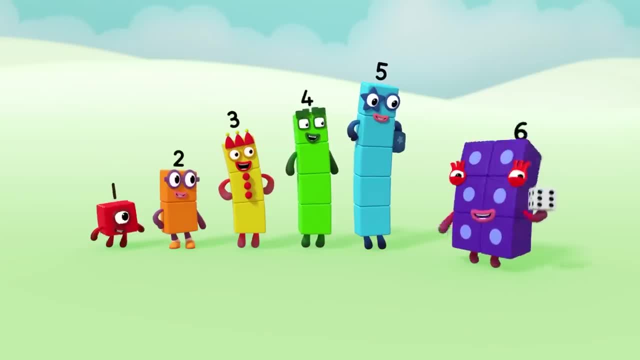 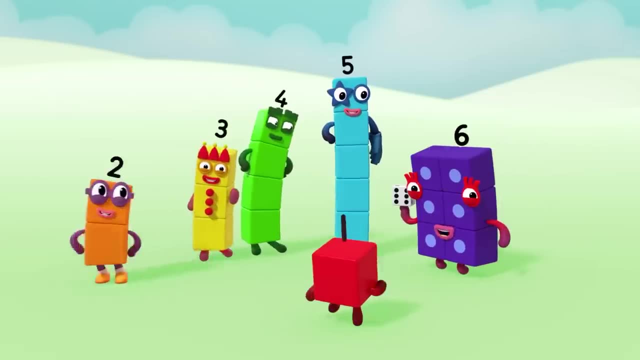 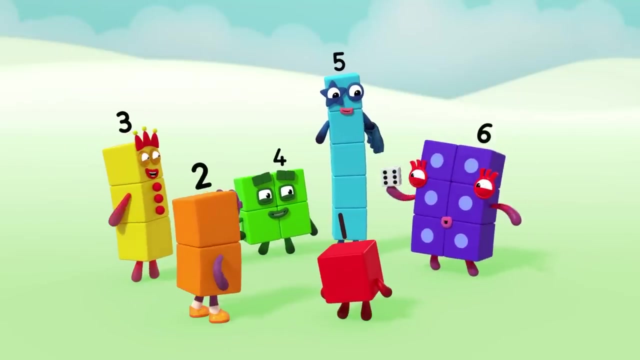 I'm number six and I've got game. When you hear my name, you'll be glad you came. So take a chance. pick my advice: Do a little dance and see what happens. Roll the dice. I'm number six. I'm in the mix. Good times are my go. that's how I roll. 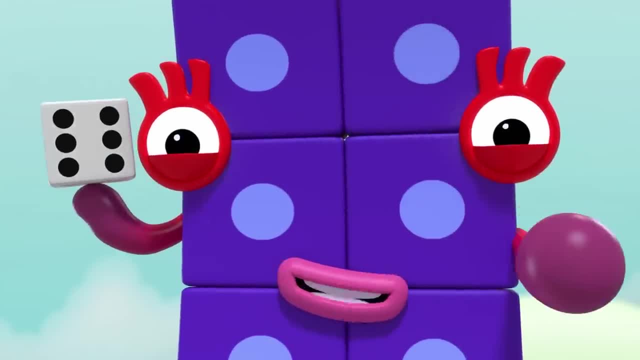 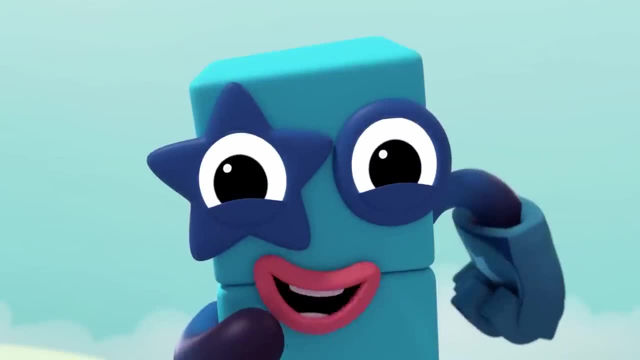 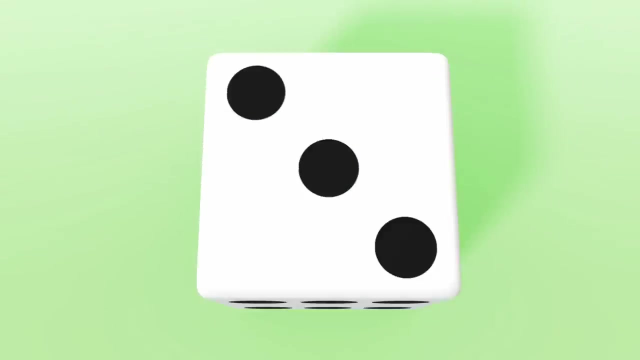 New game. If you see your number, it's your turn to dance. Let's roll Five hand jive: One, two, three, four, five. One, two, three, four, five, Three. look at me: One, two, three. 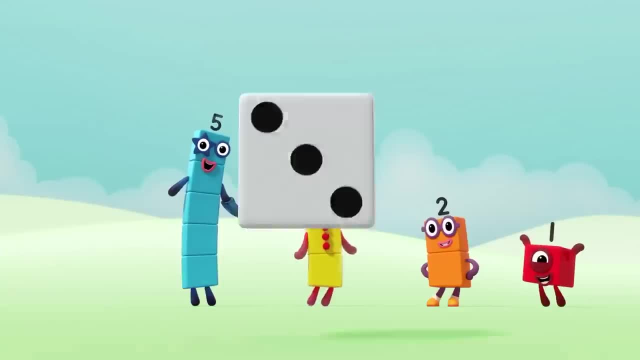 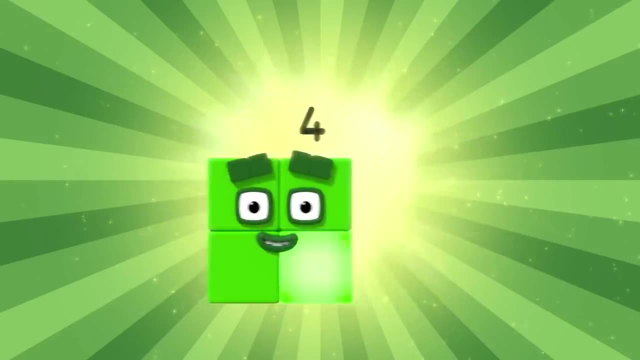 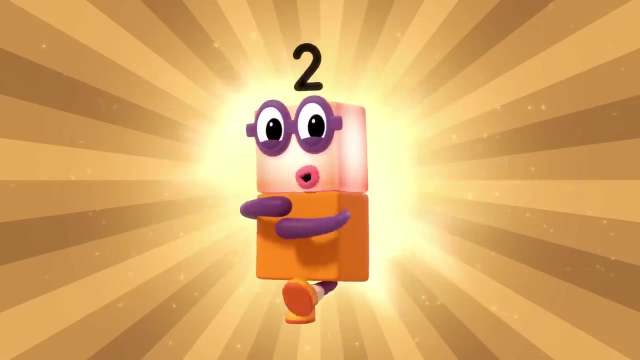 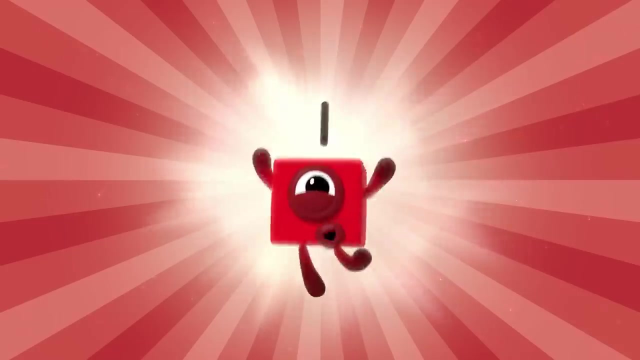 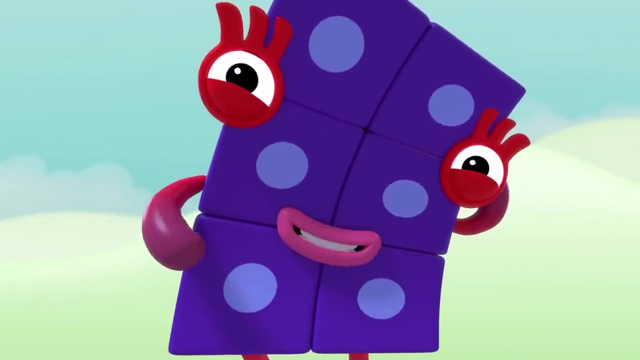 One, two, three, Four, Not sure. Oh, square dance. One, two, three, four, Two Time to use my dancing shoes. One, two, one, two, one, two, One. this is fun. One, one, one, one. Six Is in the mix. 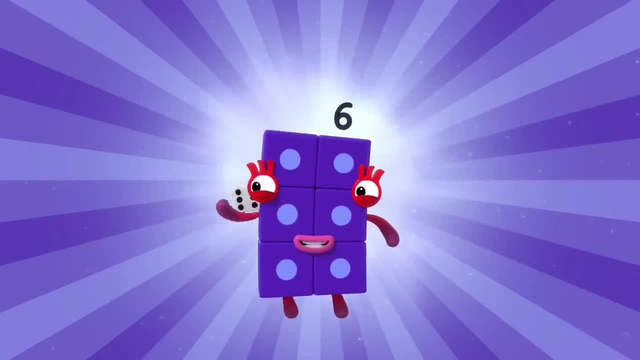 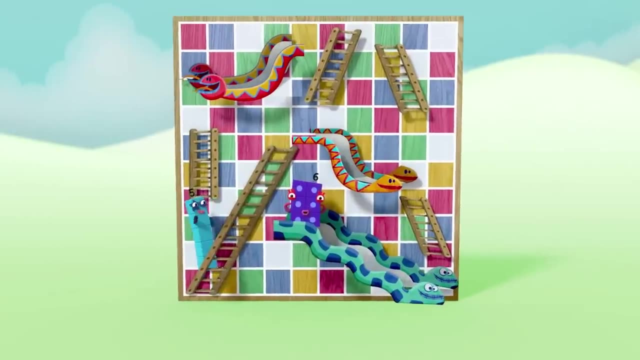 I'm number six and I've got game. When you hear my name, you'll be glad you came. There are lots of games You can play. you can play a new game every single day. Have a little go at snakes and ladders Up the steps and down the adders. 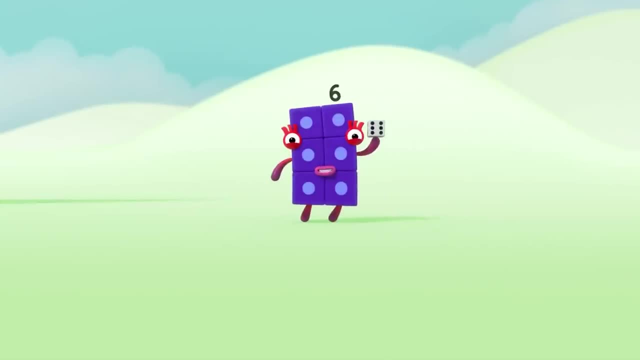 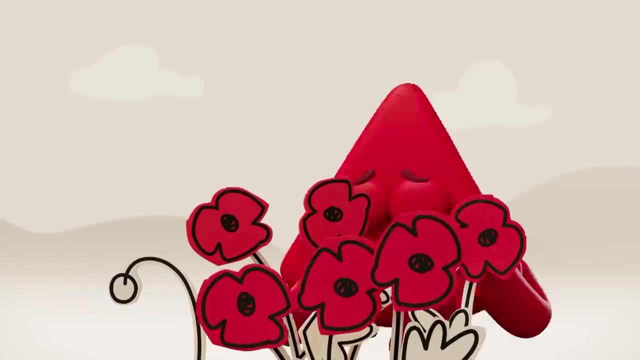 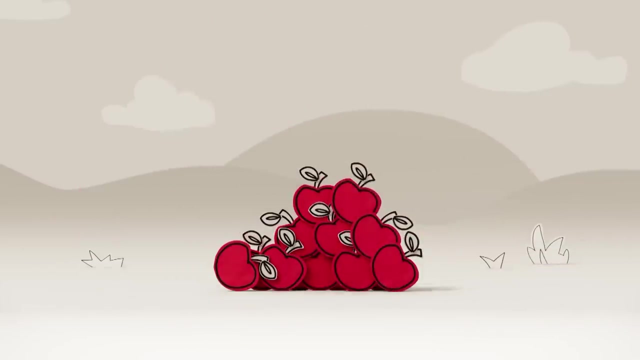 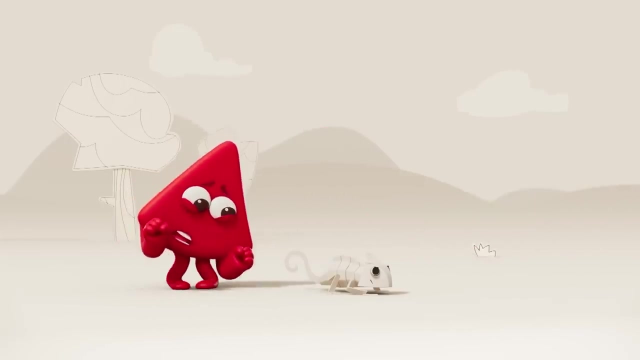 I'm number six. I'm in the mix. Good times are my go. that's how I roll: Red, I'm red and I'm ready to roll Red, red, red, red, red, Whoa. What are you? I love it. 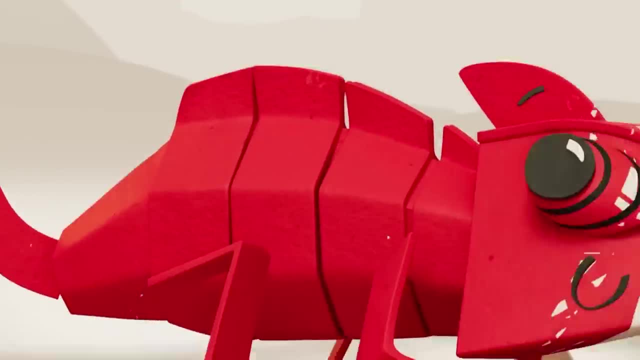 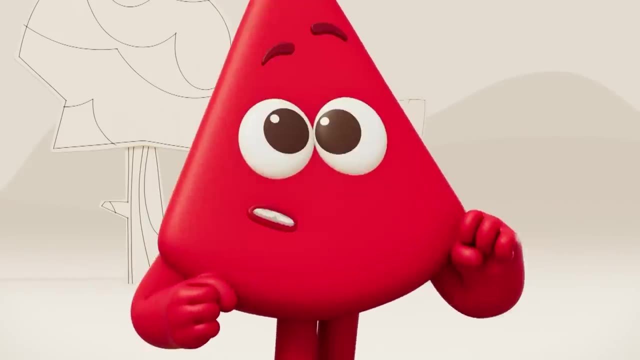 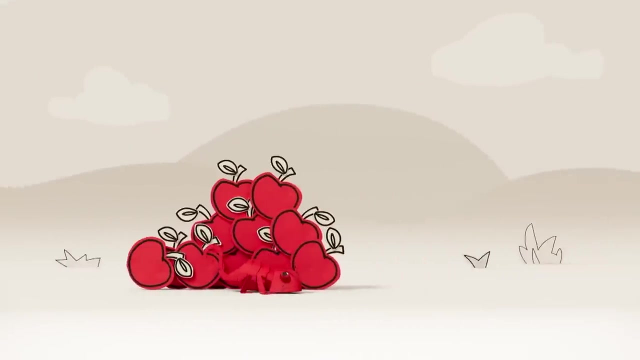 But you would be more exciting if you were red. Awesome, Oh, I'm going to call you Redora. Hey, Come back, Redora, I want to show you all the red things I've made. Oh, Redora, Redora. 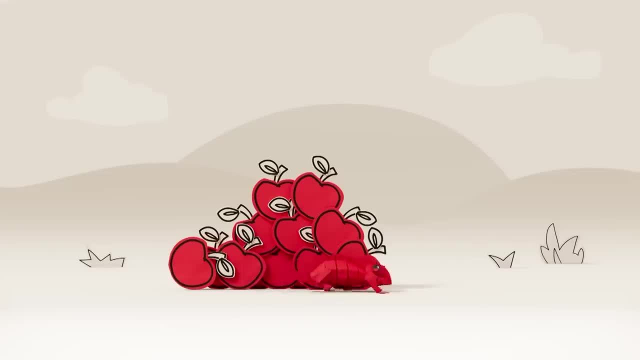 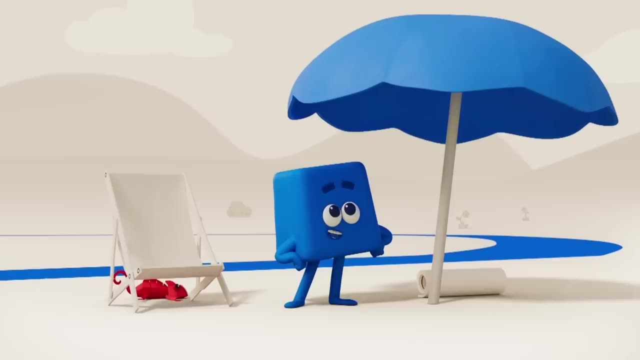 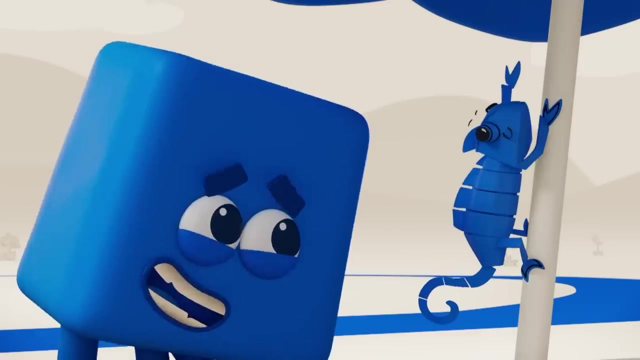 Oh, where'd you go, Redora? Blue, Cool Blue, Perfect for a relaxing day. Huh Oh hello. I don't remember colouring you, but blue suits you. I'm going to call you Bluesy. 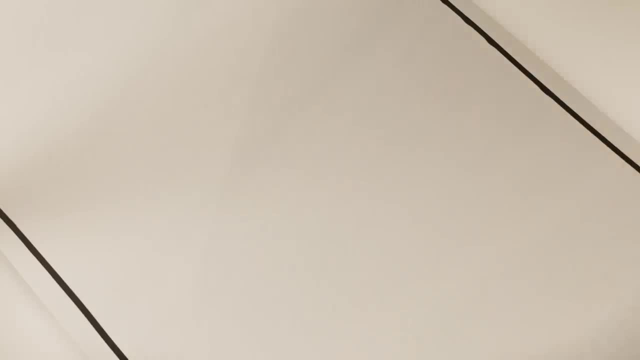 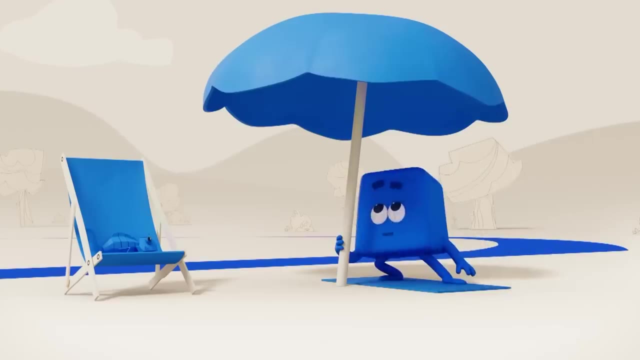 Wait here, Let me get you something to sit on. Blue, Here you go, Bluesy You can sit on Huh, Bluesy, Where'd you go, Bluesy? Where's Bluesy gone Here? Bluesy, Bluesy, Bluesy. 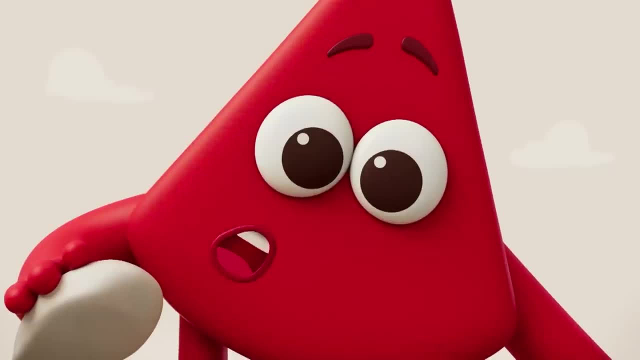 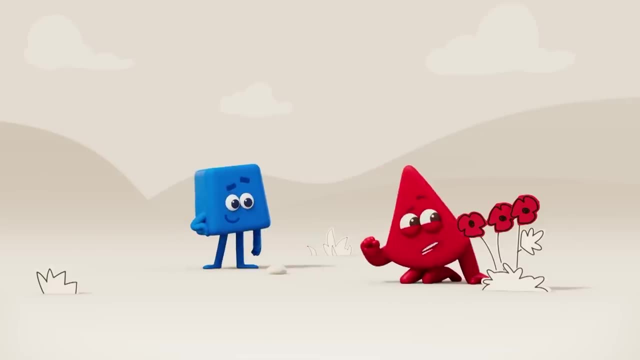 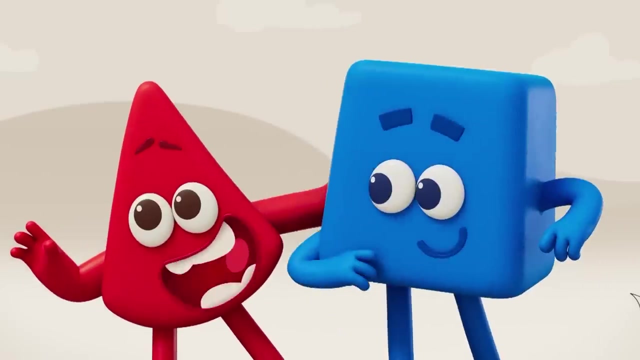 Bluesy Redora, Where are you? Oh, hey, Blue, Have you seen Redora, Redora, Who's that? Only the cutest, reddest little thing ever. She's my new friend. Hey, I'm looking for my new friend too. 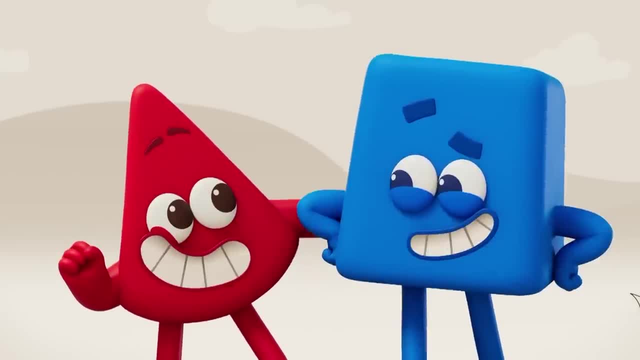 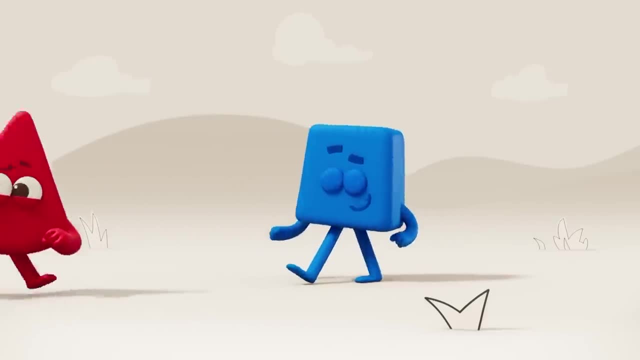 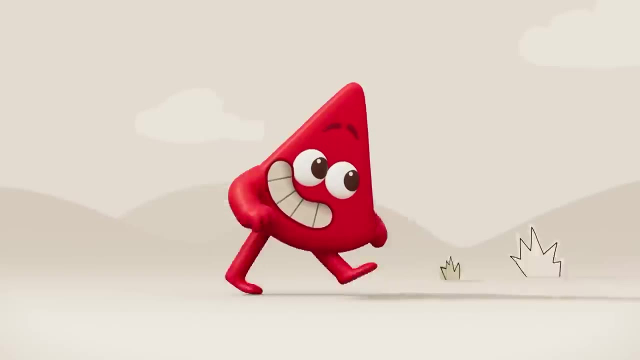 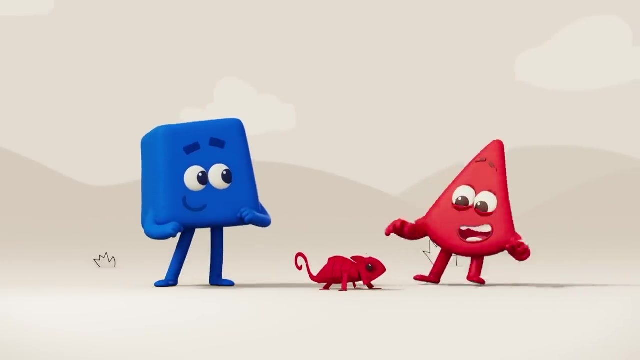 She's called Bluesy, You know, because she's blue. Since we're both looking, shall we look together? Great idea: Follow me Maybe this way. Oh, Redora, See, Isn't she awesome? I call her Redora because she's blue. 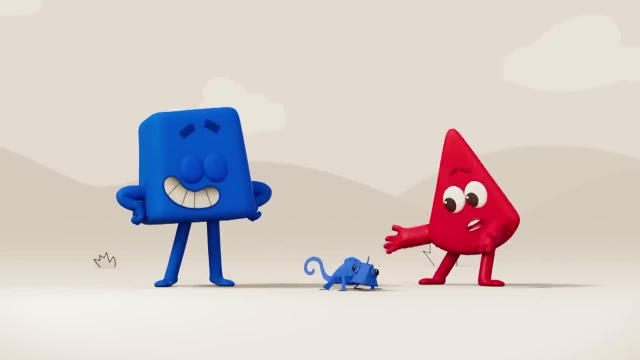 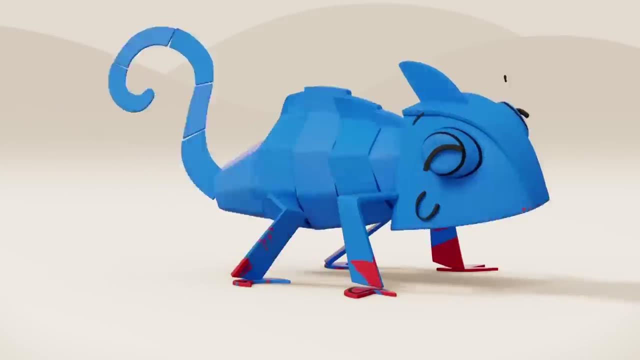 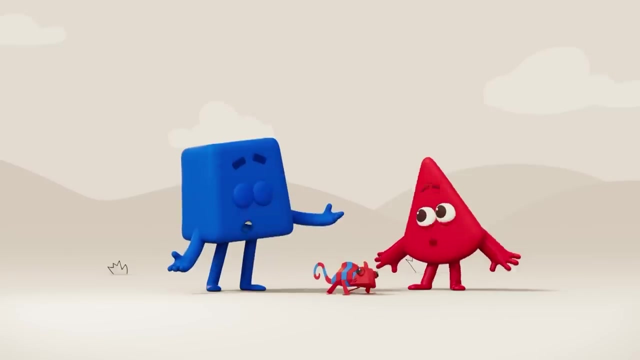 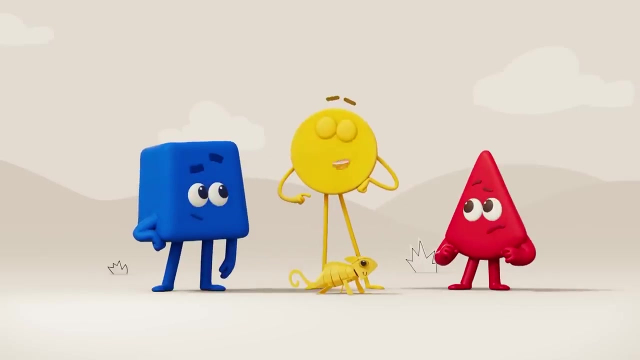 Hey, Bluesy, There you are. But where did Redora go? Now she's red. Huh, Back to blue. Blue, Wow, Red and blue, Cool, Huh, Yellow knee. There you are. I've been looking all over for you. 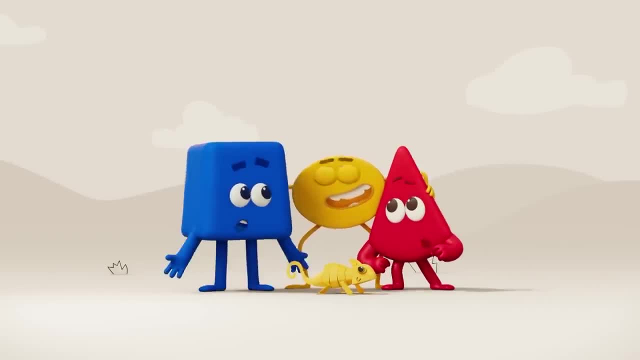 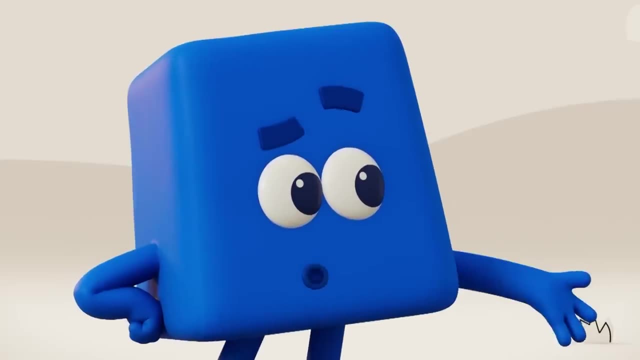 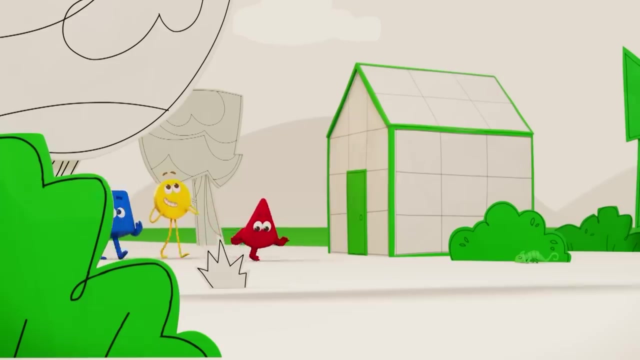 Thanks for finding my new friend, Your new friend. What's going on? Why does Redora keep changing colour? Yeah, one minute she's blue, then Hey, She's gone. Hey, Bluesy, Bluesy, Bluesy. 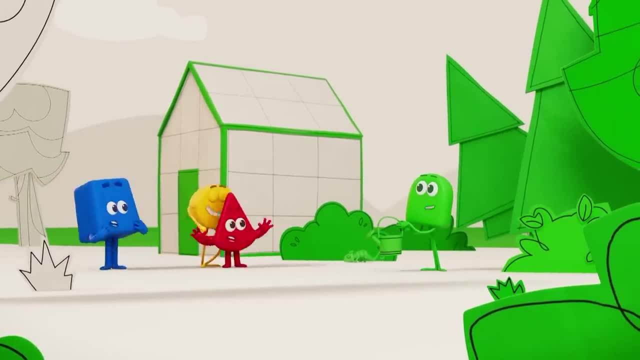 Where did she go? Where did who go? Wowzers, I didn't see you there. Sorry, Didn't mean to scare you. Who are you looking for? Our new animal friend, Oh, have you seen her? An animal, Oh, I love animals. 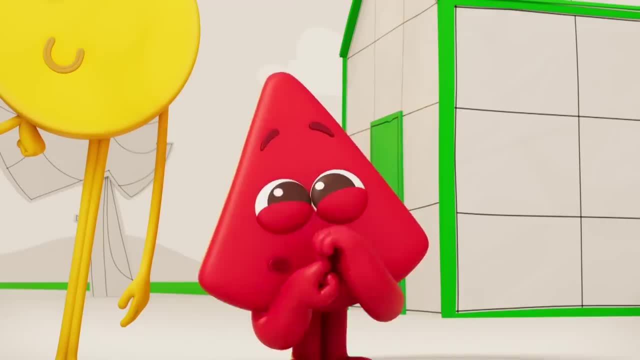 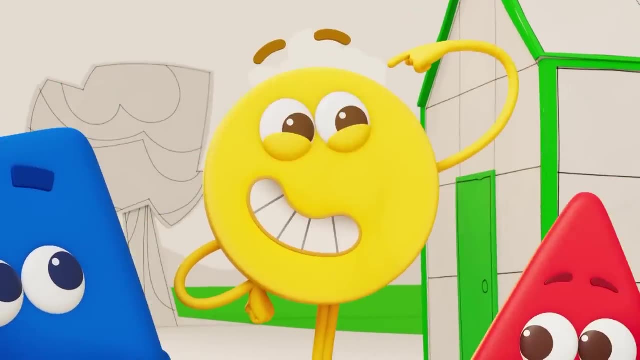 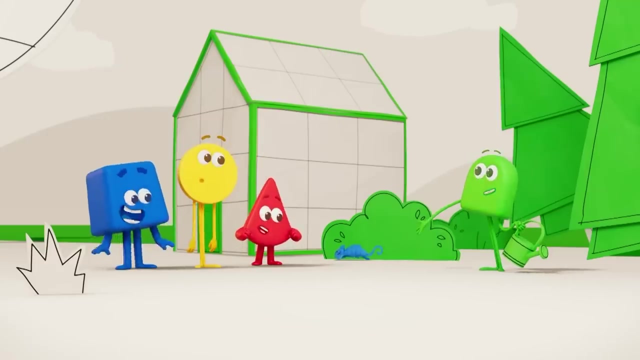 What does she look like? Well, she's small, and cute, and sometimes she's red, Yeah, but sometimes she's blue And other times she's yellow. Small, cute and changes colour. Do you mean this little one Bluesy? You found Bluesy. 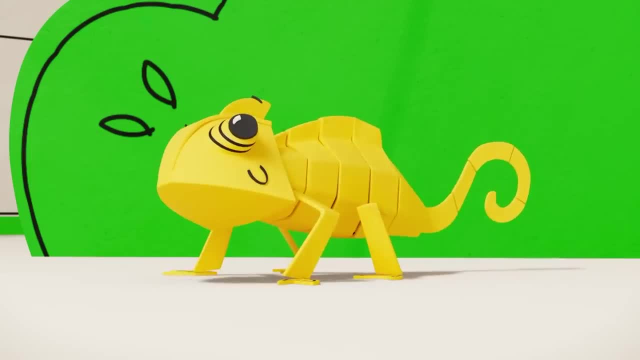 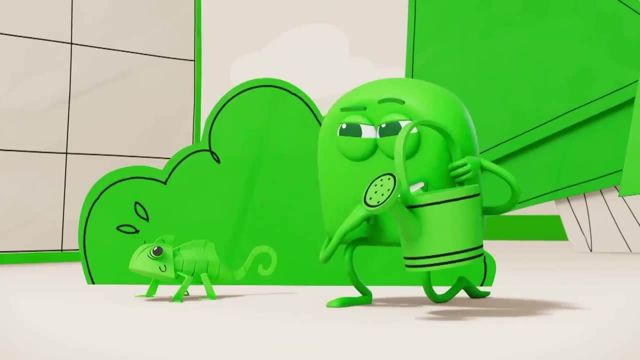 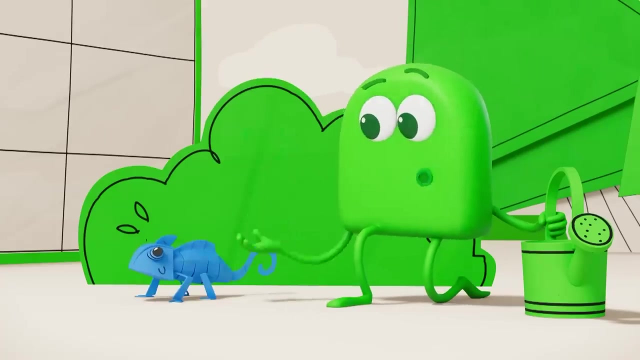 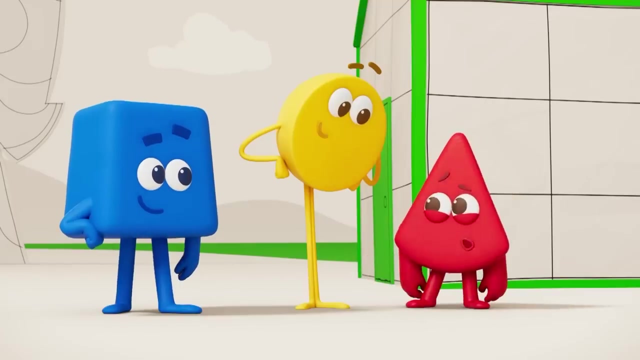 See, She did it again. She changed colour. Yep, that's what she does. Sometimes it's to hide herself, And sometimes it's to stand out, And sometimes it's to show how she feels Blue means she's relaxed. Well, if she always changes colour, I guess I can't call her Redora anymore. 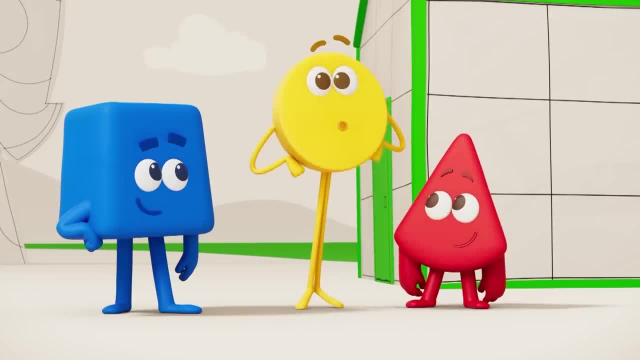 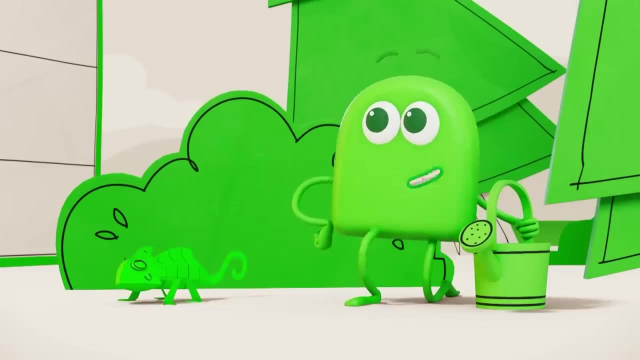 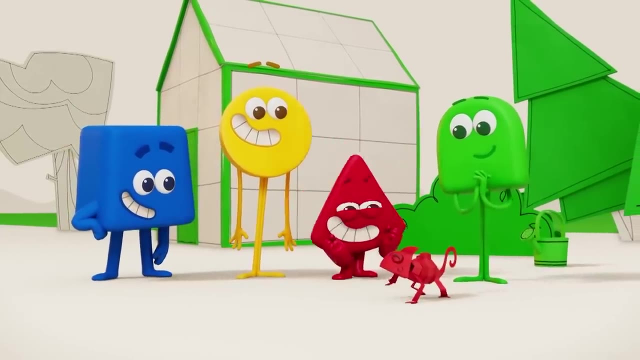 Or Bluesy either. Hmm, Oh, how about Redora Bluesy, Yelleny Green, I think. she prefers to be called Chameleon. Then that's what we'll call her: Red Chameleon, Yellow Chameleon, Blue Chameleon. 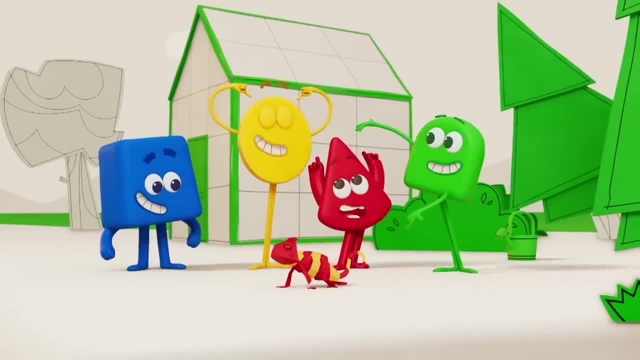 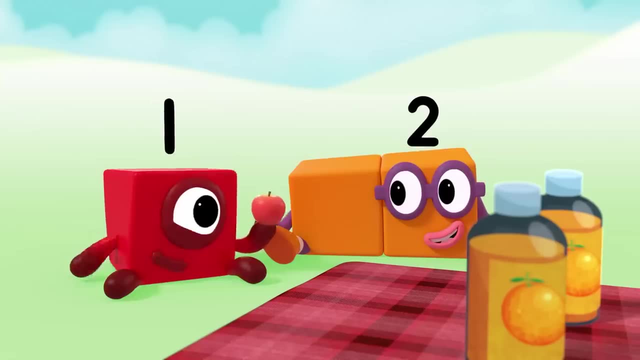 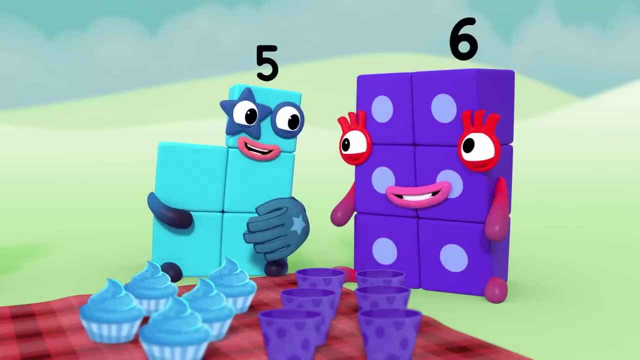 Green Chameleon, Red and Yellow Chameleon, Hooray, Br. eventually Nice picnic. I can't wait. It looks so yummy. That's a 5-star picnic. Let's get stuck in, shall we? Oh, The sun's gone in. 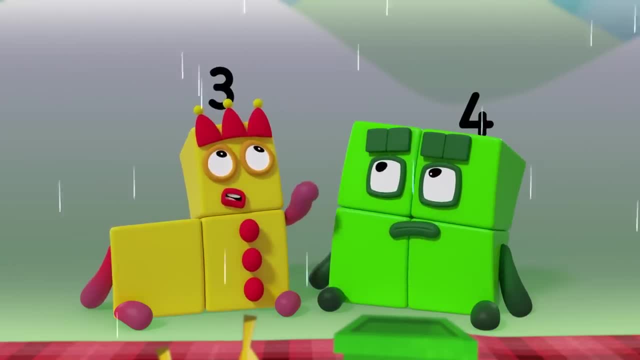 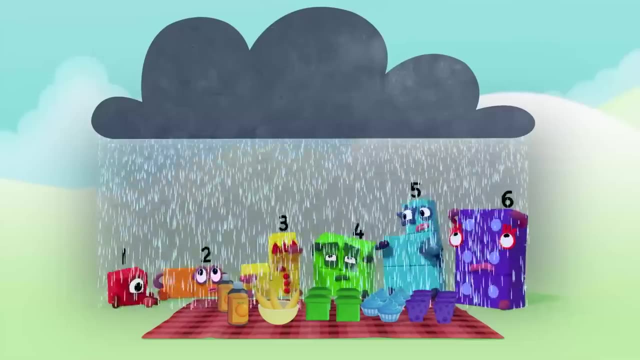 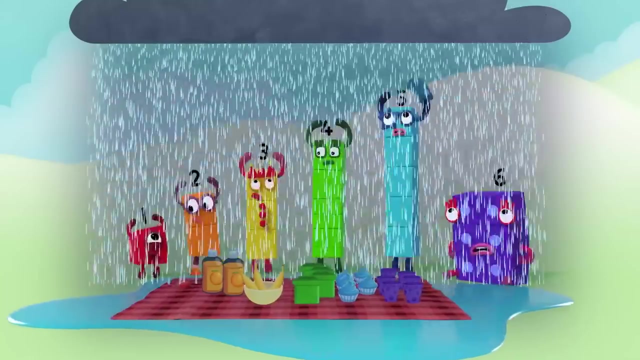 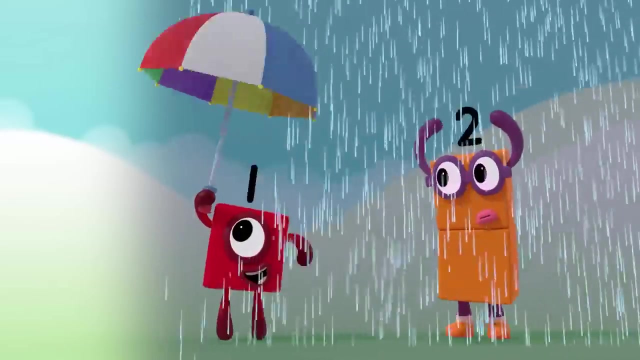 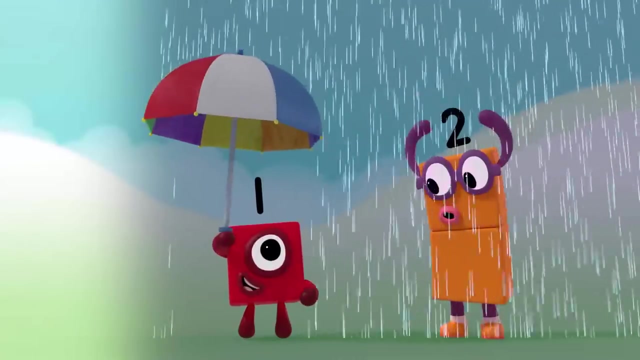 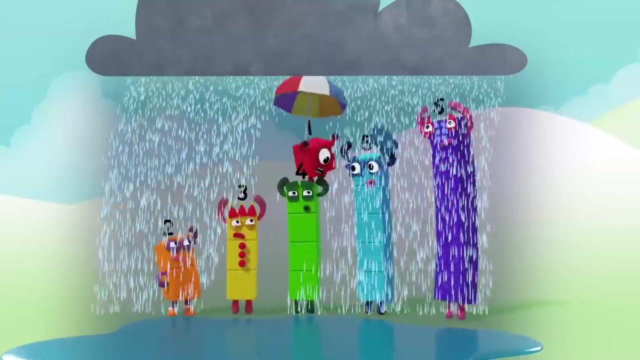 That's unlucky. Starting to rain? That's unlucky. It's raining a lot now, That's unlucky. Anyone got an umbrella? I got one, Only one. That's unlucky. I can share it. Six plus one. Six plus one. 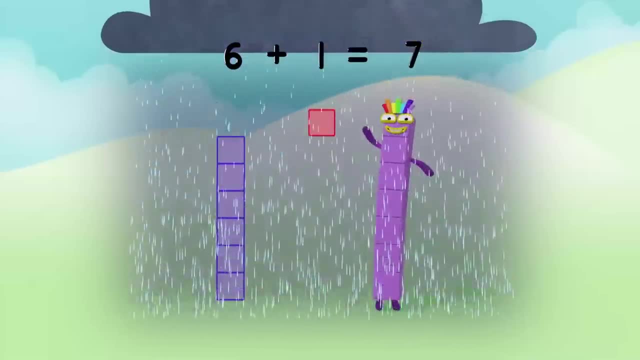 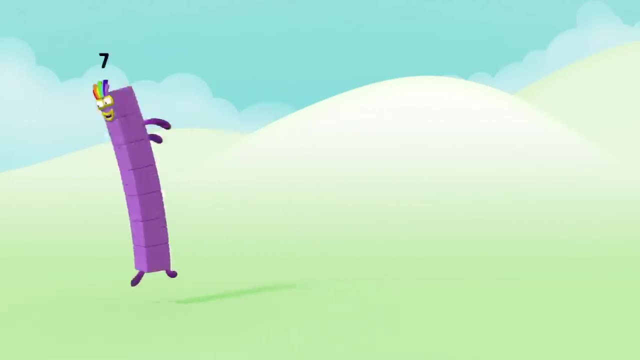 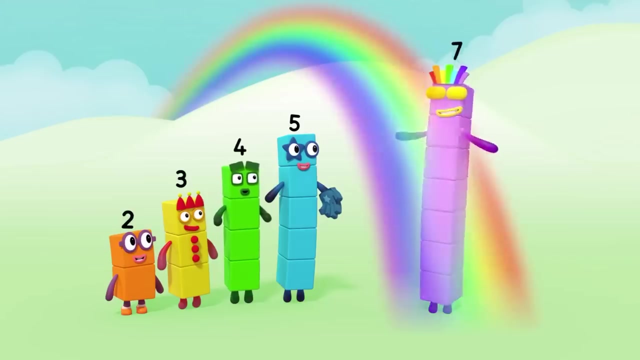 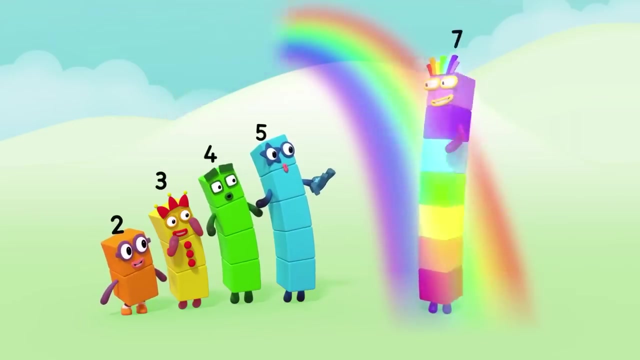 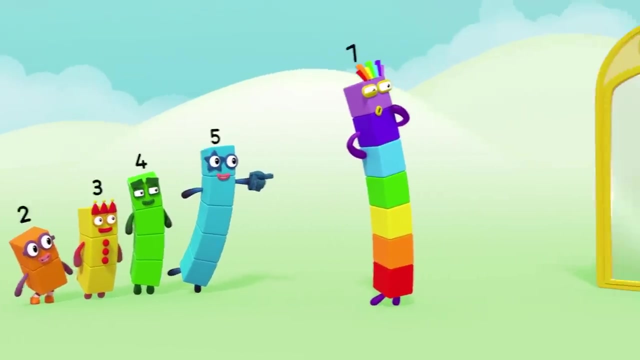 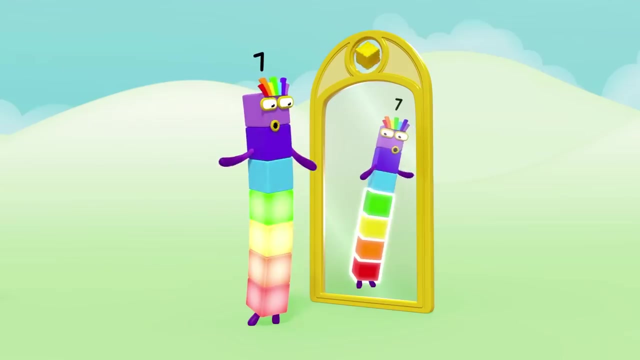 Equals seven, I am seven, Am I in heaven? You're in number land, Lucky me A rainbow. Wow, What happened? Look, Oh, a mirror. That's lucky One, two, three, four, five, six. 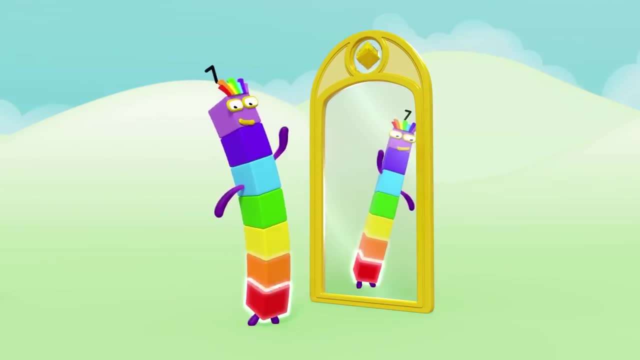 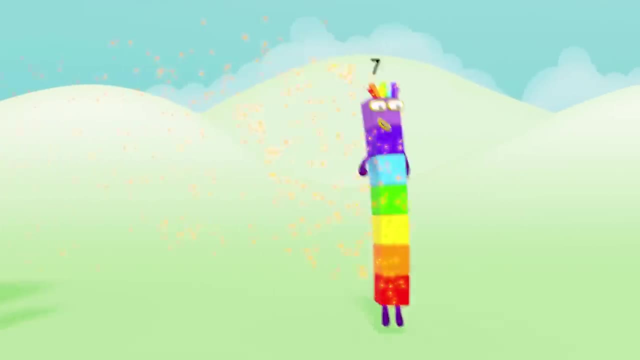 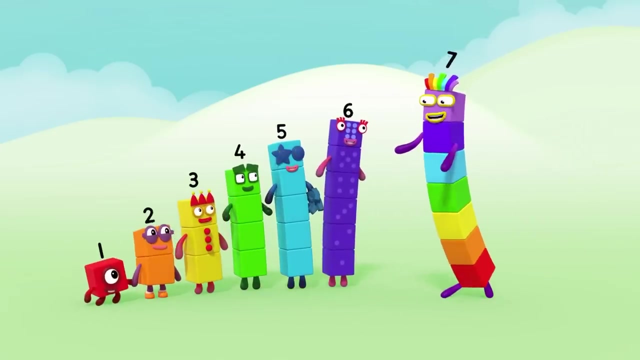 seven, Seven colours, Like all the colours of the rainbow. Now, isn't that a stroke of luck. Luckily, I know just what to do now. Seven minus one equals six. What All you lovely blocks are, my friends? Mm-hmm. 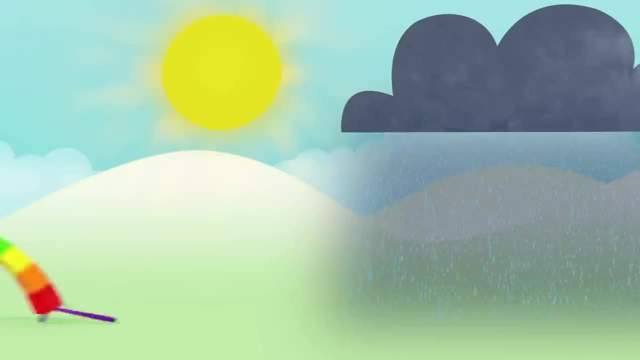 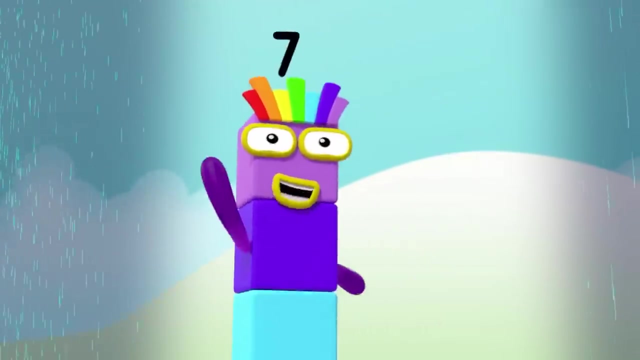 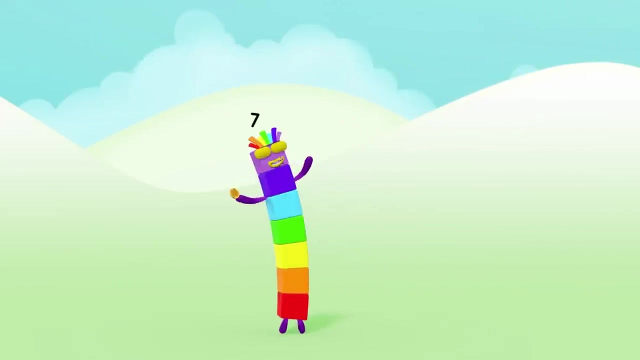 I'm the luckiest number block in the world. I'm lucky number seven. I'm in a happy place, The sun is always shining and there's always a smile upon my face. I see a penny and I pick it up, and all day long I have good luck. 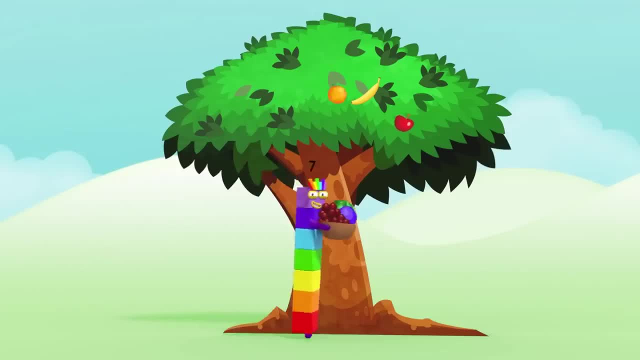 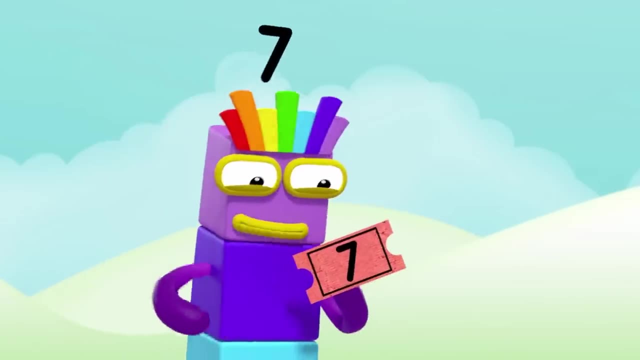 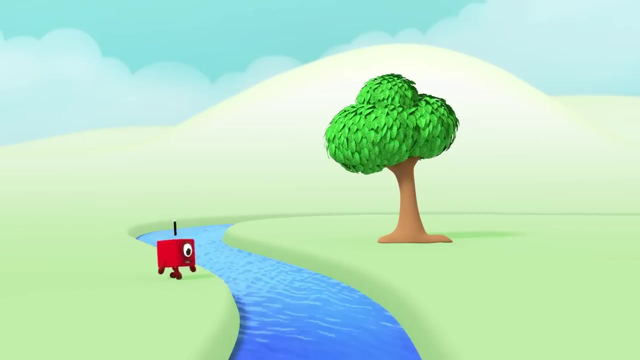 I'm lucky number seven And everything is falling into place. I'm lucky number seven And, as you might have guessed, I always win the raffle. With seven on your side, you're seven blessed In a pickle. you're in luck. 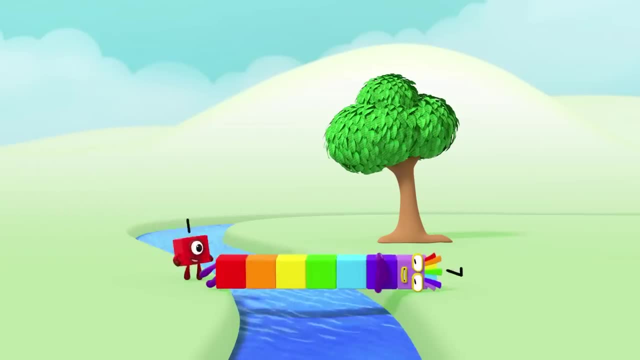 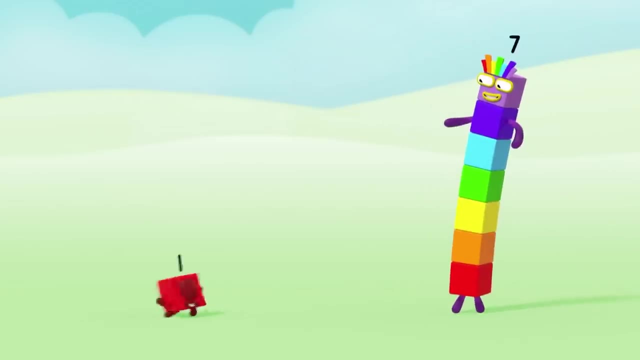 I'll help you out when you get stuck. And if you stick with seven, everything will work out for the best. Rainbow time Right. My first block is the same as you, Orange. My second block is the same as two Yellow. 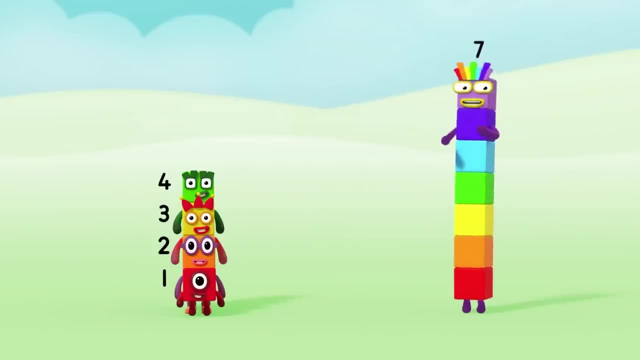 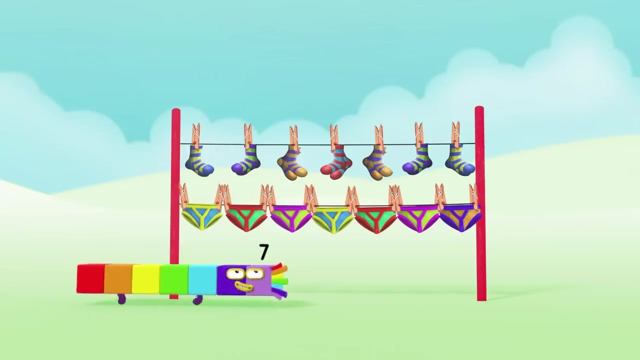 My third block is, just like number three, Green. My fourth is green, as you can see: Blue for five, Indigo for six, Violet is for seven. Oh, that's me, I've got seven rainbow-colored blocks. that makes me unique. 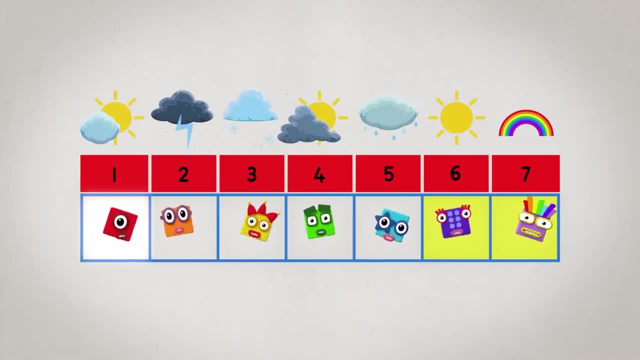 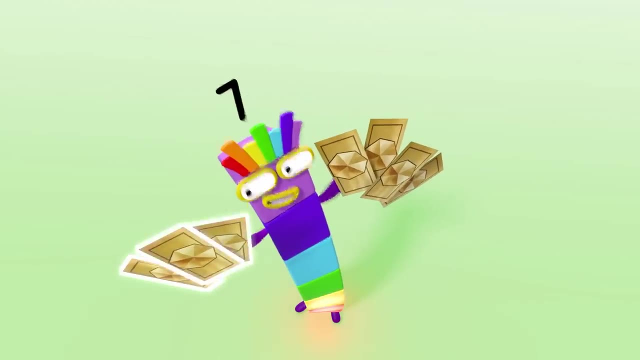 One for each day of the week: Monday, Tuesday, Wednesday, Thursday, Friday, Saturday, Sunday: One, two, three, four, five, six, seven. I've got seven golden tickets: One, two, three, four, five, six, seven. 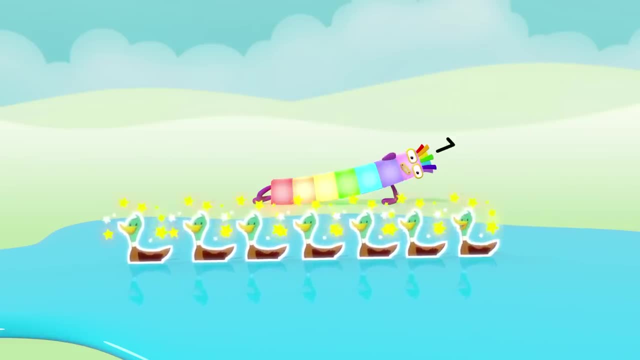 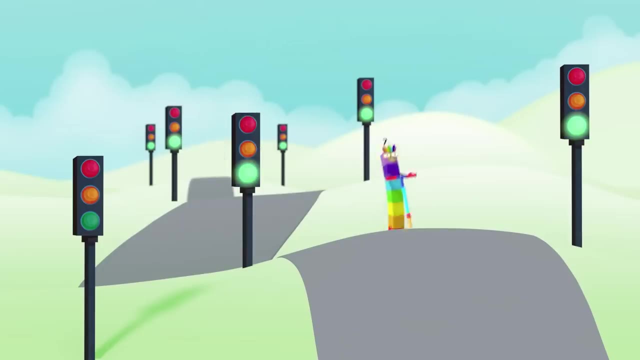 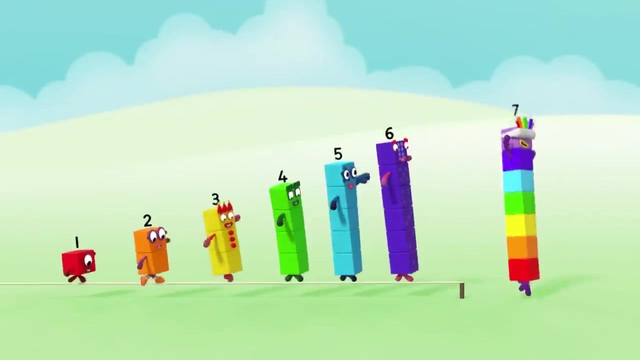 All my ducks are in a row: One, two, three, four, five, six, seven. Nothing's gonna stop me. All my traffic lights Go. I'm lucky number seven. I'd like to chance my arm In tricky situations. 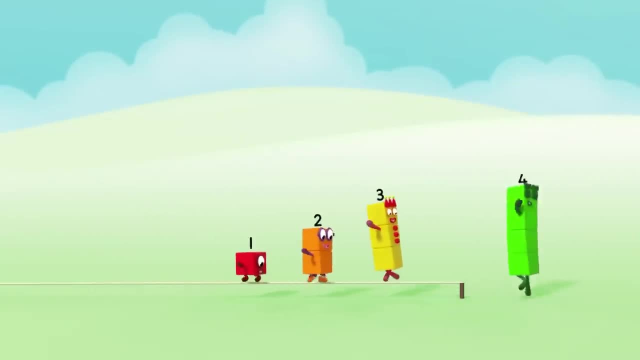 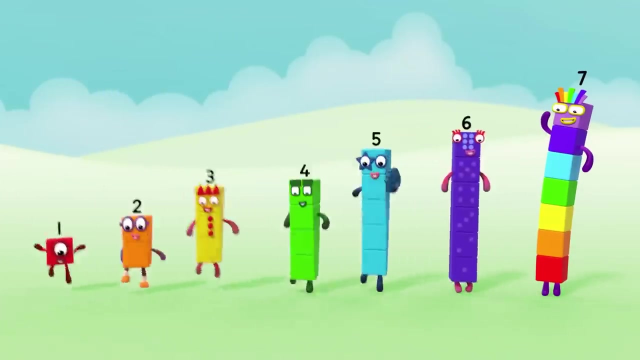 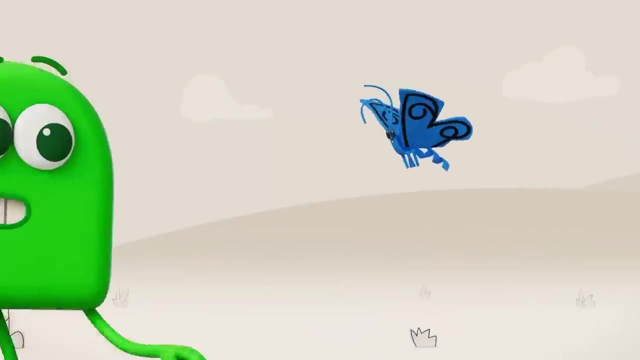 there's really no reason for alarm. I take problems in my strike. I've got fortune on my side. I'm lucky number seven. When you're with me, I'll be your lucky charm. What a nice day for a picnic, Naturally. 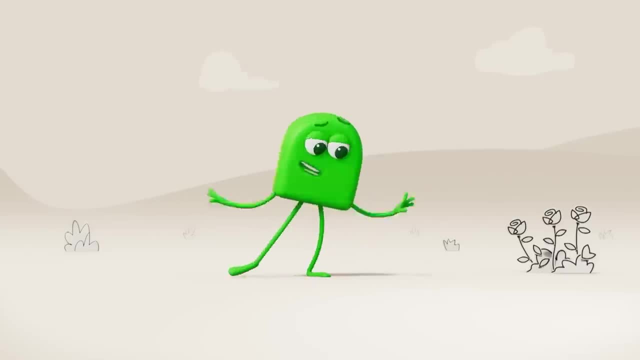 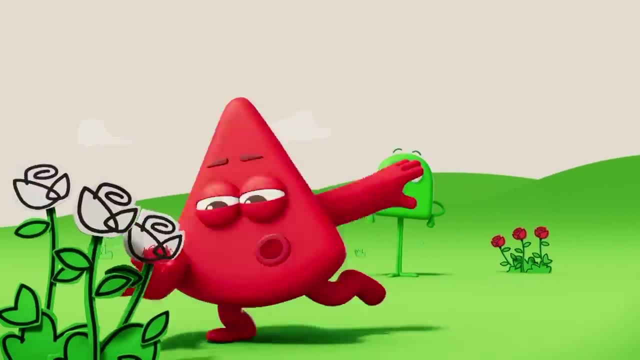 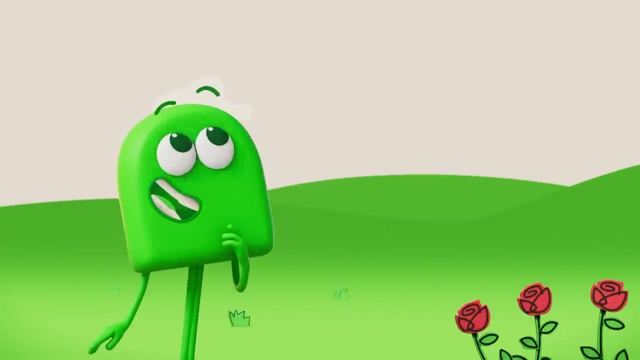 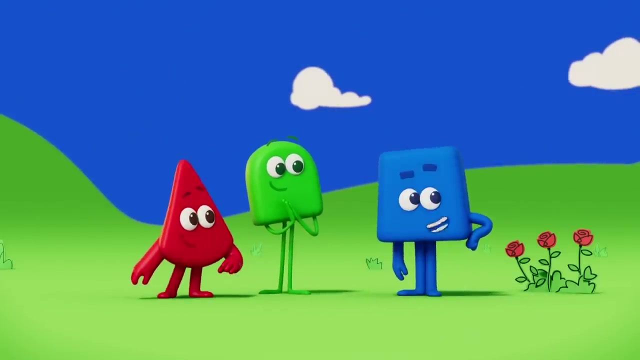 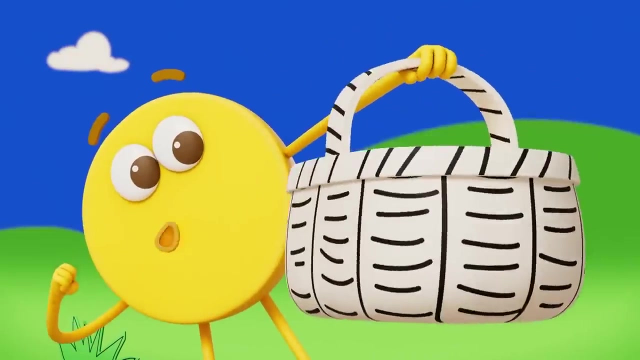 we can't have a picnic without some lovely green grass And some red flowers. No picnic would be complete without a bright blue sky- Blue Ha, Now where's yellow? I'm here, Look, everyone, I've got the most important thing of all. 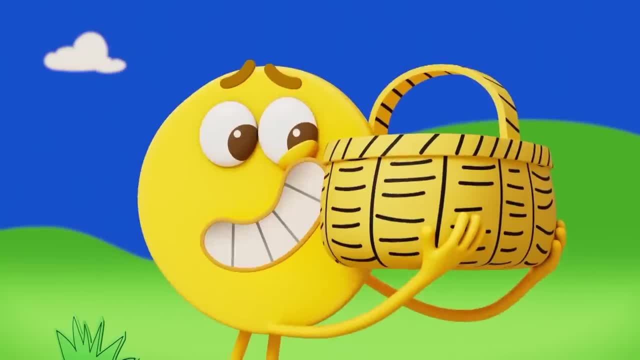 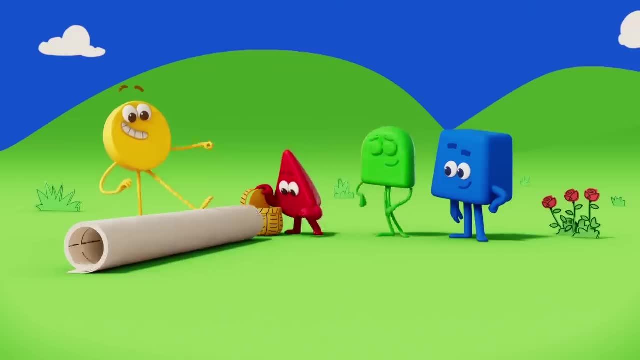 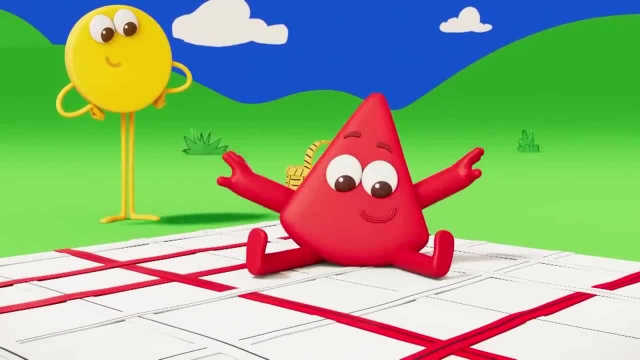 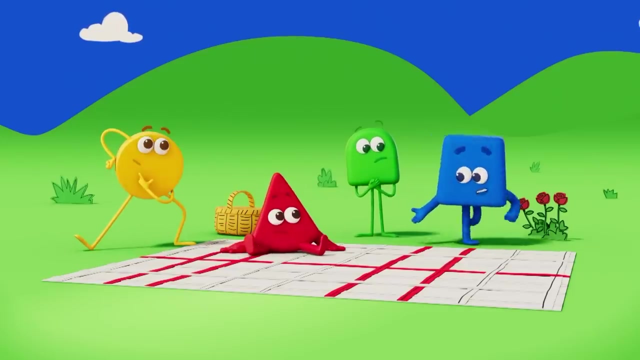 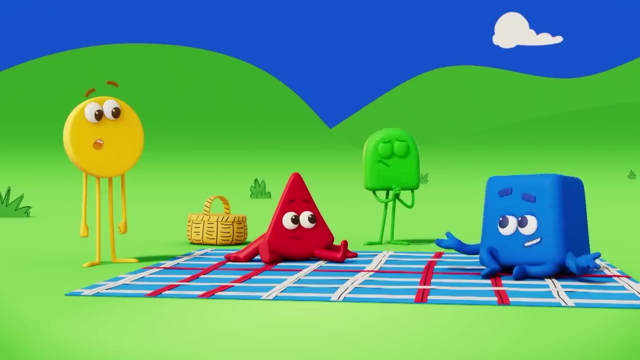 A yellow picnic basket. Exciting, Ooh, Huh, Cool. Oh, This picnic blanket should be red. Hey, Why is only some of it red? I think this blanket is supposed to be red and blue. Huh, Maybe we need some. 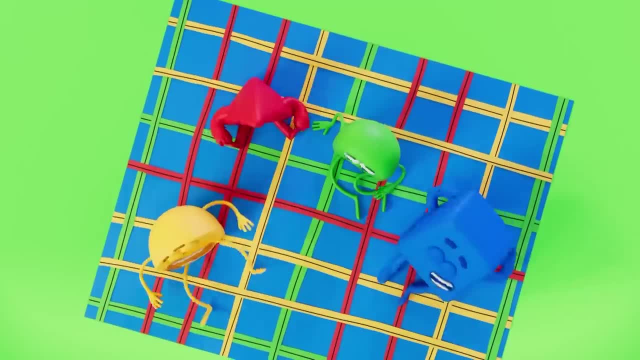 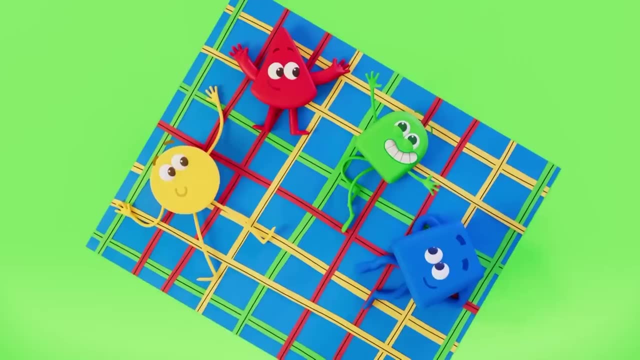 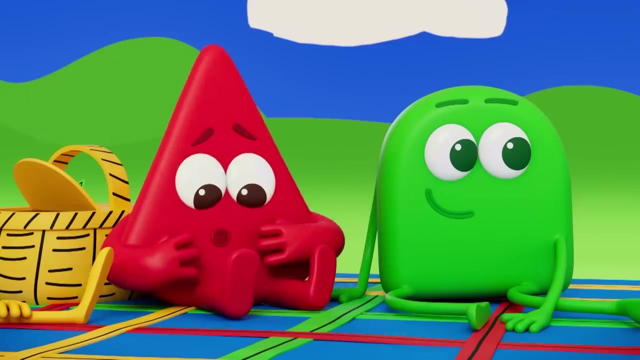 help. Green, Yellow, Hooray. The picnic blanket is a perfect pattern of red, yellow, green and blue, So some things can be lots of colours. Oh, All this colouring has made me super hungry. Can we start? 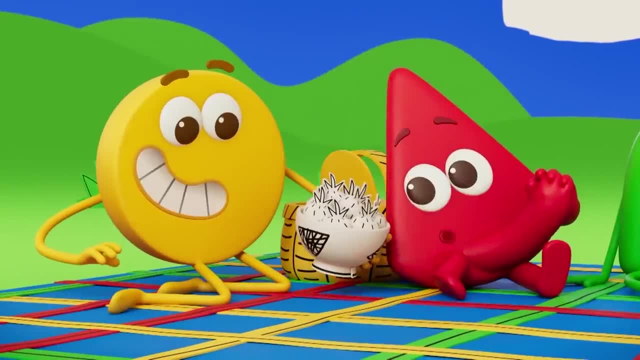 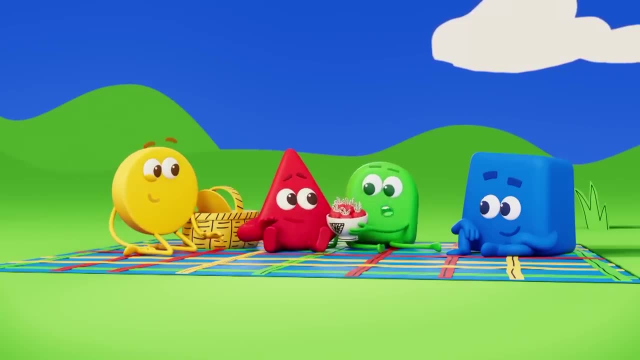 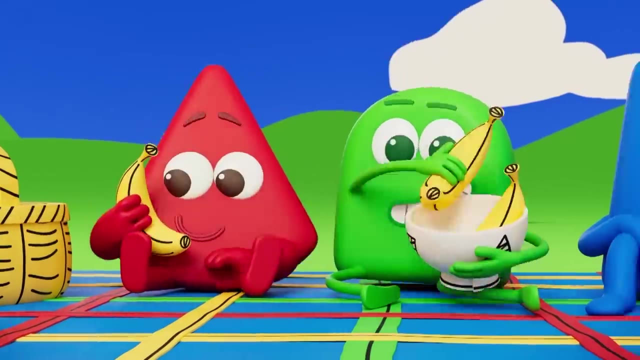 the picnic now, Please, Happily. Oh, Strawberries should be red. Yum, Naturally delicious. Oh, look, A lovely bunch of yellow bananas. Cool. What else have you got in there, Yellow? I've got some pears, Ooh. 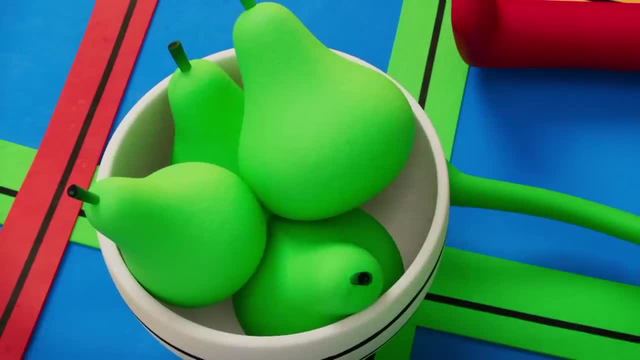 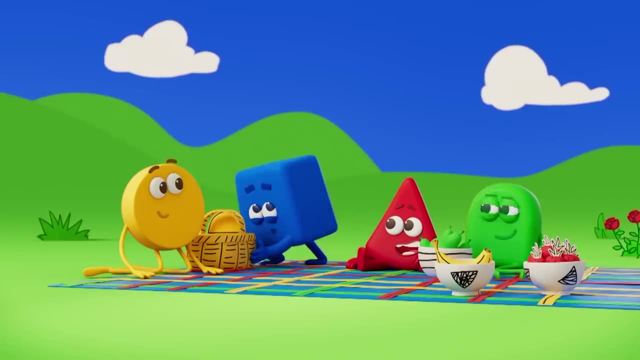 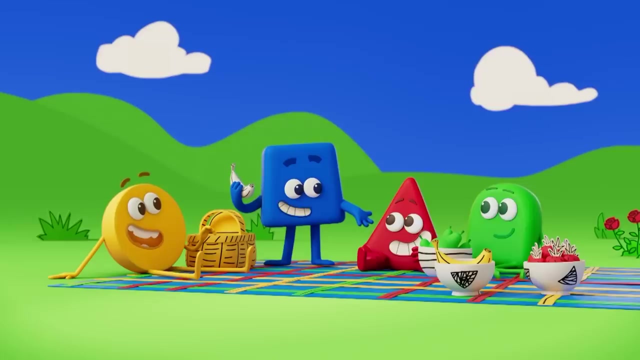 Leave those to me. Green pears, Hmm, I think it's time for some blue food. How about a blue banana? Bananas aren't blue, they're yellow. Shall we try it? What Colour it? a silly colour, Why not? It'll be funny. 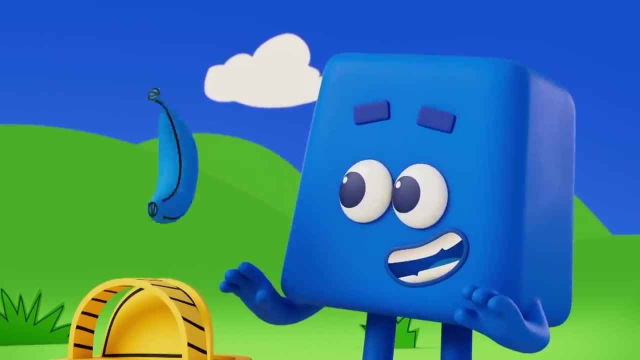 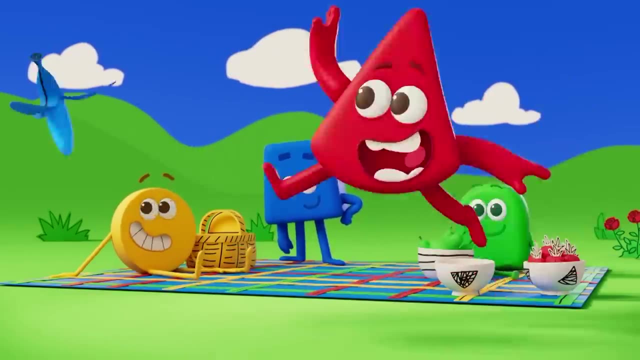 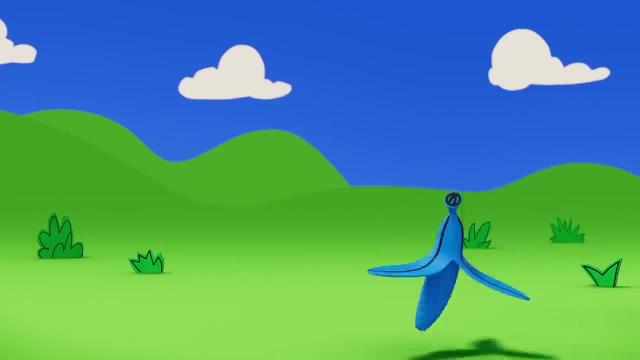 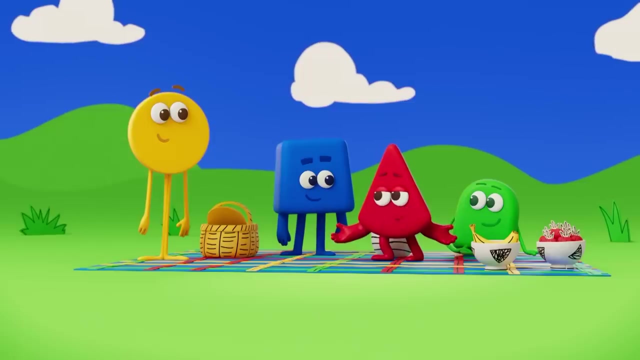 Blue, Blue bananas are very strange. Whoa Come here, blue banana, Look, look, Blue bananas are so funny. Phew, I think I'll stick with yellow bananas. At least they don't chase you. I think it's time for some more. 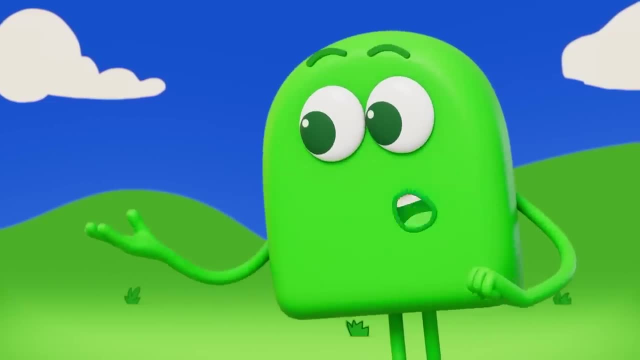 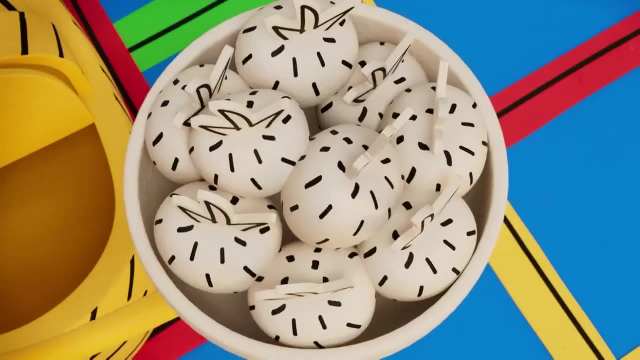 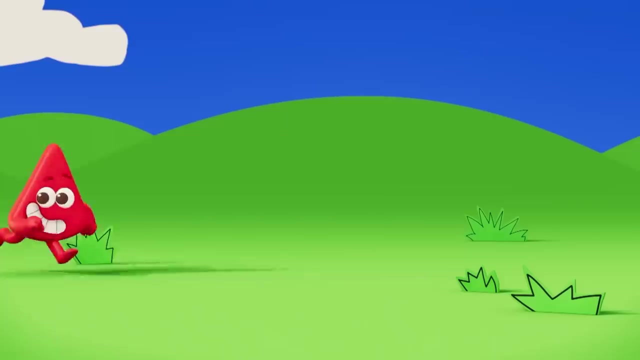 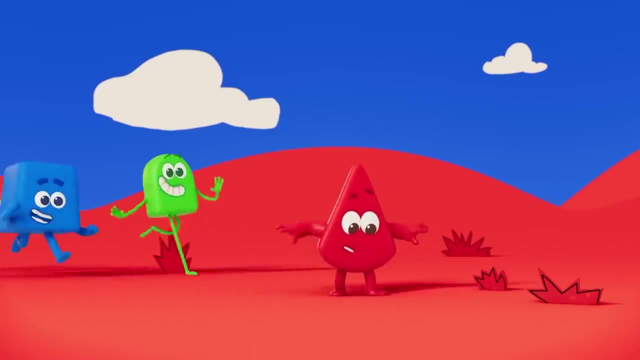 silly colouring. Yes, Let's see what other things we can colour differently. Hooray, Let's do it. Look, I'm going to colour these strawberries yellow, Exciting Me. next Red. Ooh, Look, The red grass is bouncy. 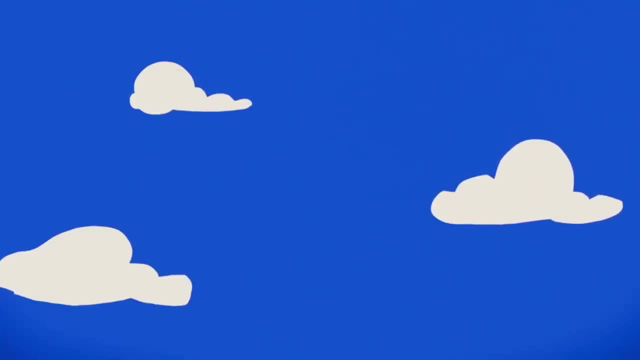 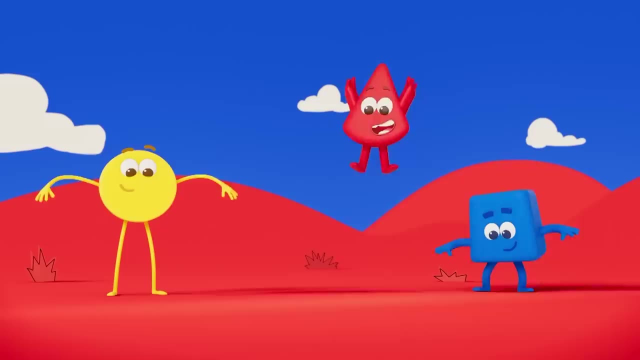 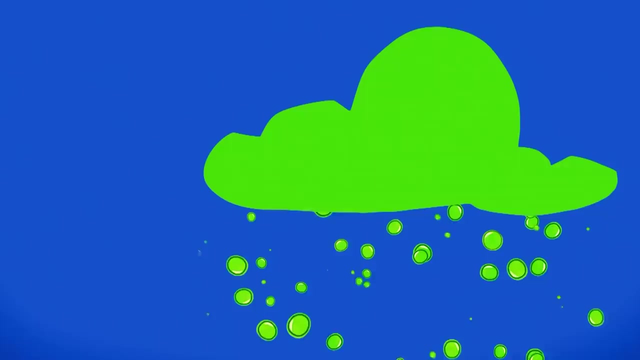 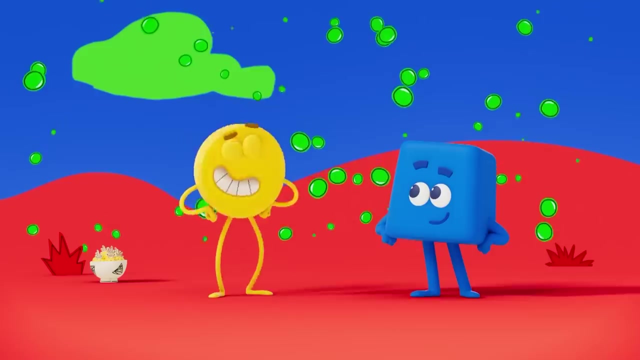 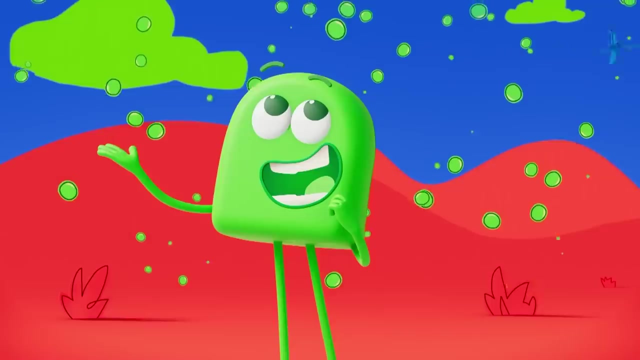 Yippee Cool Wahoo. Let's try some bright green clothes. Green Holy Wahoo, Woohoo, Wahoo. Silly colouring makes me happy. Whoa, Wahoo, Wahoo, Oh Ooh. 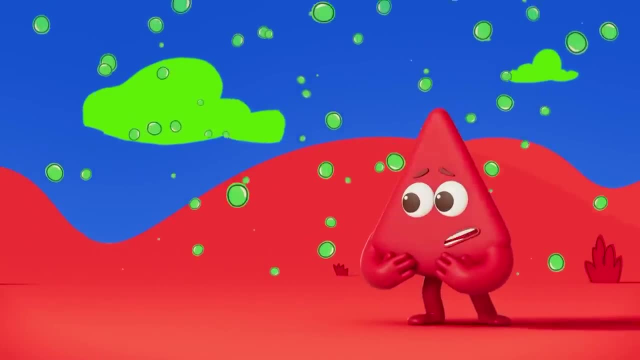 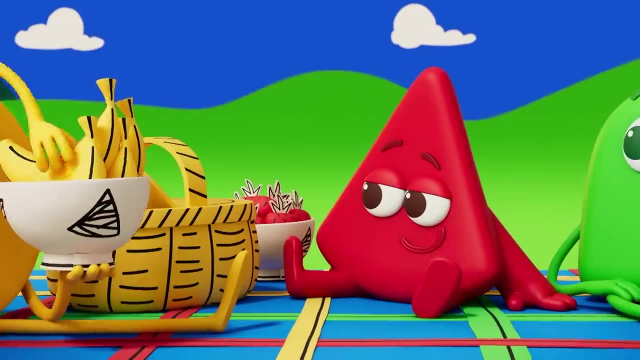 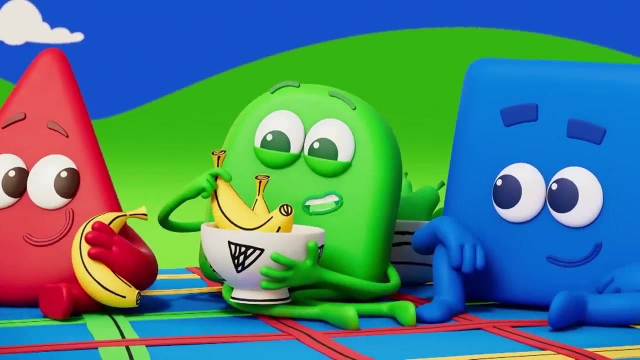 Ooh, I'm hungry again. Picnic this way. Phew, I'm glad it's a yellow banana. I'm too hungry for a silly blue one. It's good to colour things the colour they're meant to be, But it's cool to have silly colouring. 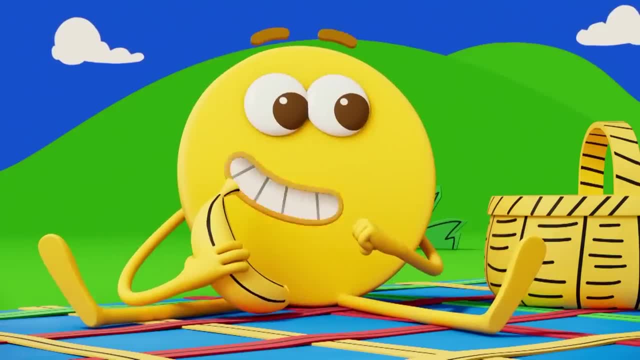 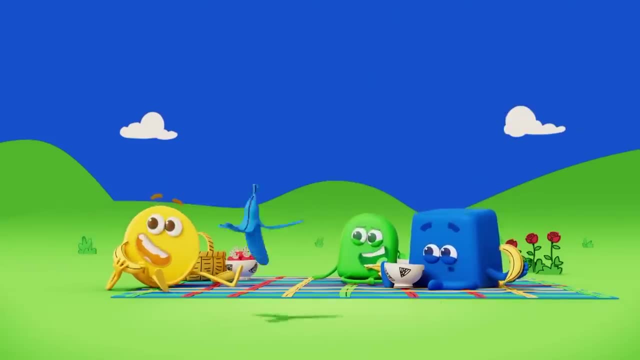 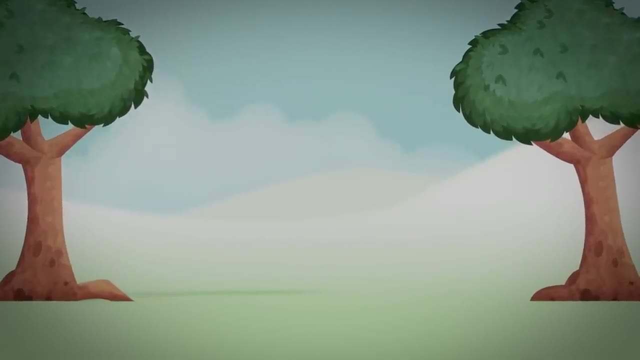 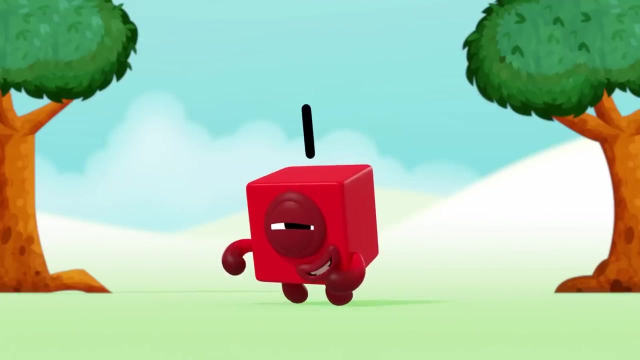 time too. You never know what fun things might happen. Uh oh, Here we go again. If there's nothing going on, no one's there and it's no fun. you can get the party started with a bang by adding one. I am one. 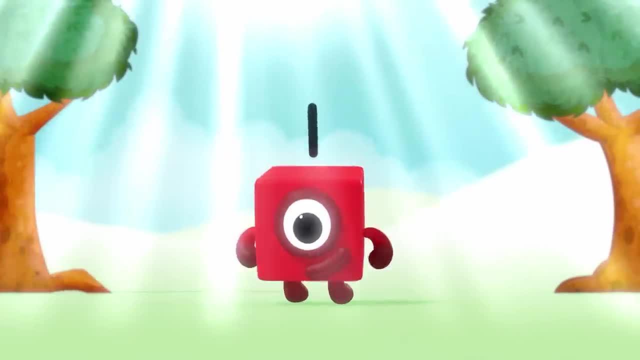 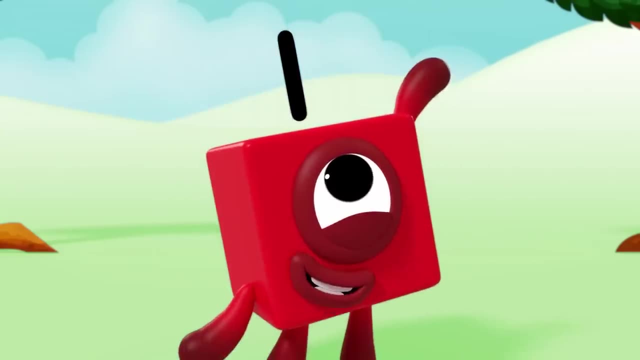 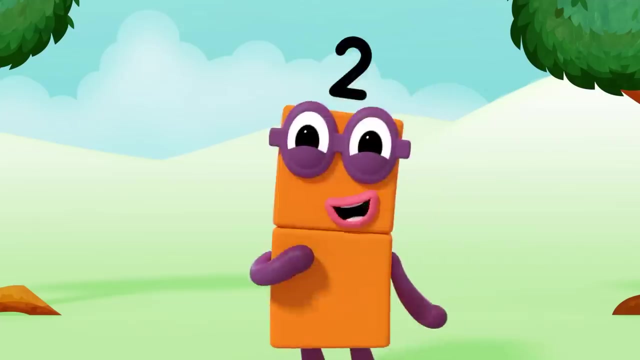 And I'm playing in the sun. being one, It's my idea of fun. One, One little block. Now let's add another one. One plus one equals two. I am two and I'm playing in the sun. A song and dance. 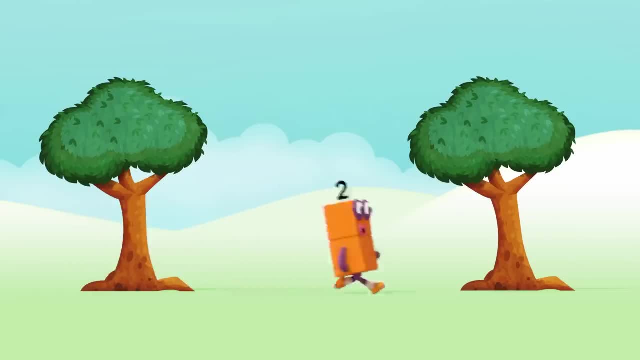 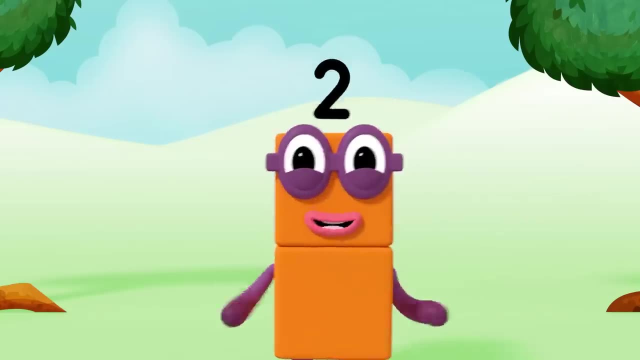 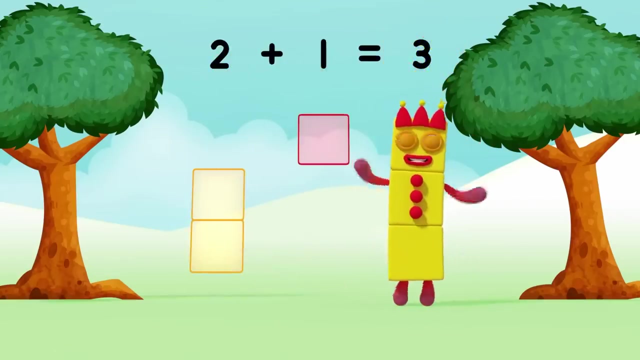 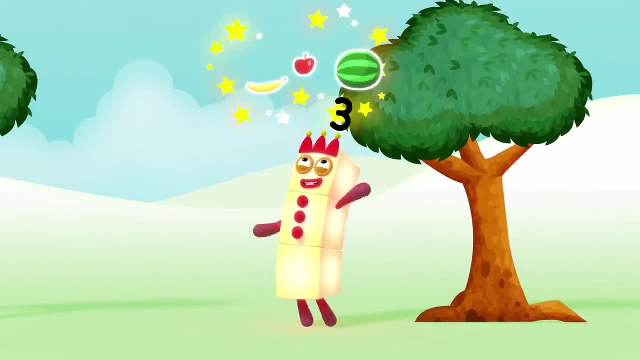 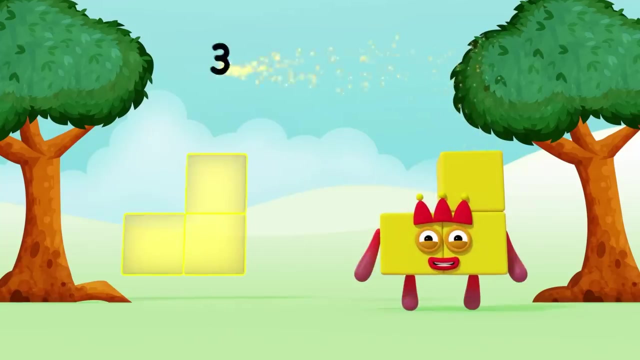 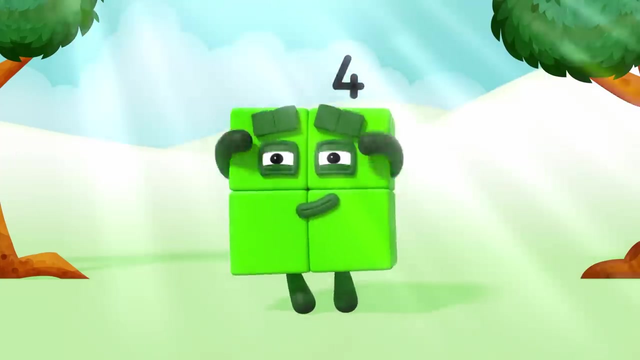 is my idea of fun. One, two, three, Three things. Look at me: One, two, three. Now let's add another one. Three plus one equals four. I am four and I'm playing in the sun, being square. It's my idea of fun. One, two. 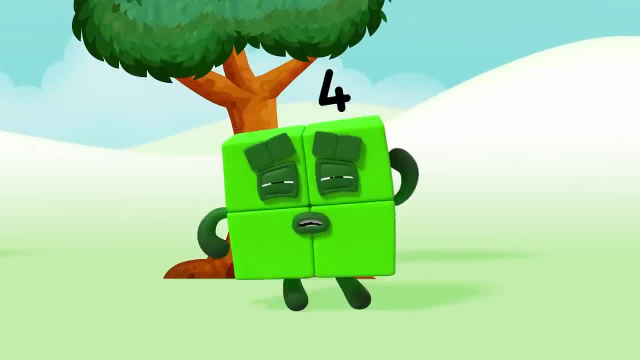 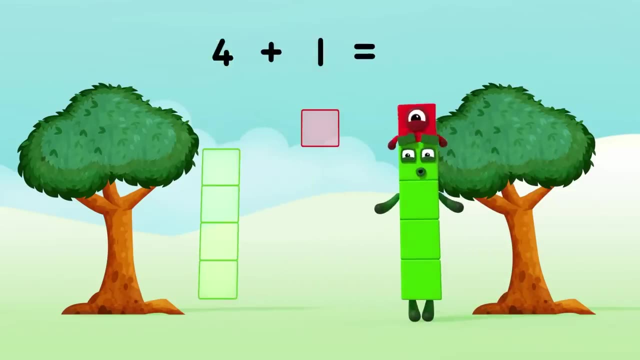 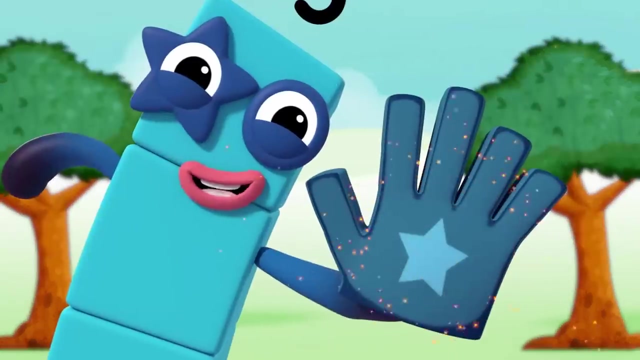 three, four, Four sides Out, out, out, out, Four corners. Now let's add another one. Four plus one equals five. I am five and I'm playing in the sun. High five, Or my idea of fun. One, two, three, four, five. 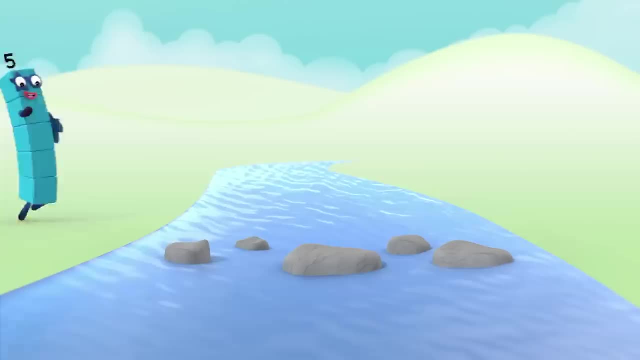 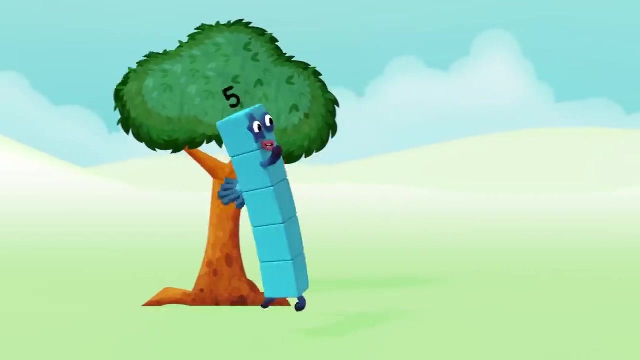 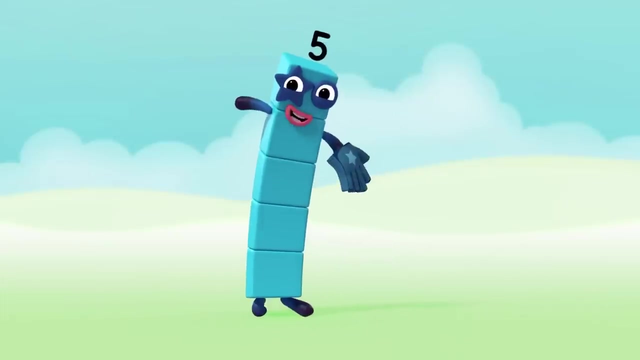 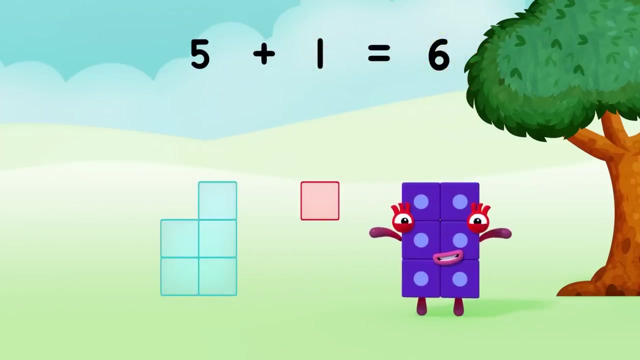 Five fingers. If you add another one, the number gets one bigger, And if you keep on adding one, you can get to any bigger. Now let's add another one. Five plus one equals six. I am six and I'm playing in the. 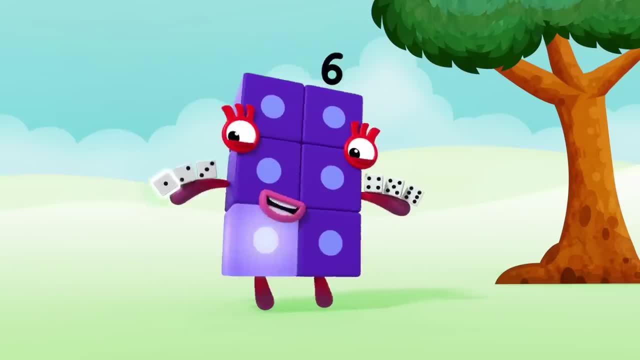 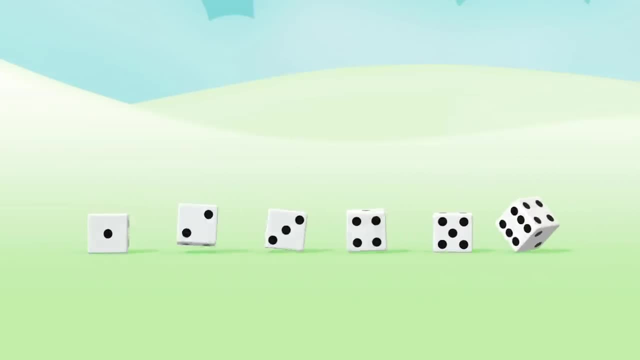 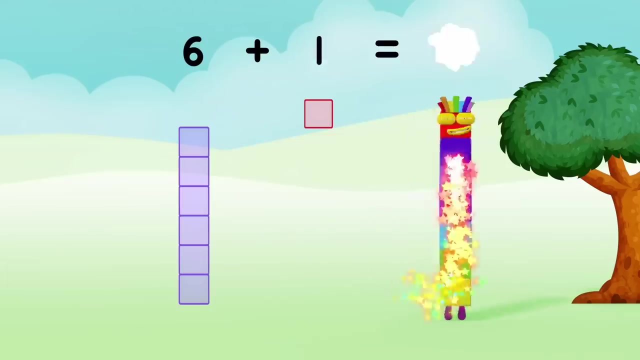 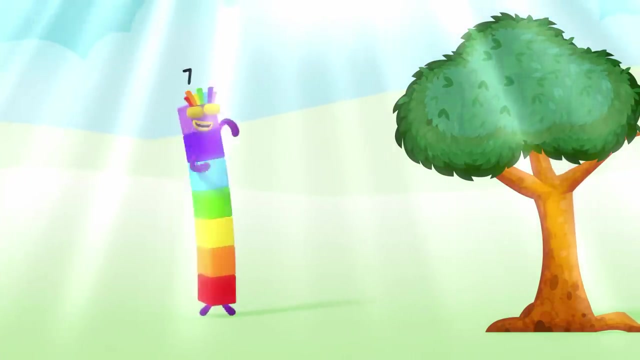 sun playing games. It's my idea of fun. One, two, three, four, five, six, Six dice. Now let's add another one. Six Plus one equals seven. I am seven and I'm playing in the sun making rainbows. It's my idea of fun. 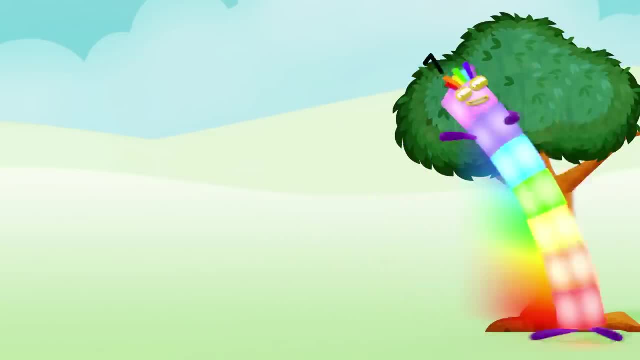 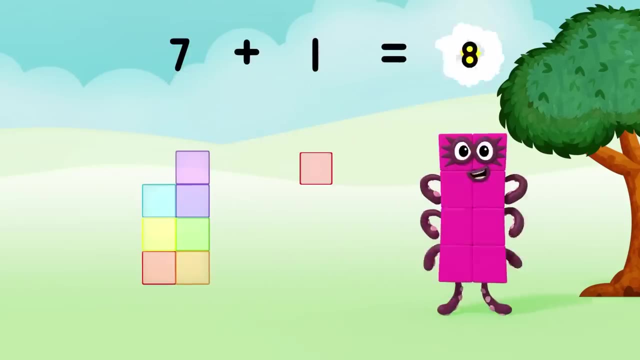 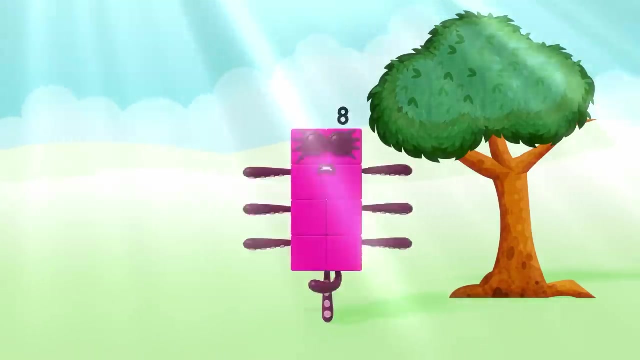 One, two, three, four, five, six, seven, Seven colours. Now let's add another one. Seven plus one equals eight. I am eight and I'm playing in the sun being Octoblock. It's my idea of fun Octoblock run. 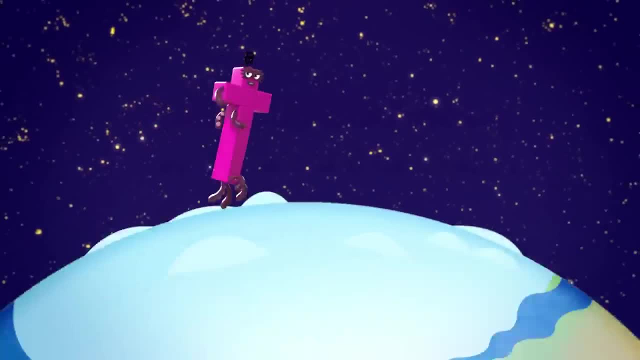 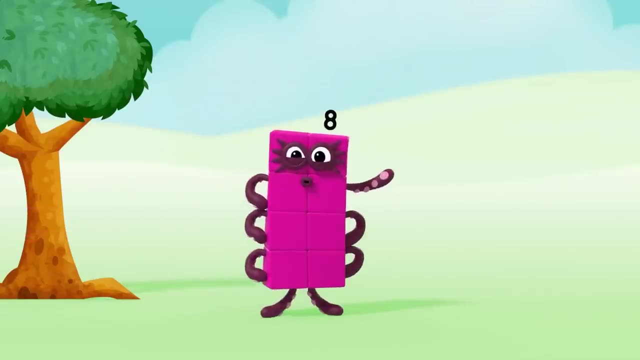 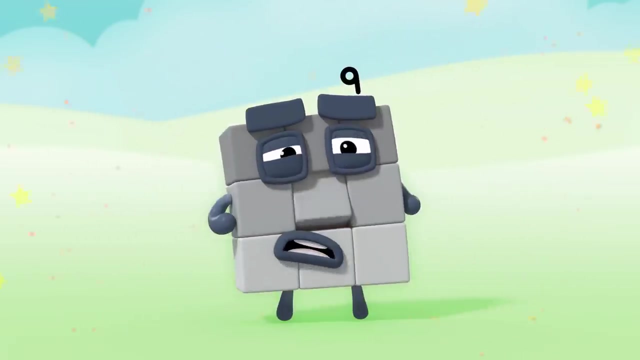 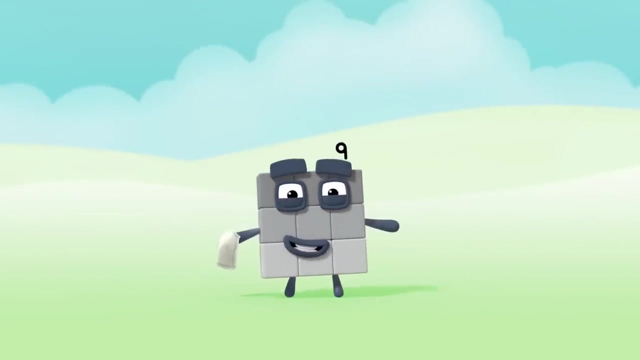 One, two, three, four, five, six, seven, eight run. Now let's add another one. Eight Plus one equals nine. I am nine, I am nine and I'm playing in the sun, not sneezing. It's my idea of fun. One, two. 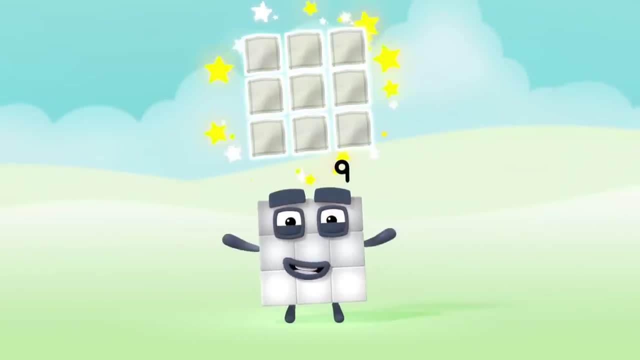 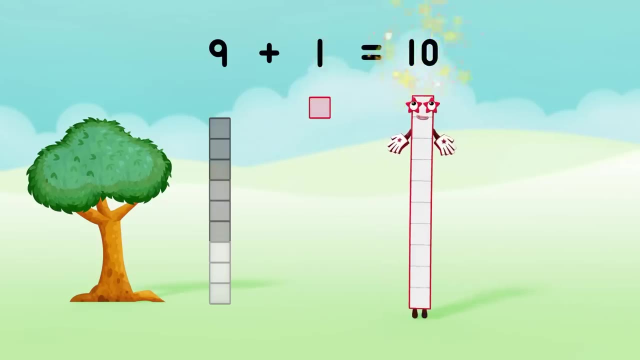 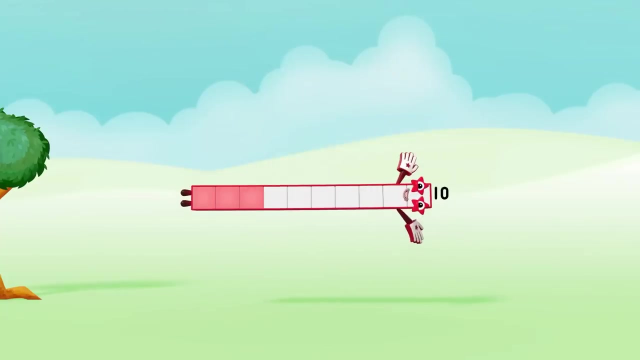 three, four, five, six, seven, eight, nine, Nine hankies. Now let's add another one. Nine plus one equals ten. I am ten and I'm playing in the sun. being ten, It's my idea of fun. One, two, three, four, five. 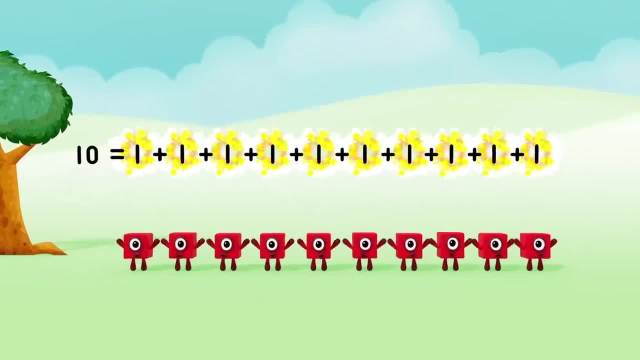 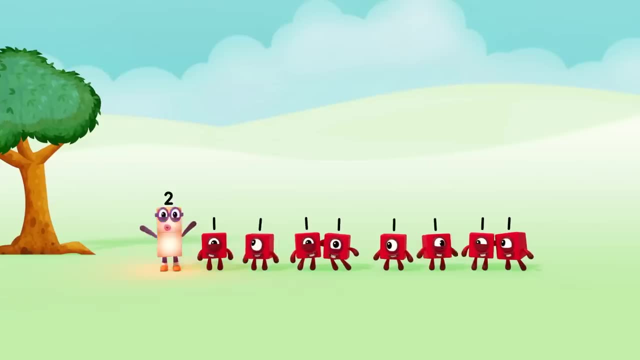 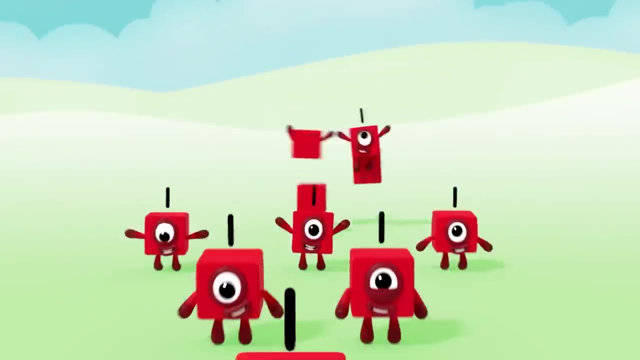 six, seven, eight, nine, ten, Ten blocks. We're ten ones and we're playing in the sun making friends. It's our idea of fun. One, Two, Three, Four, Five, Six, Seven, Eight, Nine, Ten. Remember this forever. 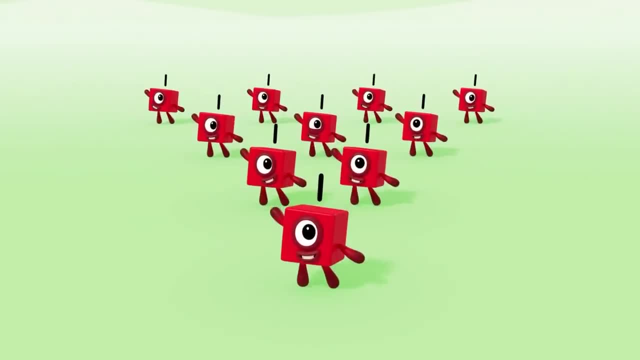 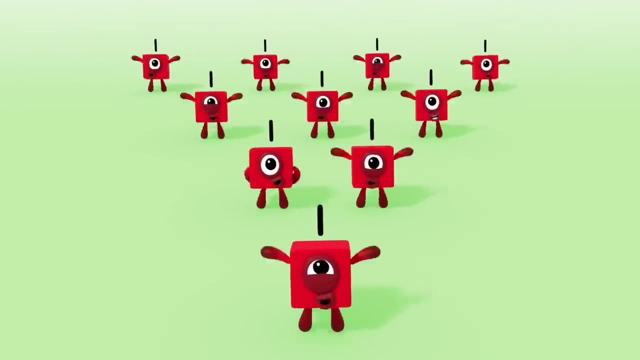 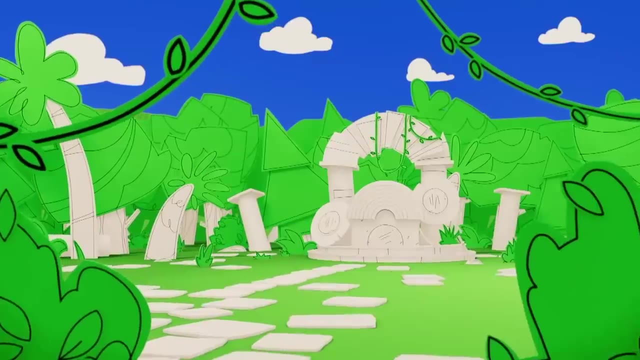 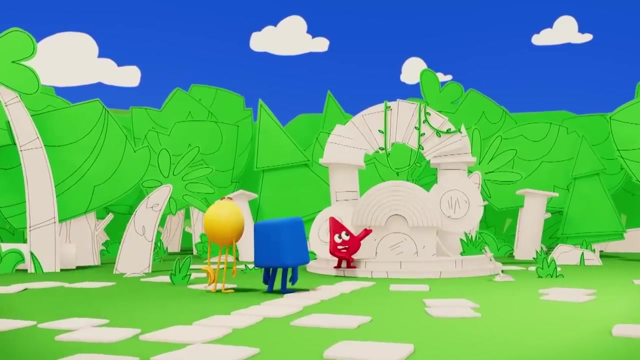 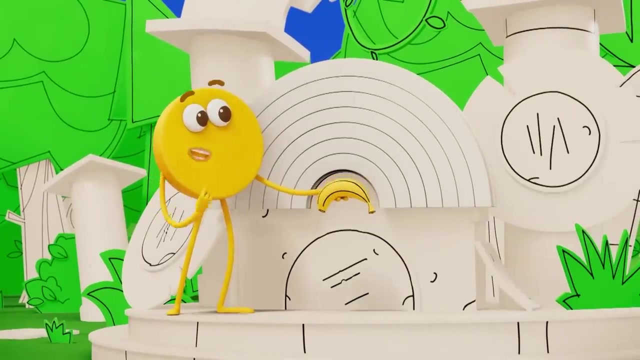 You can do what we've just done. You can make any number, Then you'll keep on adding one. That was fun. Yay, Look, Come and see these ruins. I found Cool. What is it? Bananas. It's a picture of seven bananas. 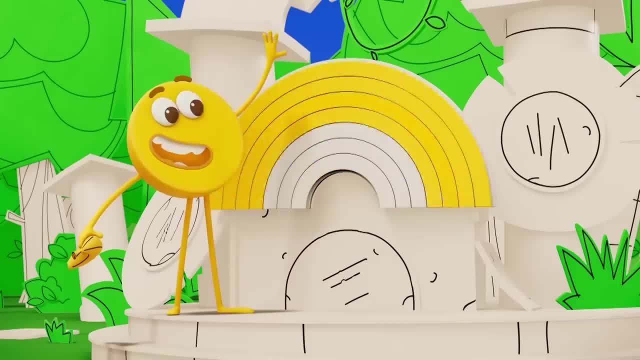 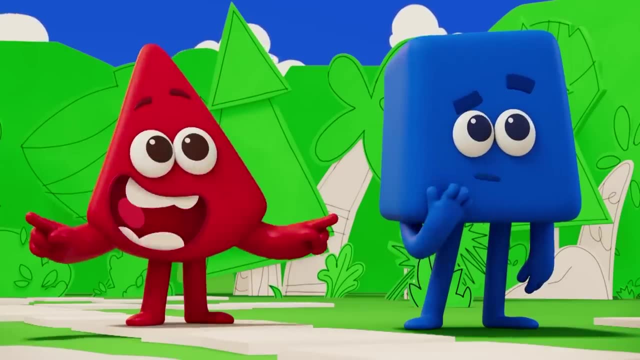 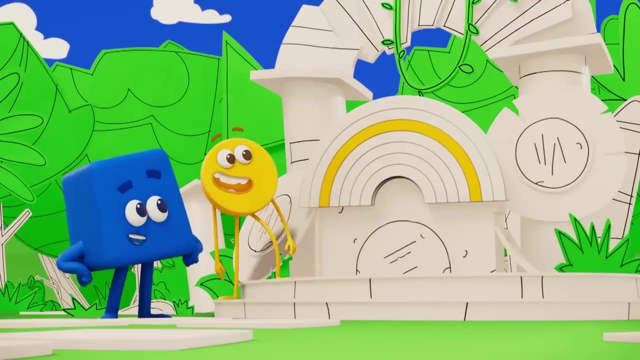 and they all need colouring yellow. Oh, They're not bananas yellow, They're curvy stripes. Hmm, I think this is some kind of puzzle, A colouring puzzle. Ooh, Exciting. Let's try colouring the other stripes. 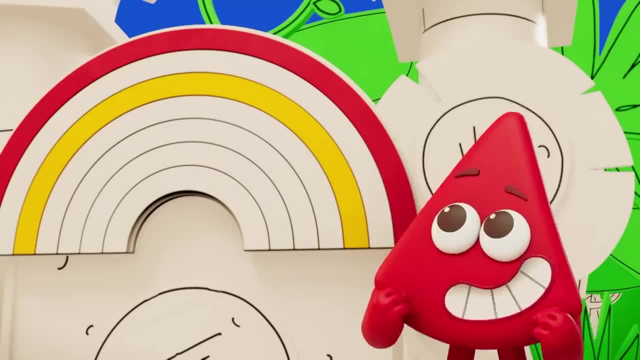 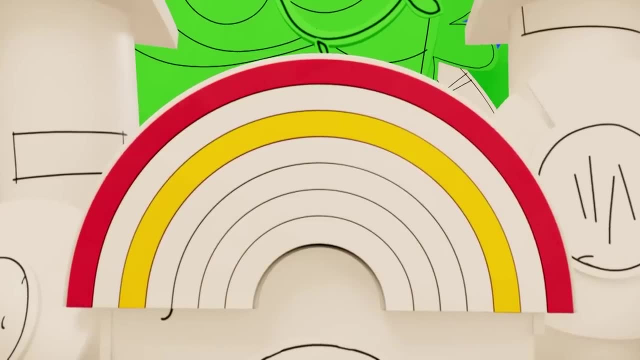 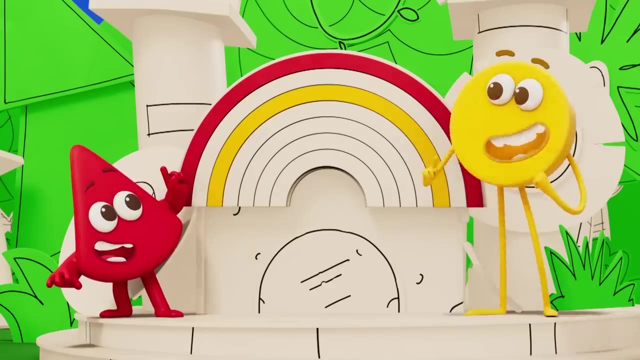 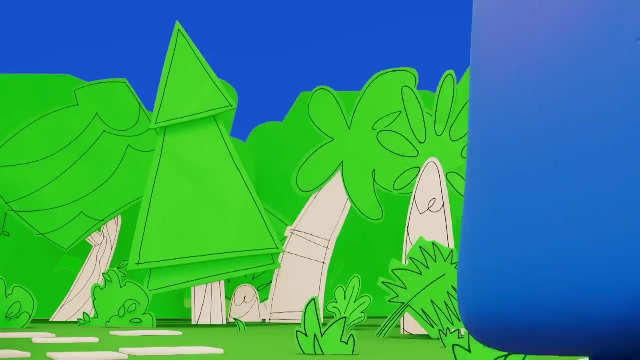 Red, Yes, Red at the top. Now, what goes between red and yellow? How about a bit of both? Oh, yes, Red and yellow mix to make orange. It must be me next Blue, Hmm, Maybe the next one Blue. 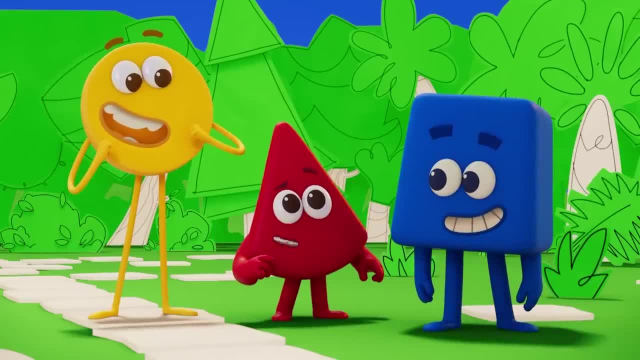 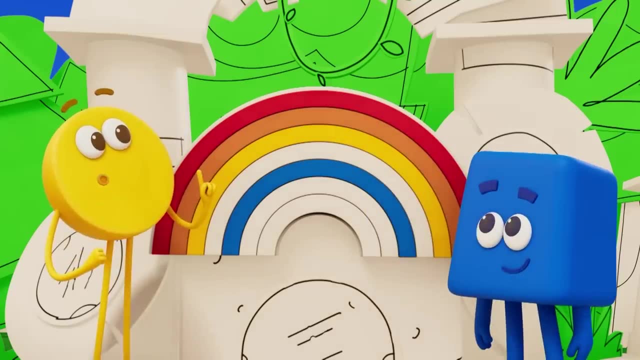 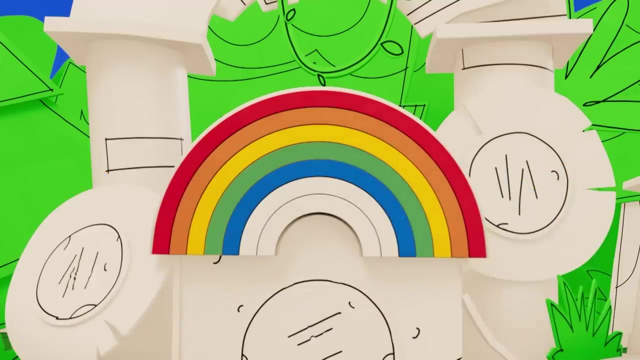 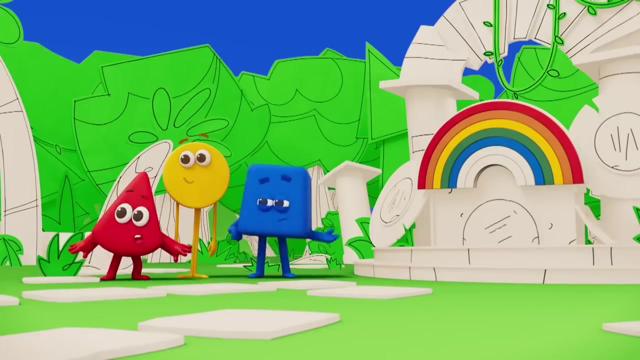 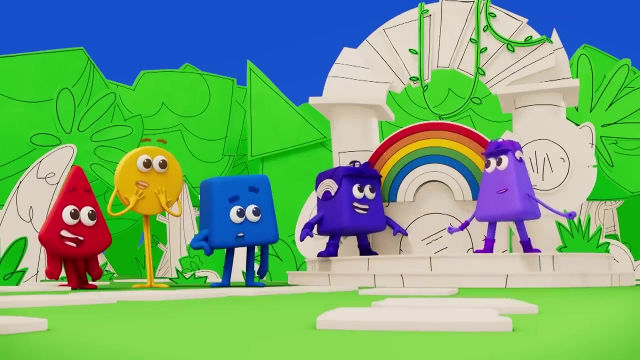 Yay, But what comes between yellow and blue? Hmm, Another mix, Yellow and blue mix to make green. Wow, So we have red, orange, yellow, green and blue. What could come next? Indigo Violet, Is it here? 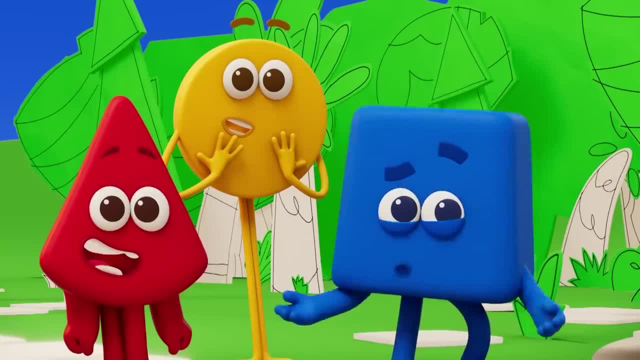 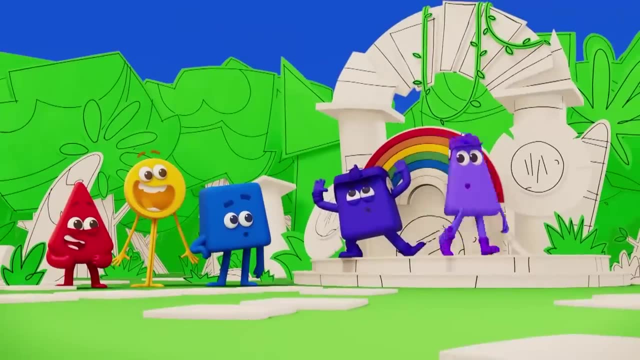 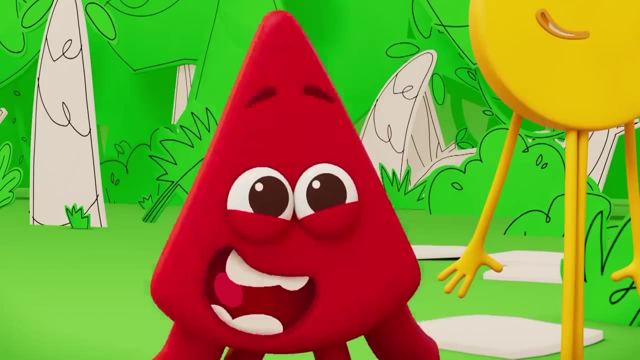 Have we finally found a rainbow? Err, Who are you? Oh, I'm Indigo And I'm Violet, And we're Rainbow Chasers, But We've never actually seen one. Wow, What is a rainbow? It's when you see colours in the sky. 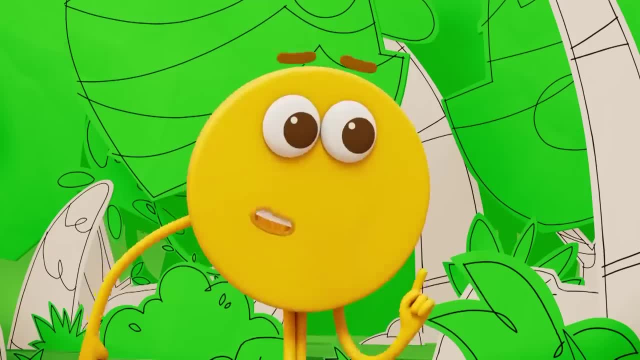 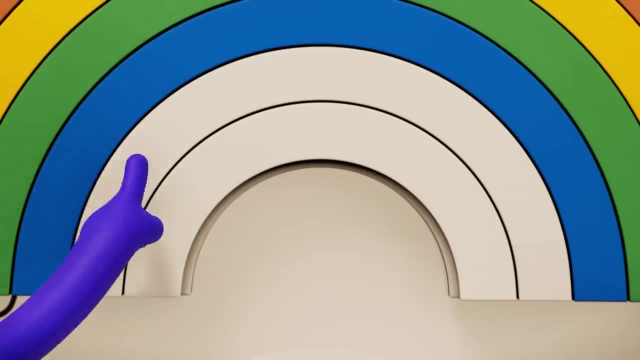 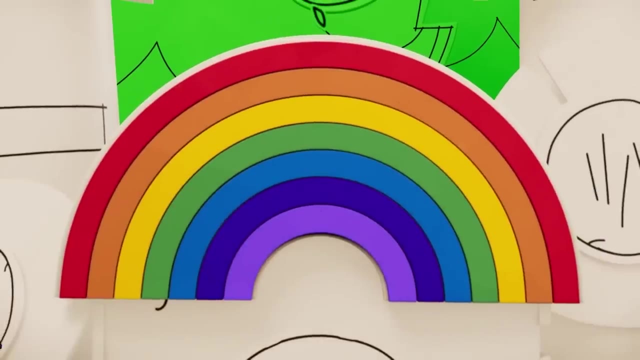 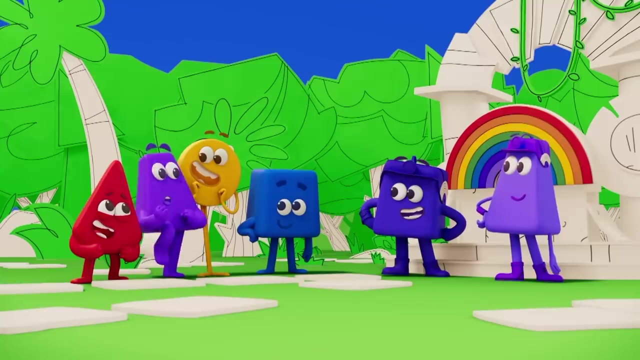 together. Oh, A bit like that. That's our puzzle, But we're missing two colours: Us Every rainbow needs Indigo And violet. Oh, Oh, What's going on here? Purple, I imagine you're Oh New colours. 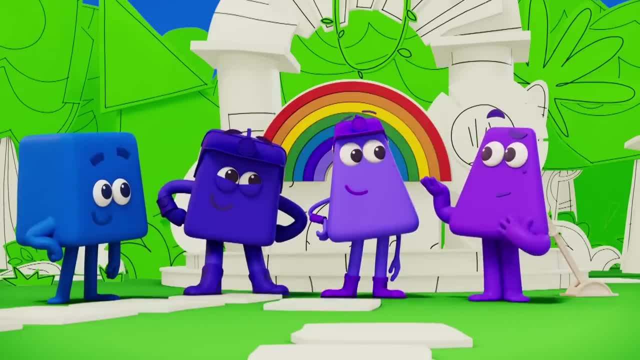 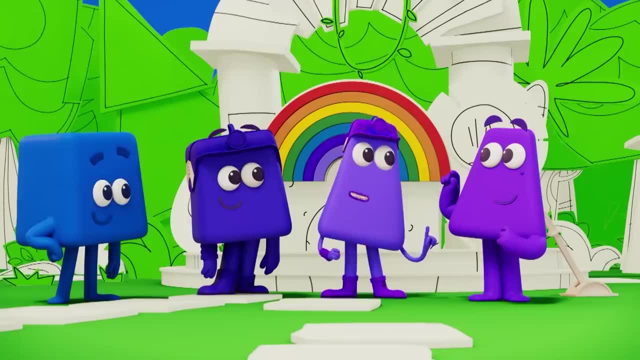 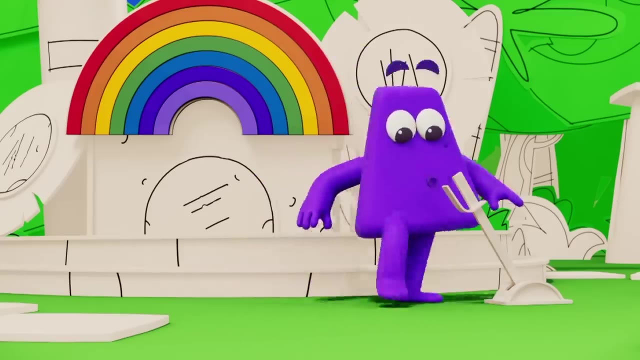 Wait, Have I seen you before? I'm Indigo. I'm like blue, but a bit more purple. I'm like you, purple but a bit more blue. And what's this? A rainbow? Ah, Oh, Then I imagine this must be a. 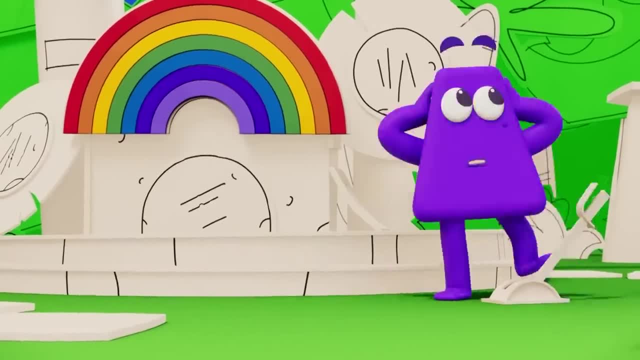 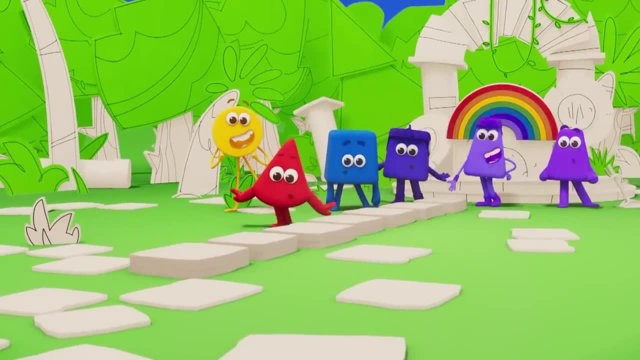 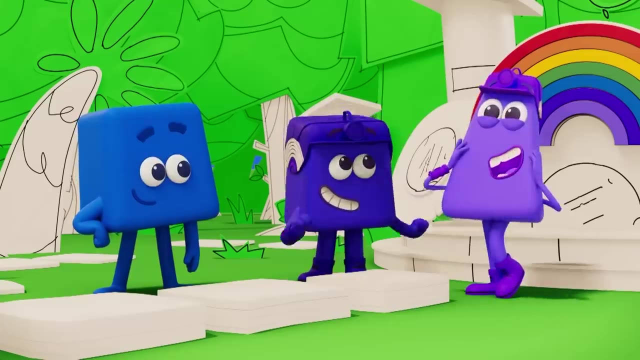 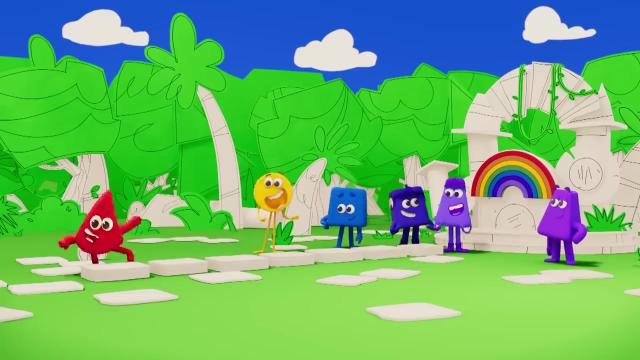 rainbow lever. Oh crux, What's happening? Wow, We've unlocked another puzzle. Maybe this one will lead us to a real rainbow. We'll finally see one. I imagine you all need to stand on a stone, But we're missing two. 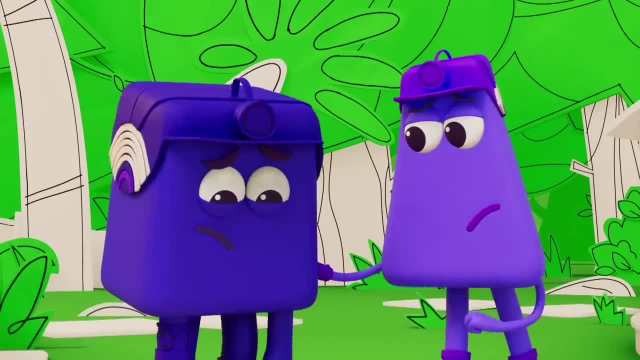 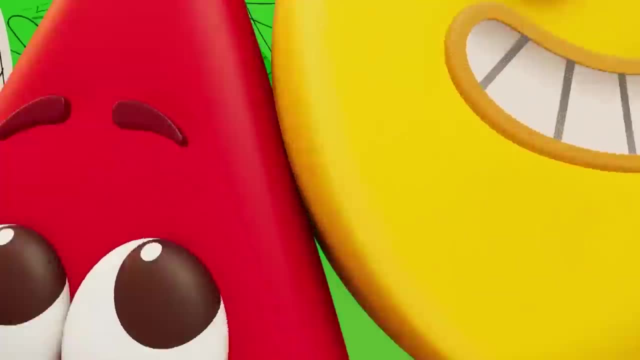 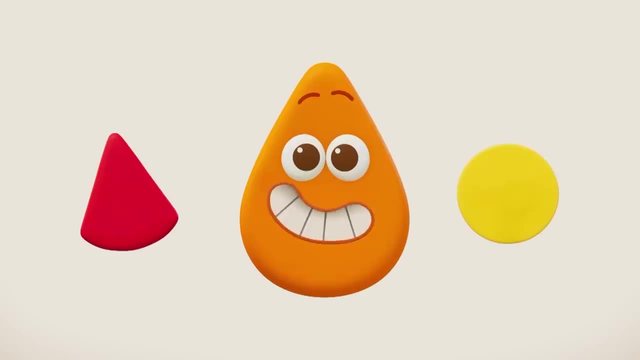 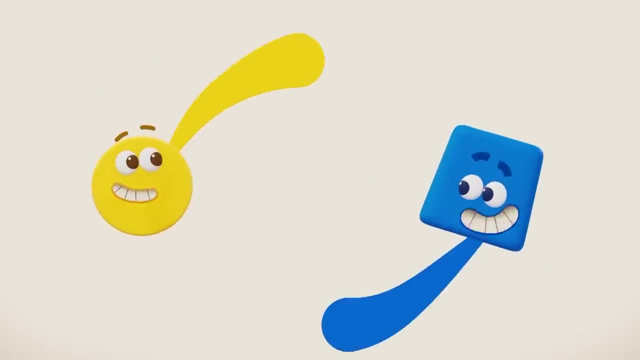 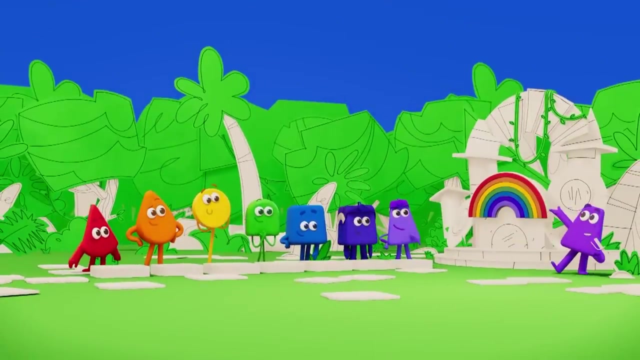 colours. We can't finish the puzzle, Don't worry, We've got friends that can help. Mixing time: Oh, Red and yellow mix to make orange. Yellow and blue mix to make green. We need your help to solve this rainbow puzzle, Everyone. 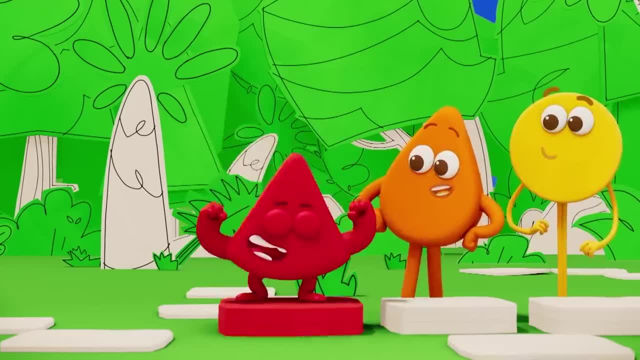 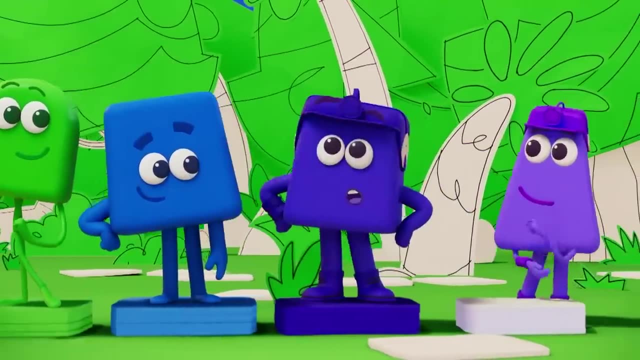 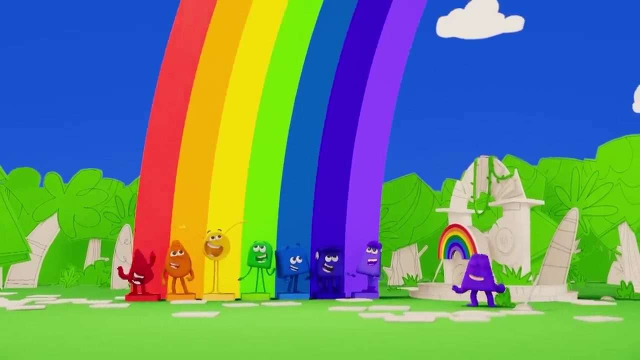 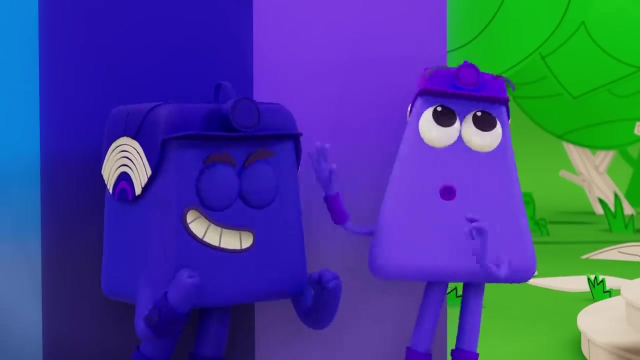 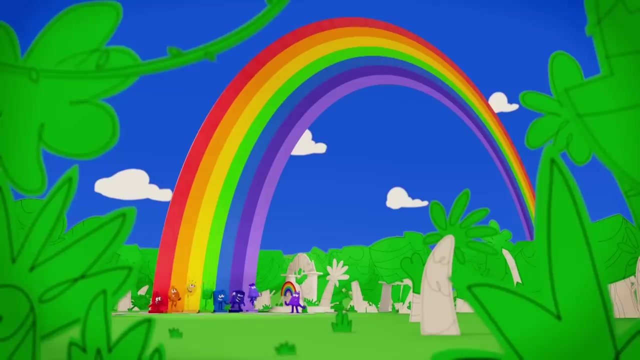 stand on your stones, Me first. Red, Orange, Yellow, Green, Blue, Indigo, Violet, Oh, Ah, Whoa, Wow, Finally We've seen one, A rainbow. Yay, Yay, Yay. 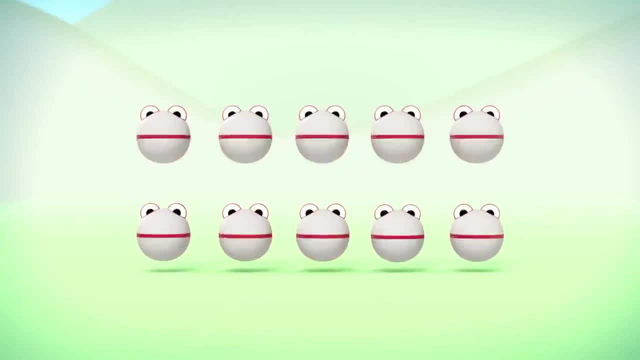 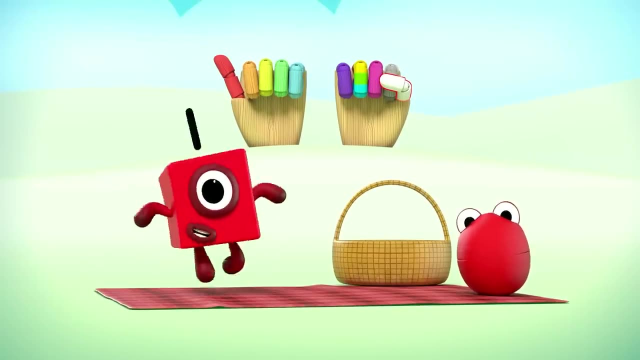 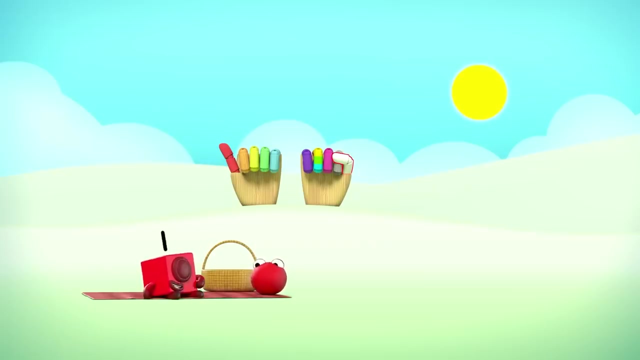 Yay, Number blobs: One, Two, One, Two, Three, Four. One number blob and me Counting everything we see, Sharing a bun, Sitting in the sun, Whistling a happy melody: One number blob And me. 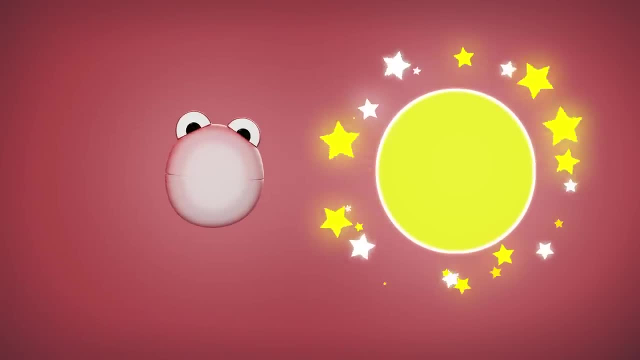 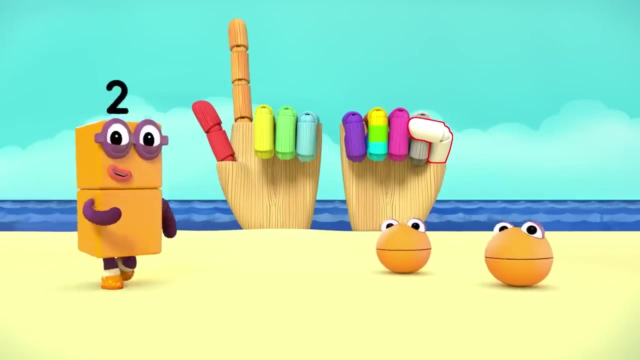 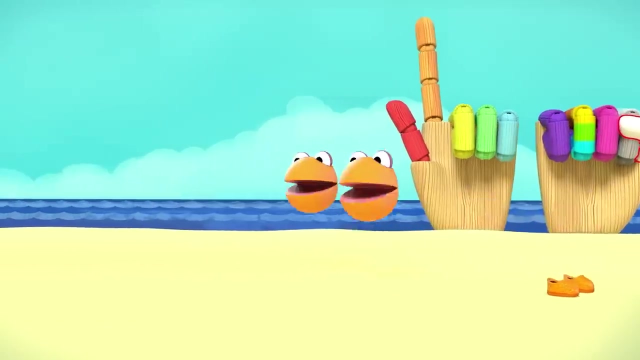 One One bun. One One sun. One number blob And me. Two number blobs and me Counting everything we see Taking off our shoes, Looking for the clothes, Whistling a happy melody. Two number blobs And me. 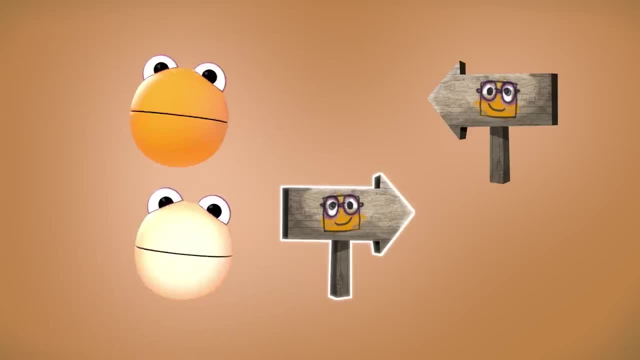 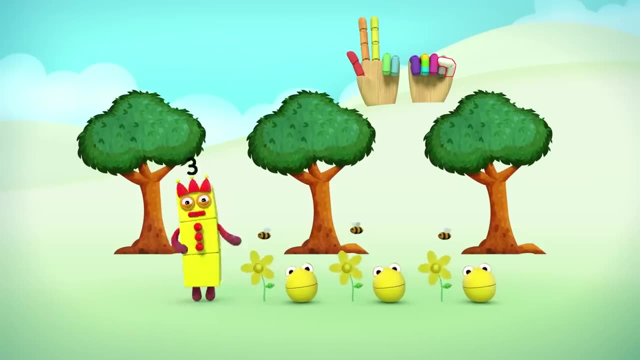 One Two, Two shoes, One Two, Two clothes, Two number blobs And me Three number blobs and me Counting everything we see Hiding in the trees, Buzzing, with the bees Whistling- a happy melody. 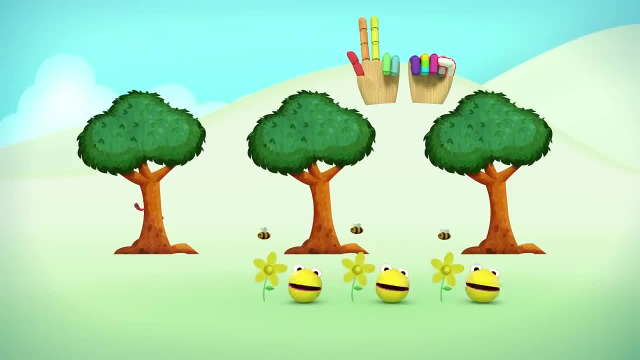 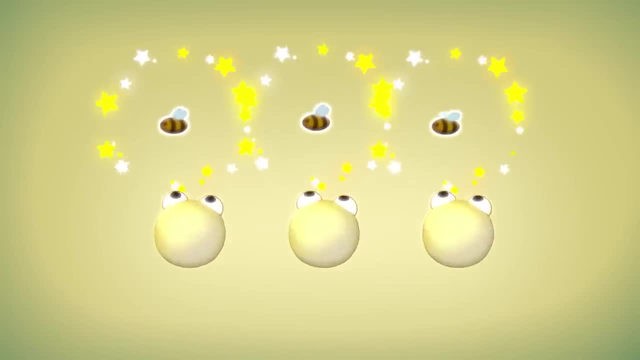 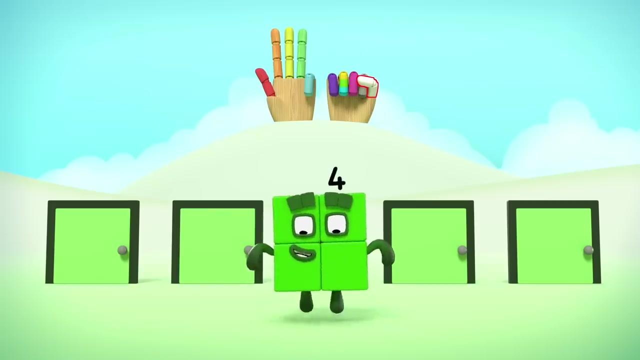 Whistling a happy melody: Three number blobs And me One, Two, Three, Three trees, One, Two, Three, Three bees. Three number blobs And me. Four number blobs and me Counting everything we see. 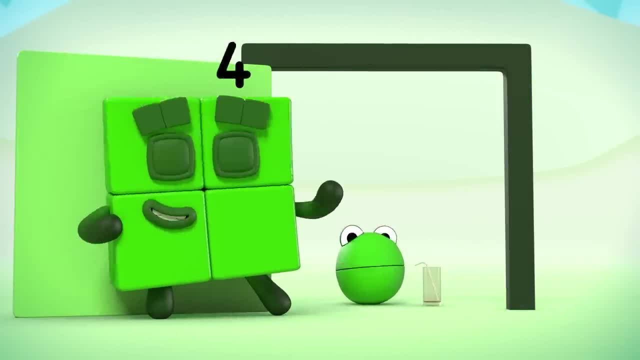 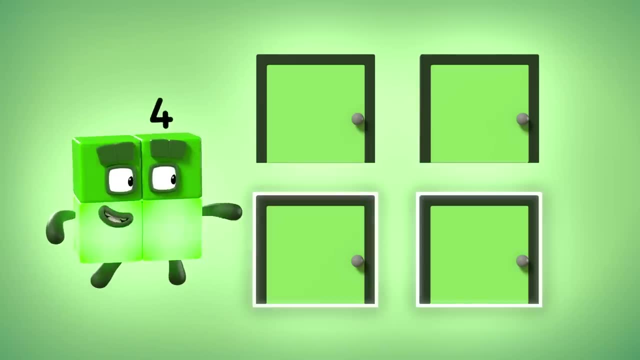 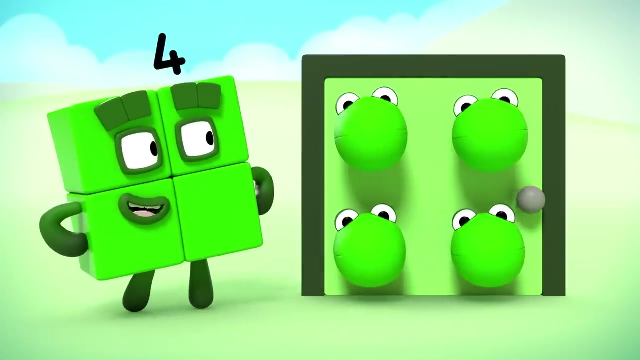 Opening the door, Surfing through a storm, Whistling a happy melody, Whistling a happy melody. Four number blobs And me. One, Two, Three, Four, Four stores. Four number blobs And me. Five number blobs and me. 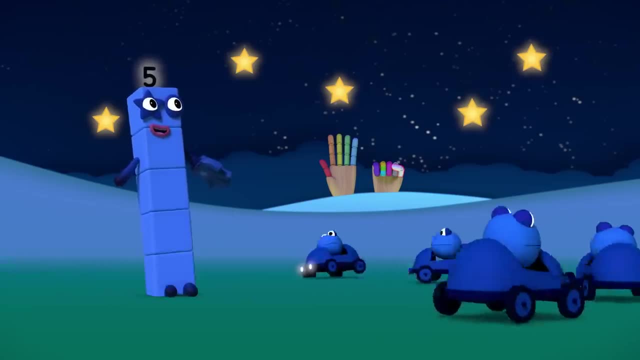 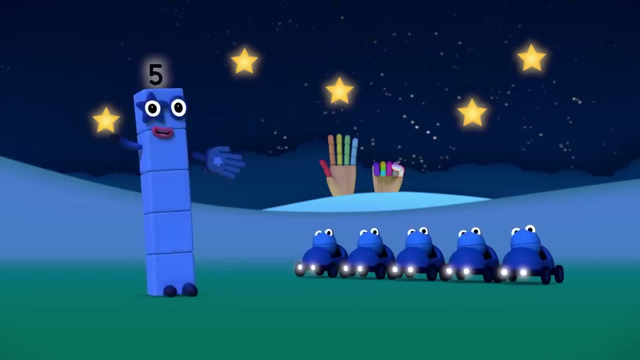 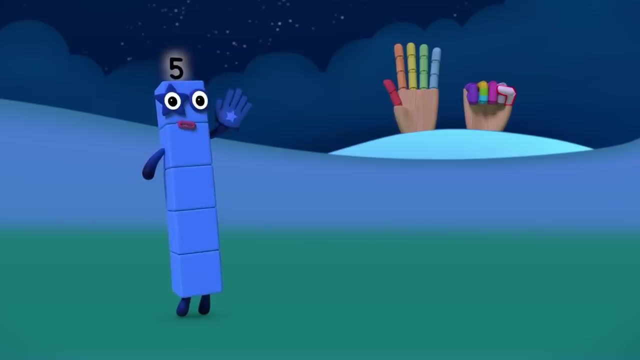 Counting everything we see, Gazing at the stars, Parking all the cars Whistling a happy melody, Five number blobs And me: One, Two, Three, Four, Five, Five stars, Five cars, Five number blobs. 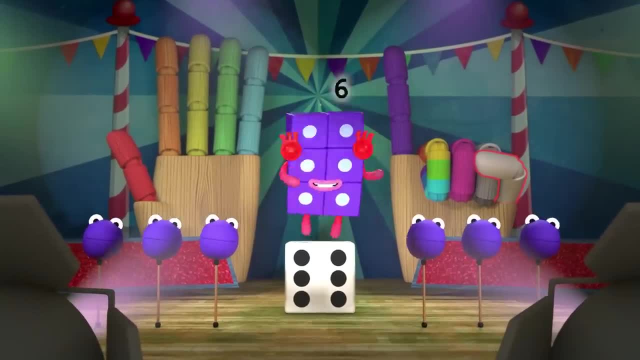 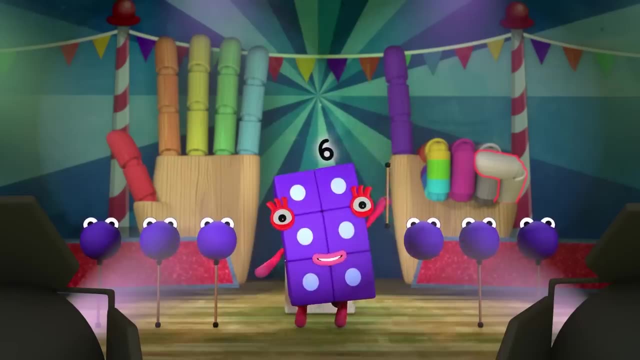 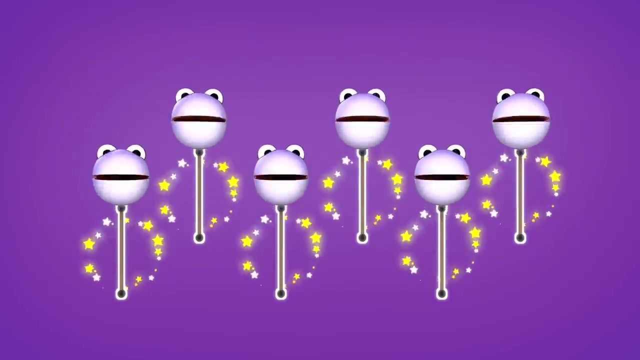 And me Six number blobs and me Counting everything we see Picking up a stick, Showing off a trick, Six number blobs And me One, Two, Three, Four, Five, Six sticks, Six tricks, Six number blobs. 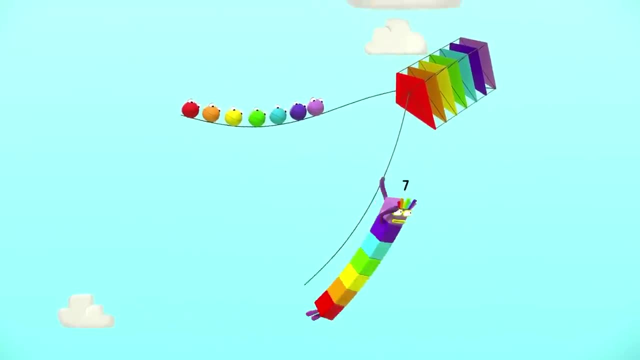 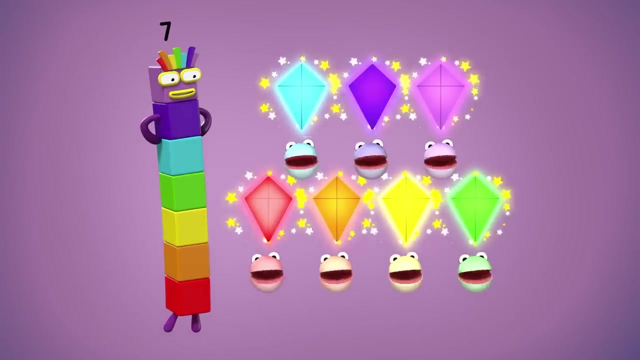 And me Seven number blobs and me Counting everything we see Flying a kite, Rainbow lights, Seven number blobs And me One, Two, Three, Four, Five, Six, Seven, Seven kites. One, Two, Three, Four, Five, Six. 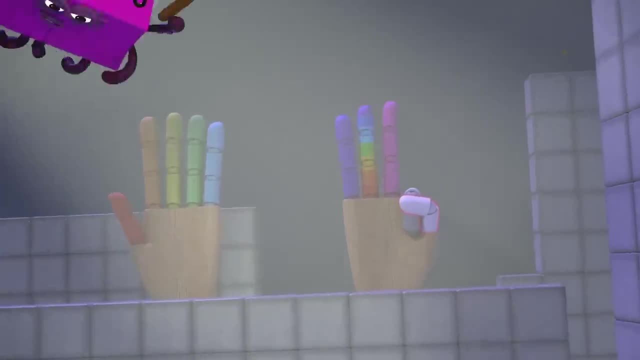 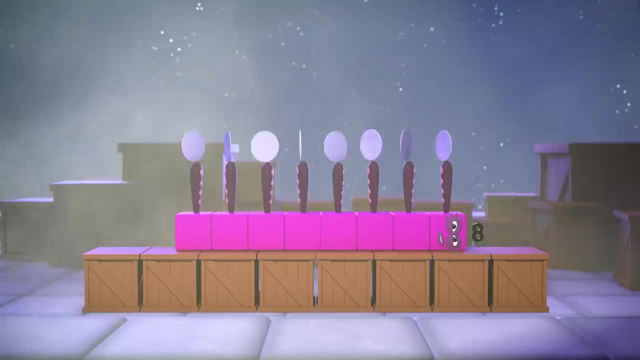 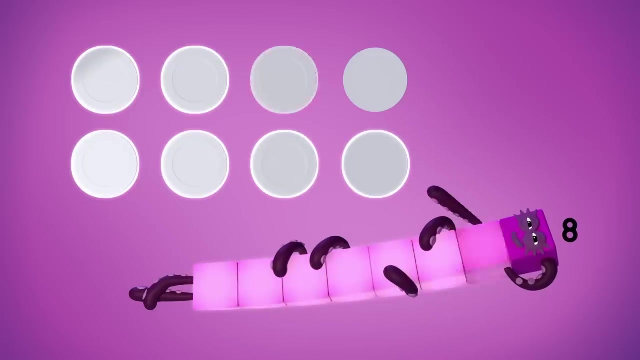 Seven, Seven lights, Seven number blobs And me Eight number blobs and me Counting everything we see, Spinning all the plates Off the block, spin Lifting all the crates: One, Two, Three, Four, Five, Six. 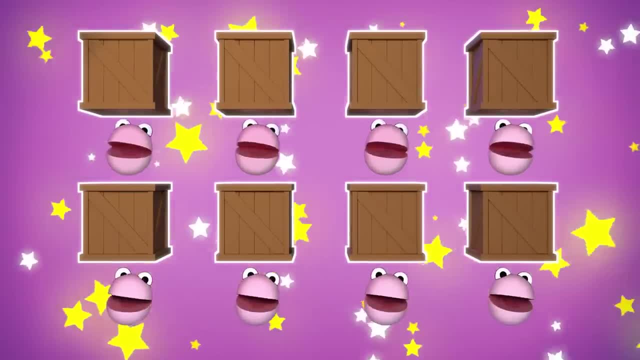 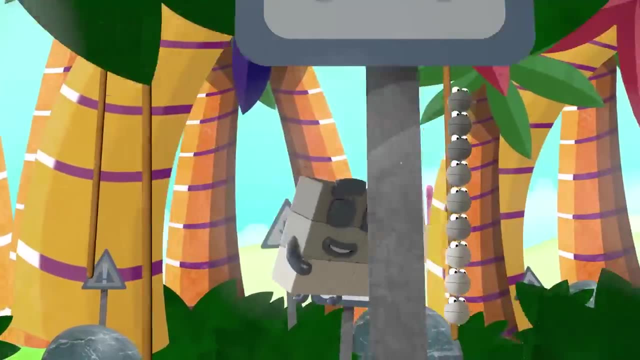 Seven Eight Eight plates. One, Two, Three, Four, Five, Six, Seven Eight Eight plates. Eight number blobs And me. Nine number blobs and me Counting everything we see Swinging through the vines. 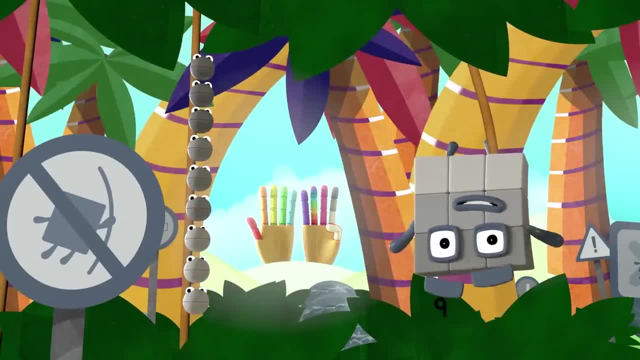 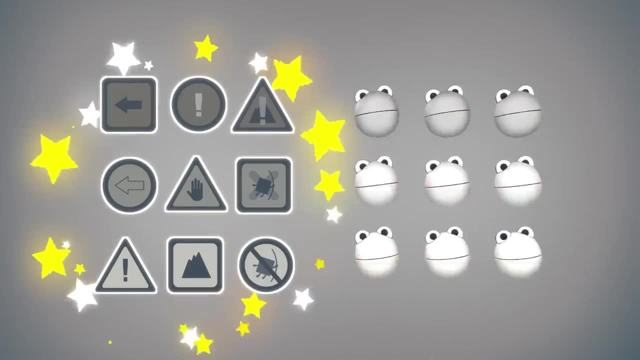 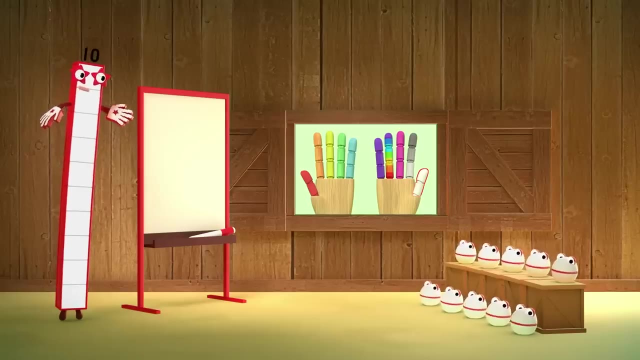 Ignoring all the signs: Nine number blobs And me One, Two, Three, Four, Five, Six, Seven, Eight, Nine, Nine vines And me Ten number blobs and me Counting everything we see Writing with a pen. 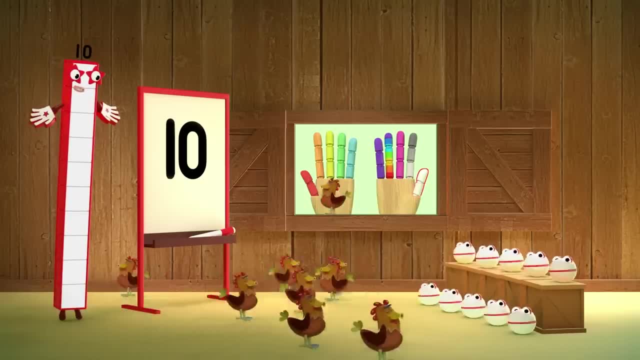 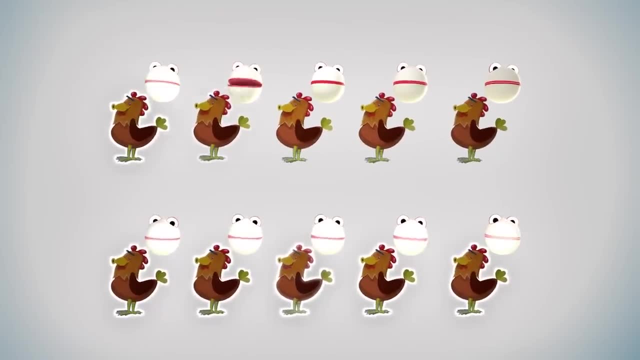 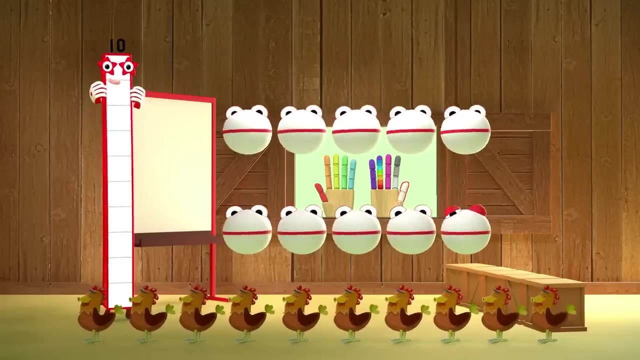 Plucking like a hen. Ten number blobs And me One, Two, Three, Four, Five, Six, Seven, Eight, Nine, Ten, Ten pens. Ten number blobs And me Ten colored pens. Ten little hens. 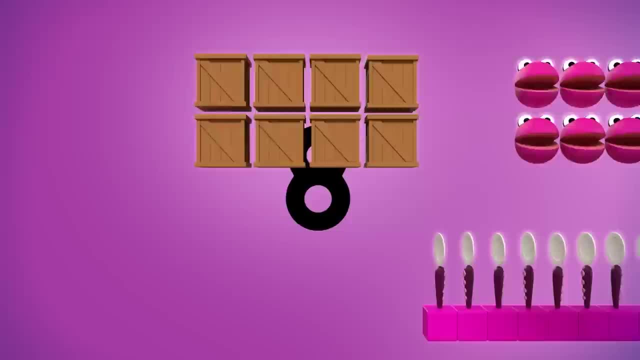 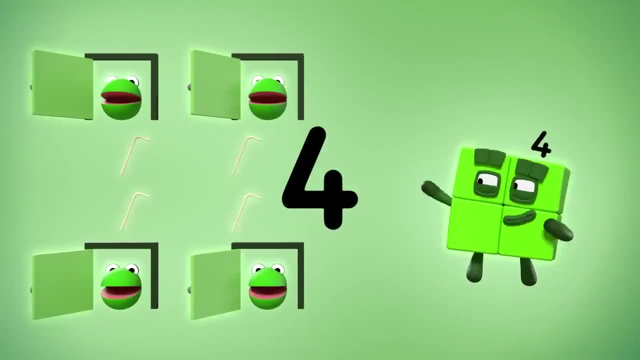 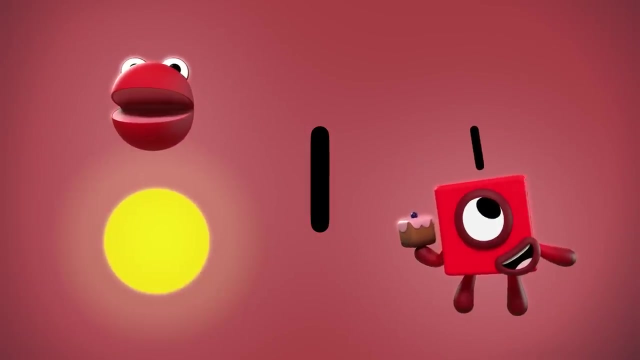 Nine swinging vines, Eight spinning plates, Eight heavy crates, Seven floating kites, Seven rainbow lights, Six wooden sticks, Six clever tricks, Five shooting stars, Five motor cars, Four open doors, Four bendy stores, Three leafy trees. 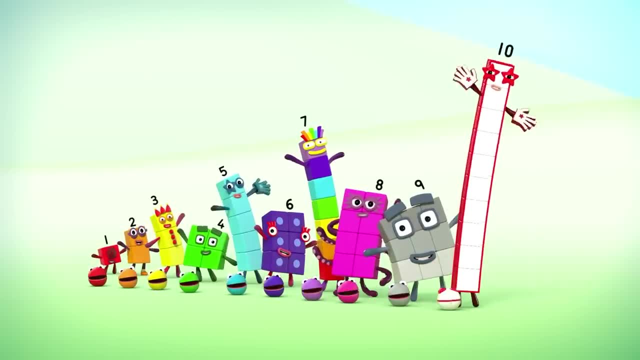 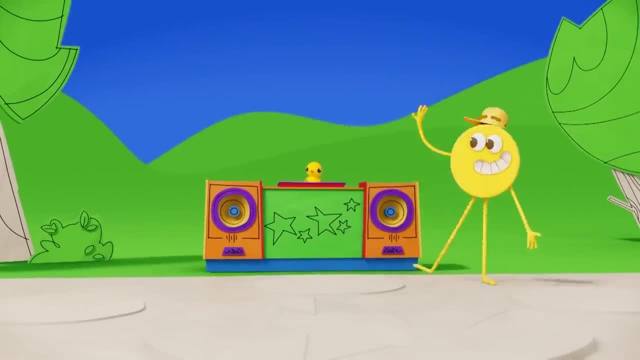 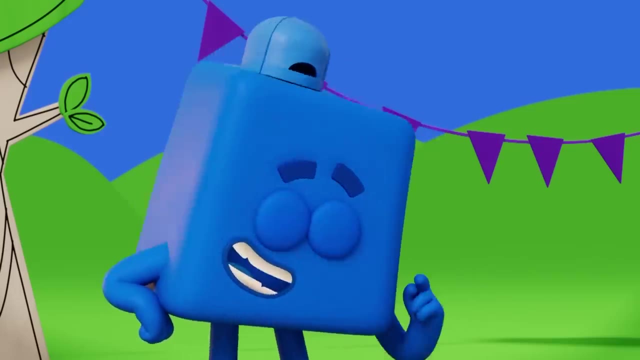 Three moldy leaves, Two dancing shoes, Two vital clues, Two: DJ Ducky's disco dance floor. I can see DJ Ducky, but where's the dance music? And what's with the cool hats? You'll see Now. everyone find their spot around the dance floor. 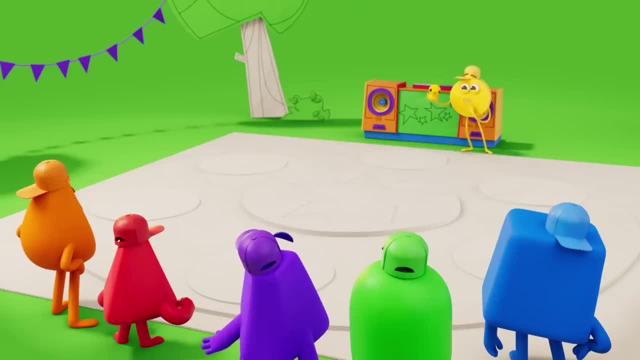 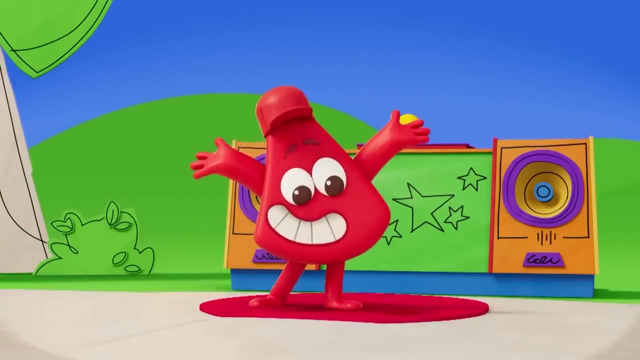 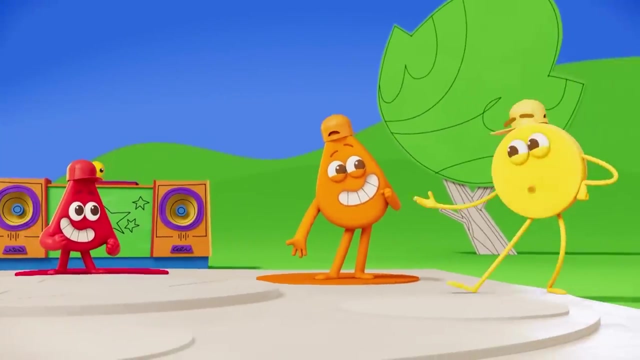 DJ Ducky says: go around in color order, Exciting, I'll go first Red. I'm like you Red, so I'll go next Orange And I'm like you Orange, so yellow goes here. This spot has blue all over it. 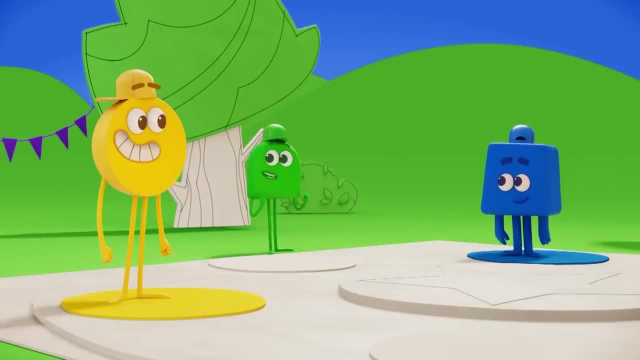 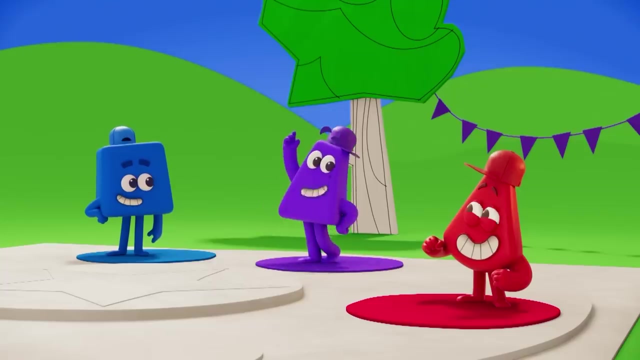 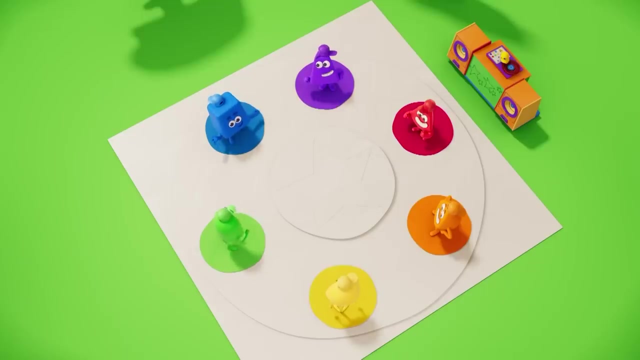 Naturally I go between you two. because Yellow and Blue mix to make Green. I imagine this must be my purple spot, The royal place between blue and red. Cool, We join up in a color circle. It's like a wheel. 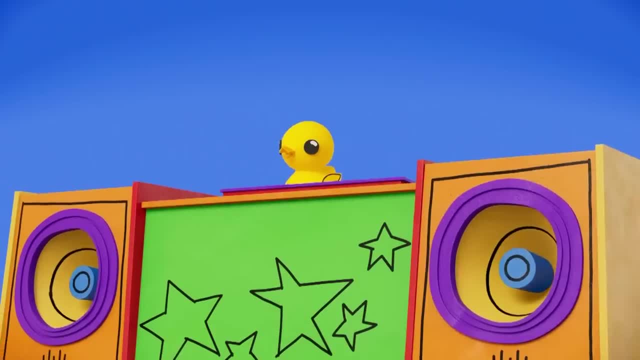 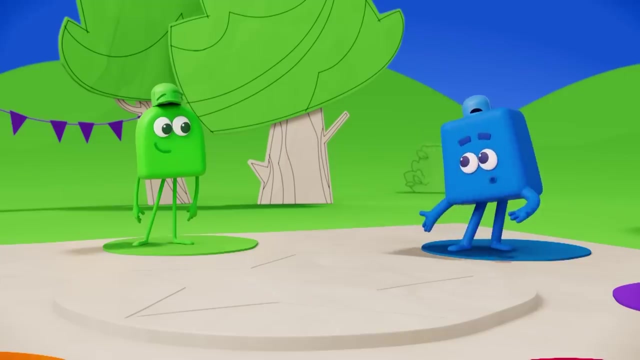 A color wheel. Ooh Nice, Who wants to be the first to dance in the middle? I'll go first. Pick a partner, up to you. Who's it gonna be? Who, who, who? I pick the color next to me. 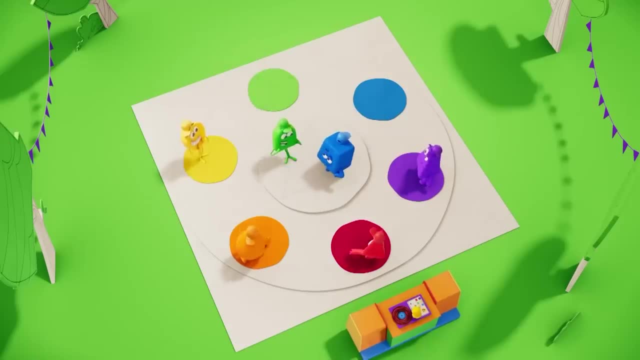 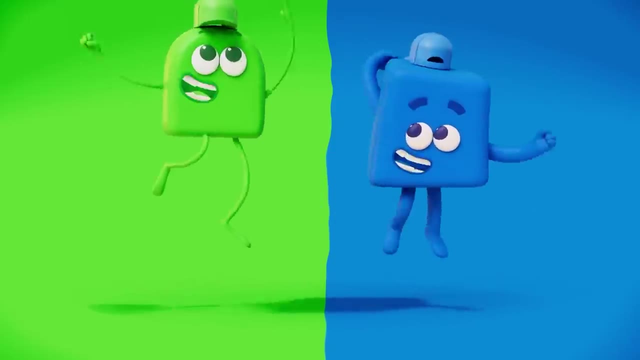 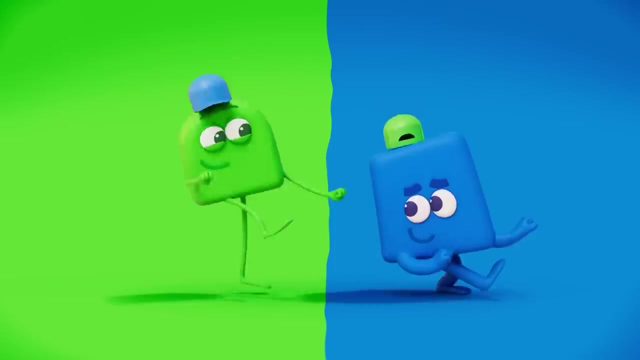 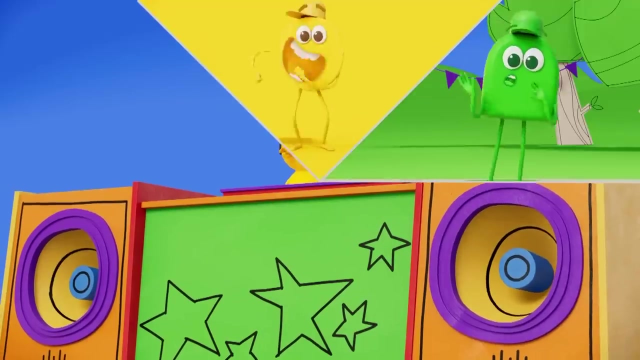 Green, Yay Swap. I love that combination. They go so well together. That's because blue And green Are close color friends. We're similar colors. Ooh, Me next Pick a partner, up to you. Who's it gonna be? 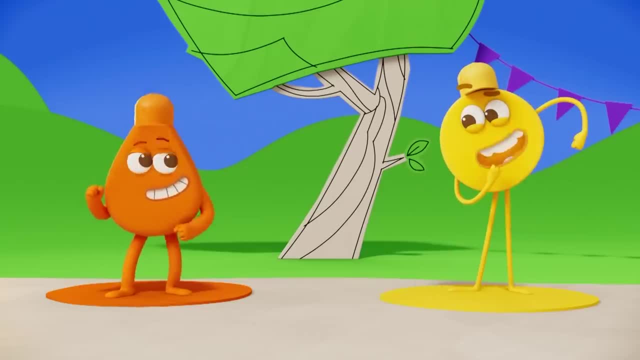 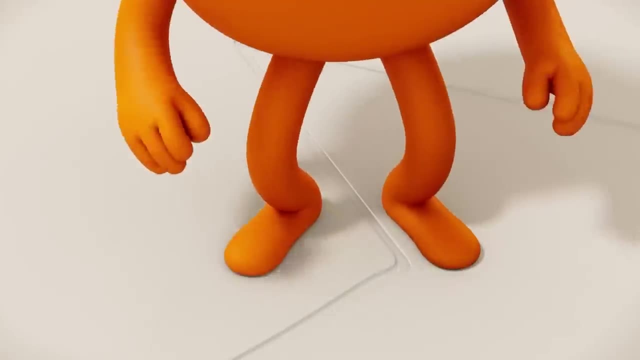 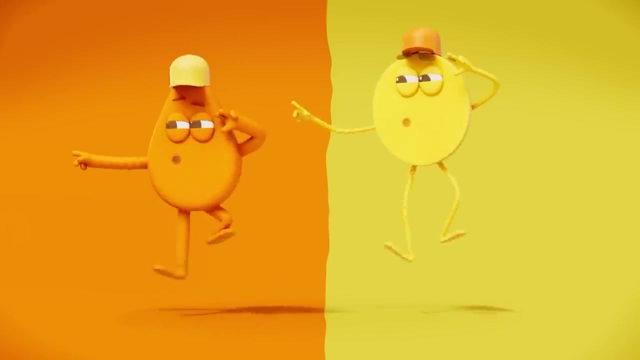 Who, who, who, Ooh, I'll pick the color next to me too. Orange, Hello, neighbor, Hello. They look good together too. That's because yellow And orange Are close color friends too. We're similar colors. 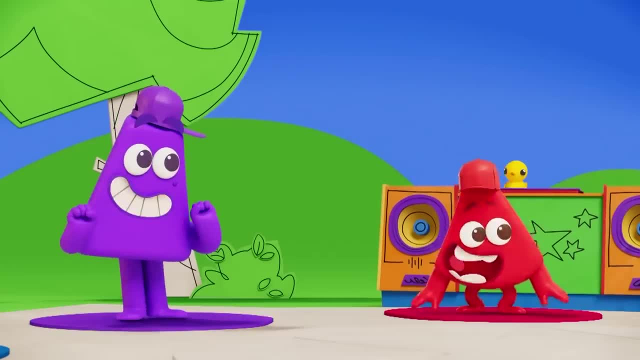 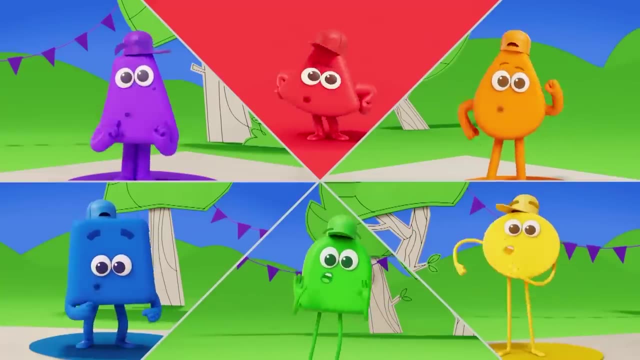 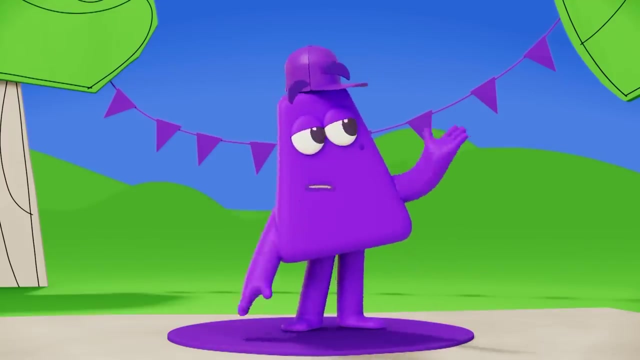 Ooh, Who's next? Me, me, me. Pick a partner up to you. Who's it gonna be? Who, who, who It's obviously going to be me. I'm next to red round the wheel And I have the best royal dance moves. 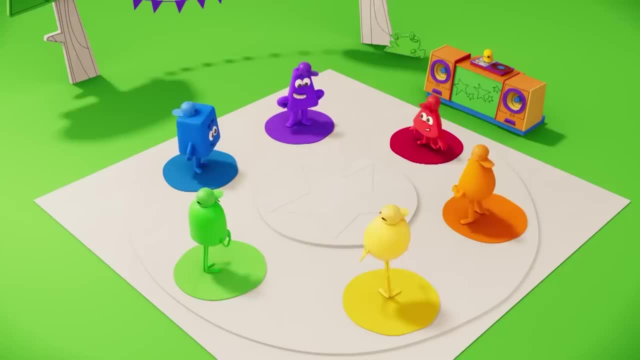 And I have the best royal dance moves. And I have the best royal dance moves. I Pick Grey, Oh, But red's not similar to green at all. But red's not similar to green at all. Green is on the other side of the color wheel. 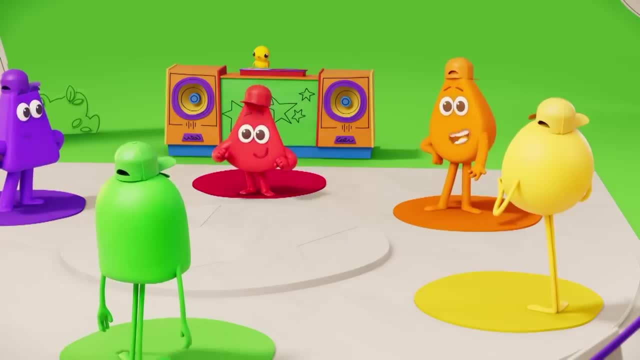 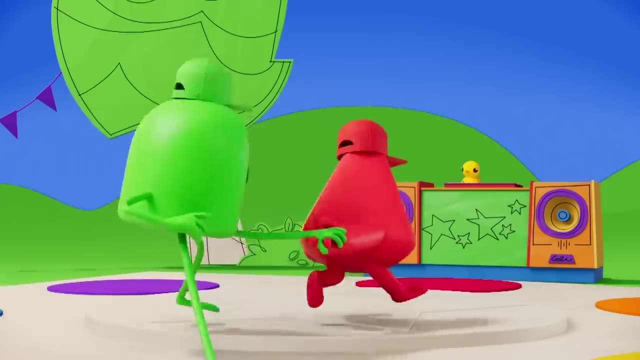 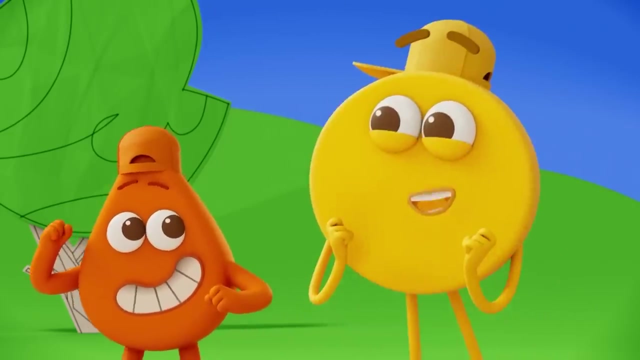 Green is on the other side of the color wheel, Your opposites. Green is opposite red. But that's who I want, Green, If you're sure. Wow, Their two colors really stand out. They look so bold together. They're opposites. 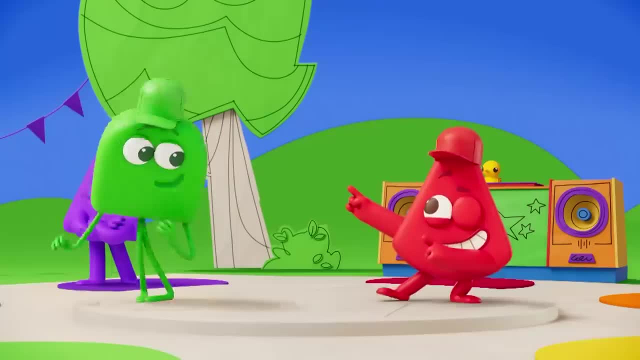 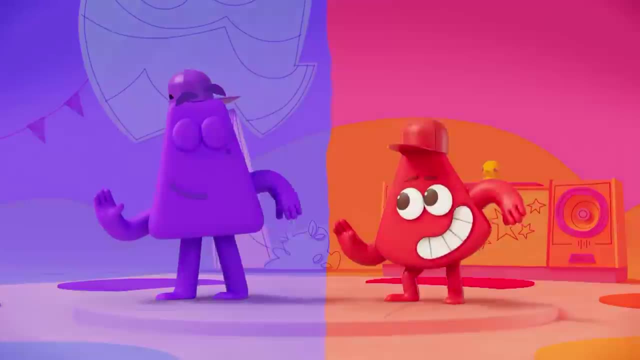 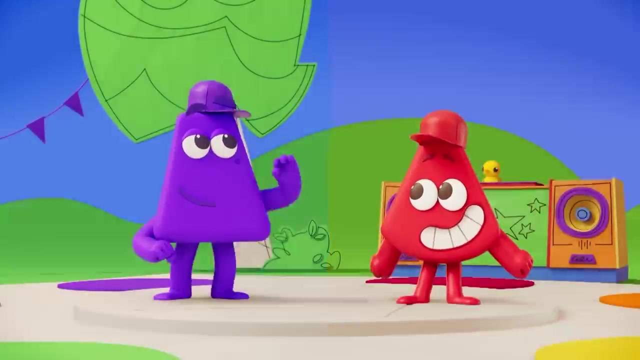 but they do go well together. Now I want to pick someone similar, But they do go well together. Purple About time, But they do go well together. But they do go well together, But they do go well together. Time for the next track. 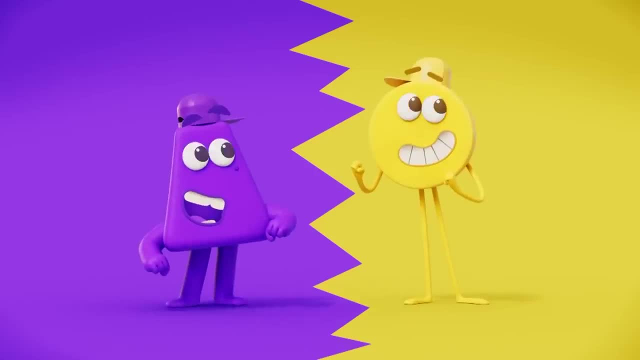 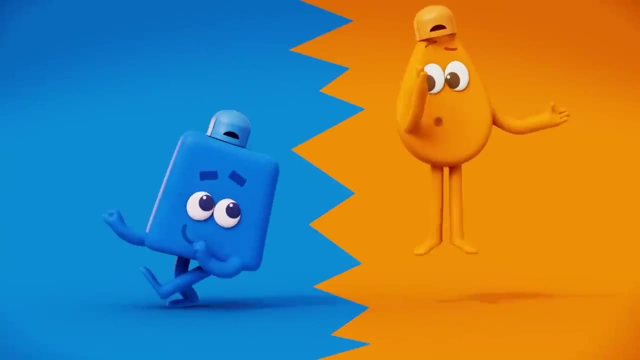 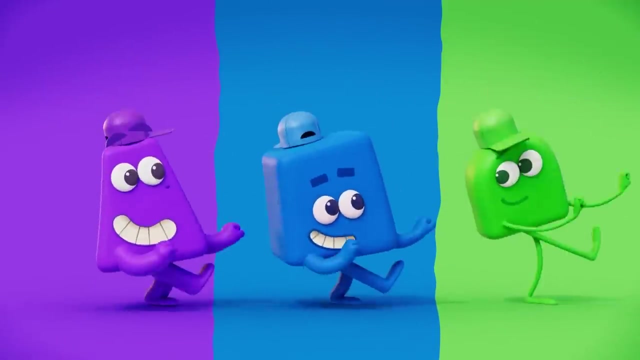 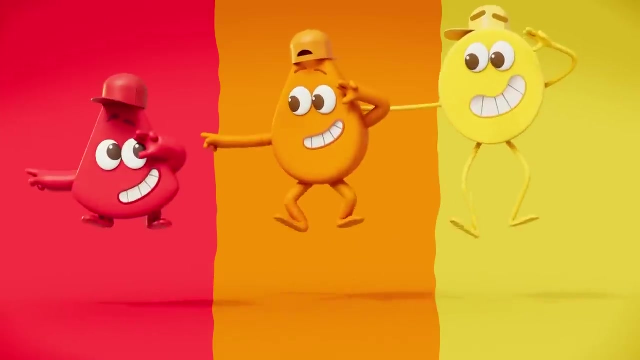 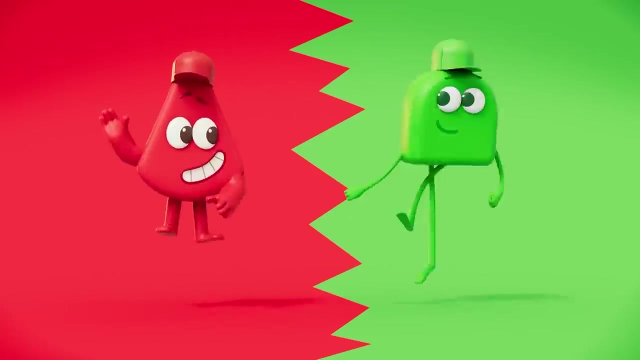 Opposite, Opposite, Opposite, Opposite, Opposite, Opposite. Let's go Similar, Yeah, Similar, Alright, Let's go. Let's go Opposite, Opposite, Opposite, Opposite, Opposite. 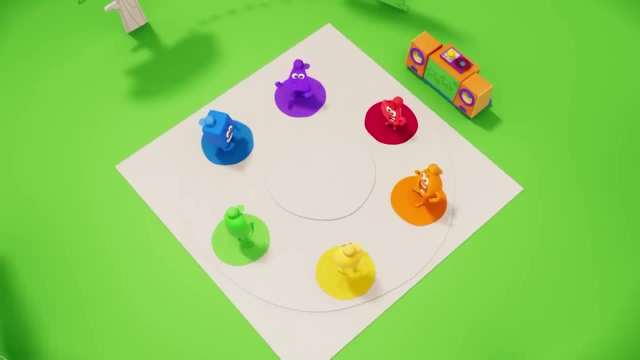 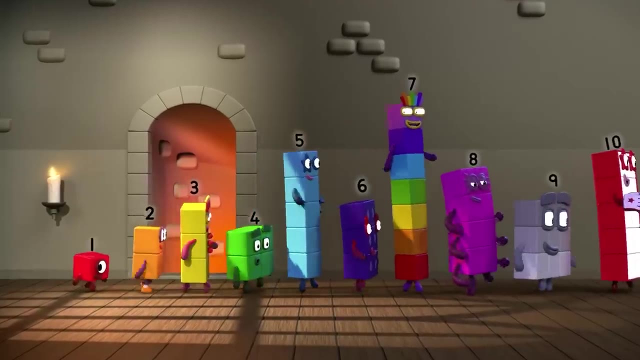 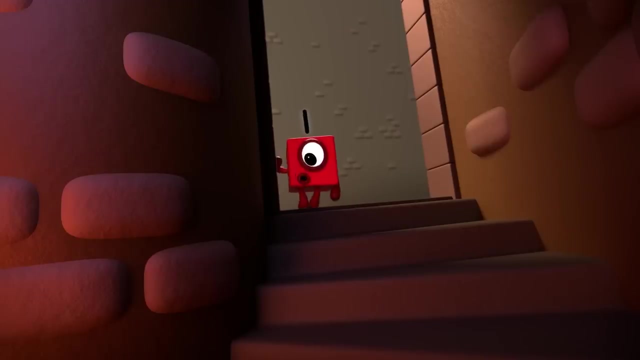 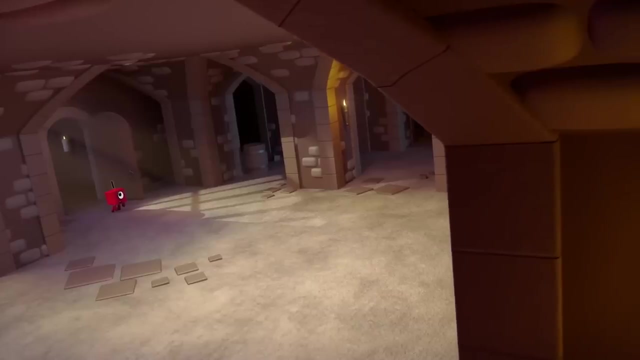 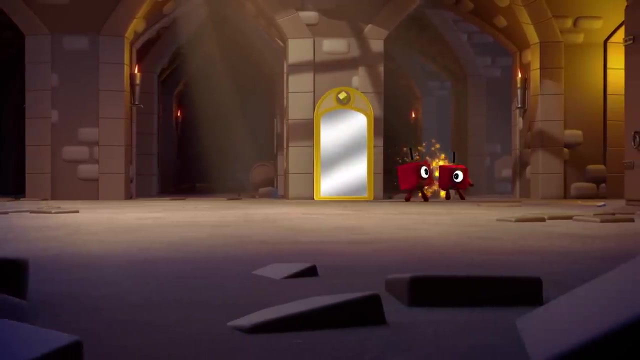 Similar and opposite: Opposite, Opposite. Aye, aye, Opposite, Opposite, Hey, yeah, Opposite, Upper, Ahh, yeah, Brett Europy. Opposite, Opposite, Opposite. Oh, it's a magic mirror. 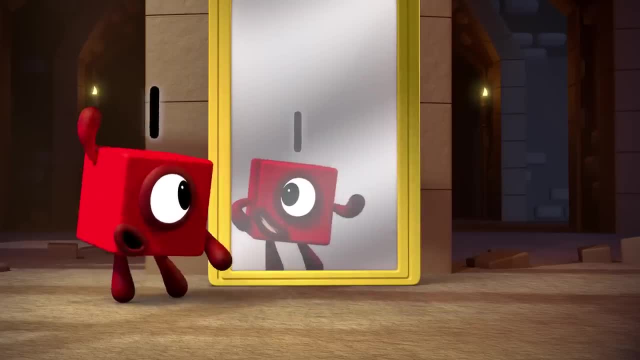 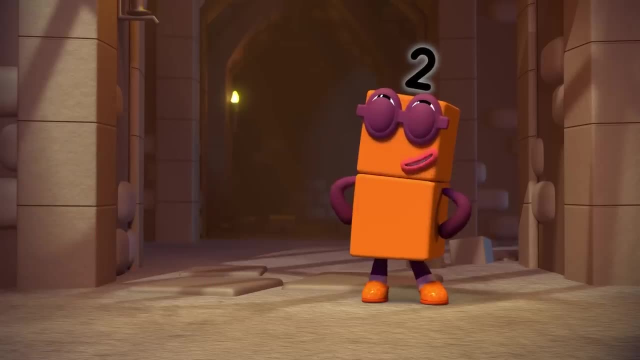 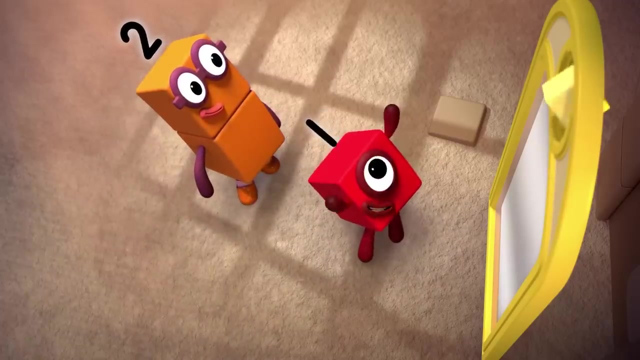 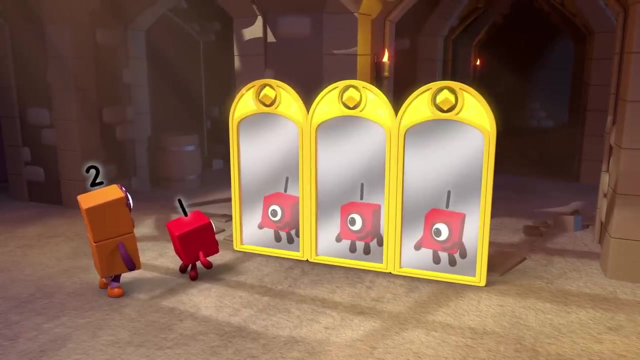 Oops, I've made two. lots of me. Making friends is fun. Oh, let's make three next. Oh, Mirror, Mirror, hear my plea. I wish you could make three of me. Your wish is my command. Wow, Three. lots of one. 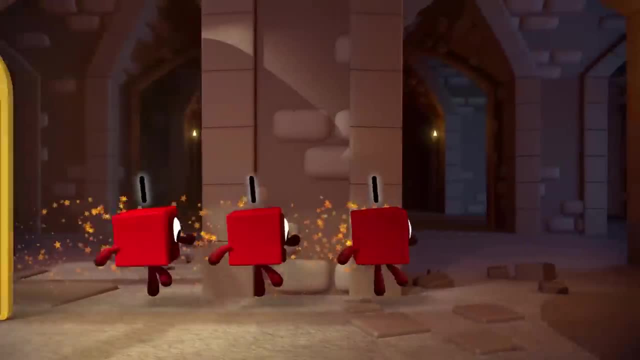 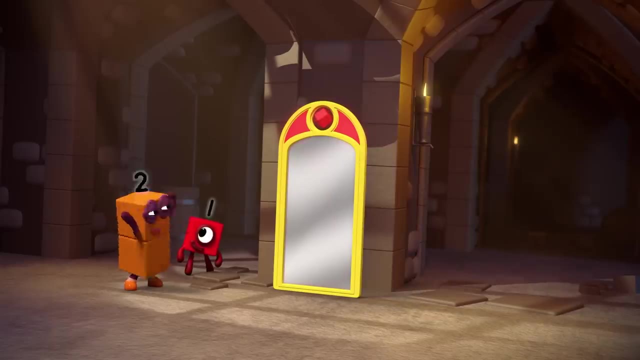 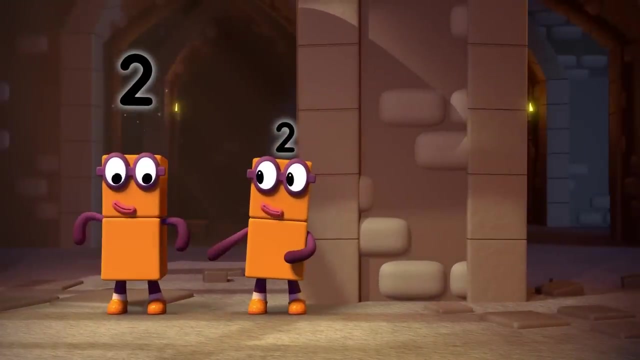 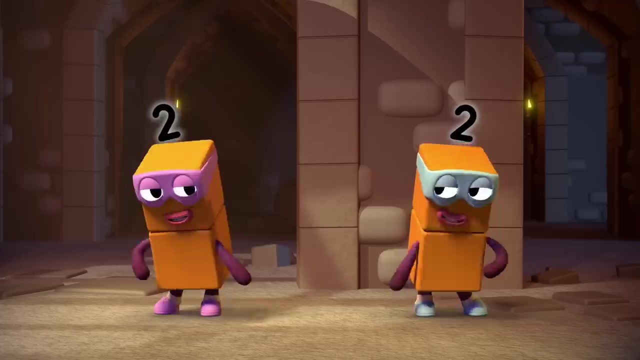 One plus one plus one equals three. Ooh, My turn, my turn. Two lots, please. Two lots of two. Two plus two equals four. I'm four. I'm two lots of two. The two lots of two. Two lots of two. 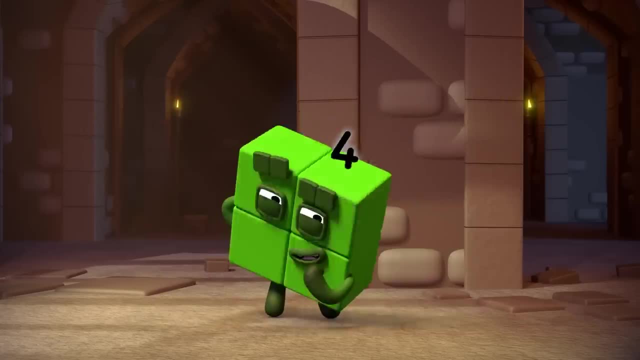 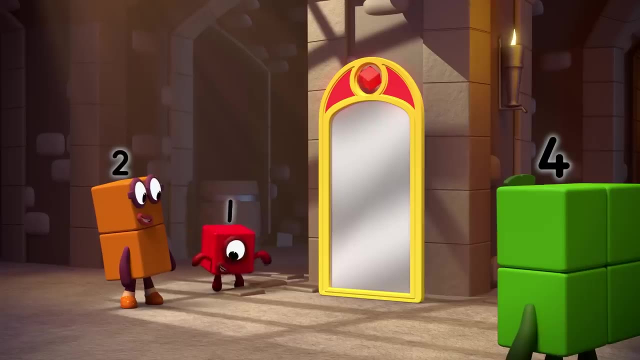 Two lots of two equals four. Two lots of two equals four. Two lots of two equals four. The magic mirror is even more magical than we thought. Oh, the others will want to see this. Keep an eye on it while I'm away. 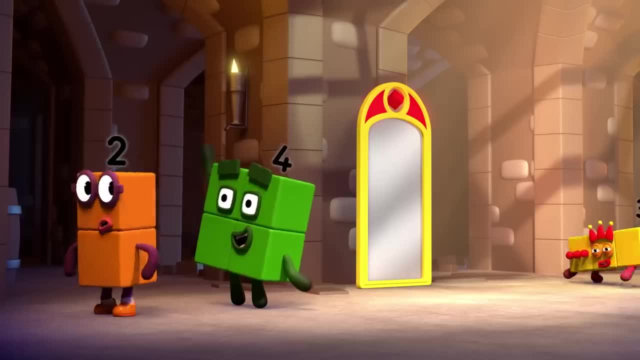 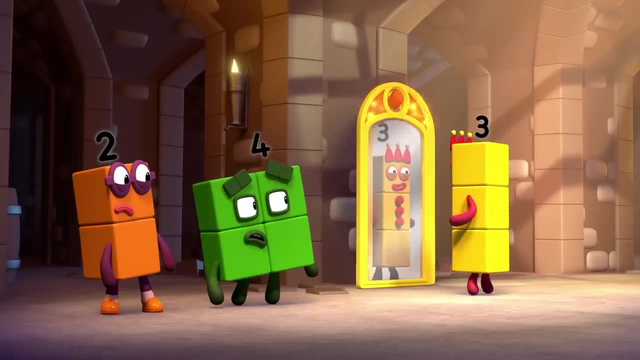 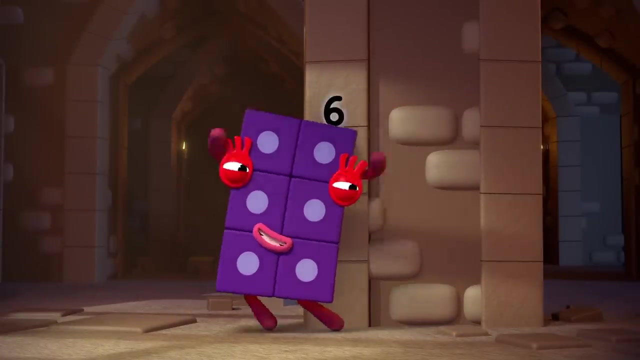 and don't mess around with it. Right, my turn. One said not to. Oh, go on, it's only fair. Two lots, please. Two lots of three is six. Number six is on the floor. Don't be shy, let's have some more. 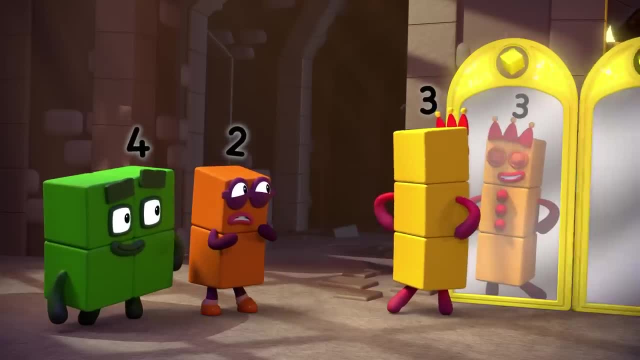 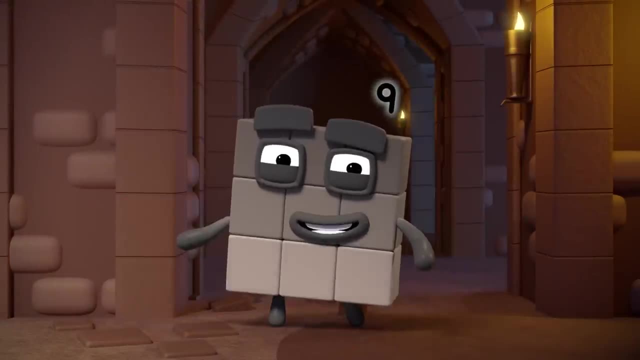 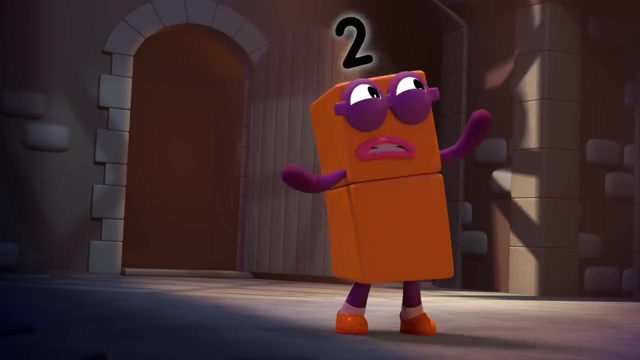 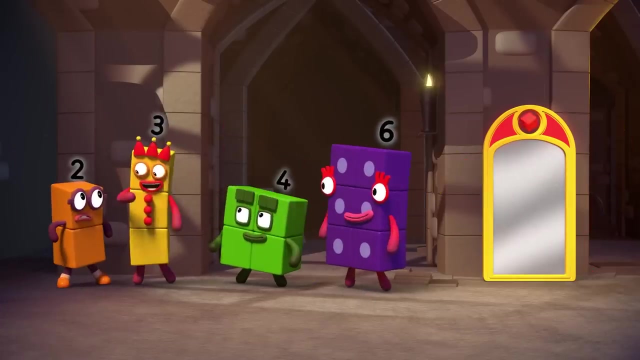 Good idea. Three lots, please. Three lots of three is nine. I'm three threes, see, Ha Yay, We should probably stop now. Look, there are so many of us here already. What would be surprised if she comes back and everyone's here? 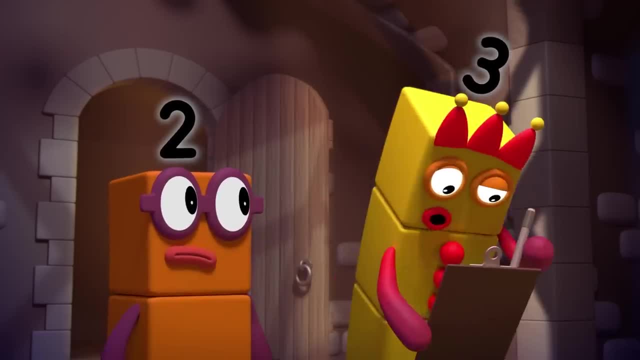 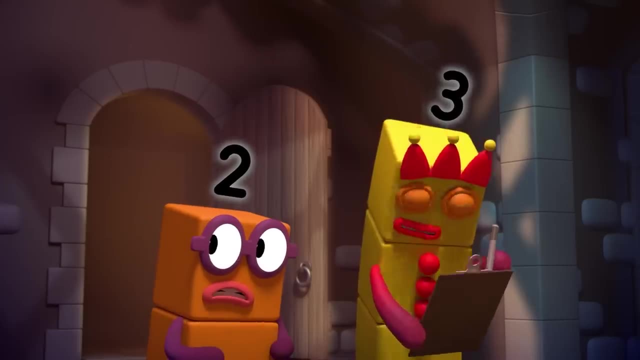 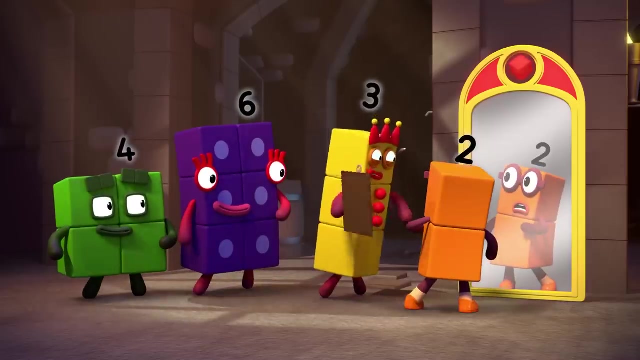 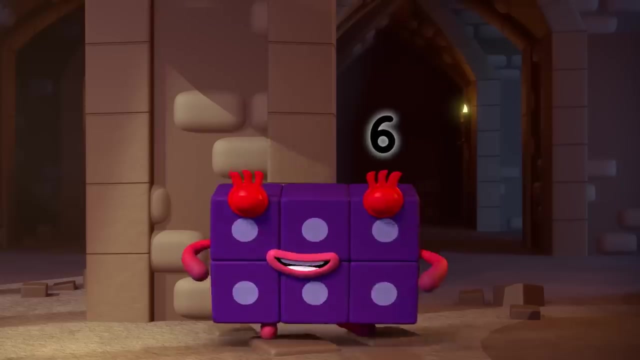 All right, then We've got two, three, four, then six. Oh no, We're missing five. How many lots of who is five? Hmm, Let's try you: Three lots, please. Three lots of two is six. 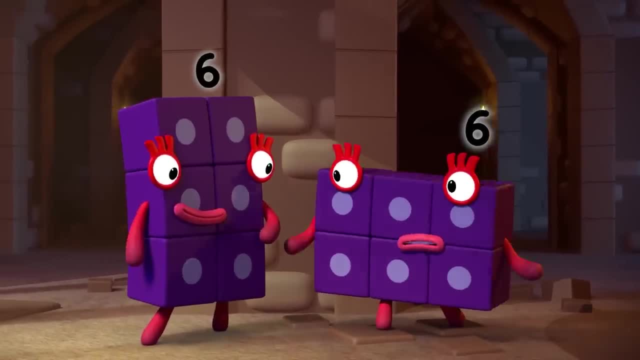 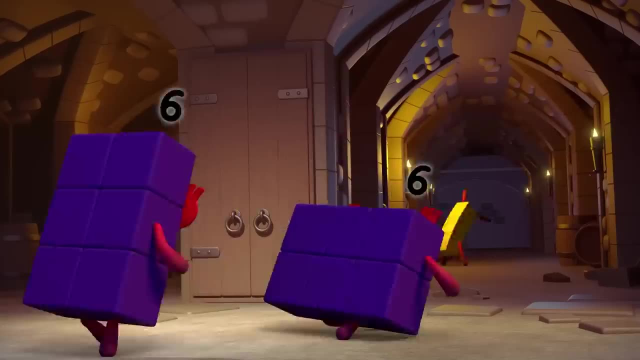 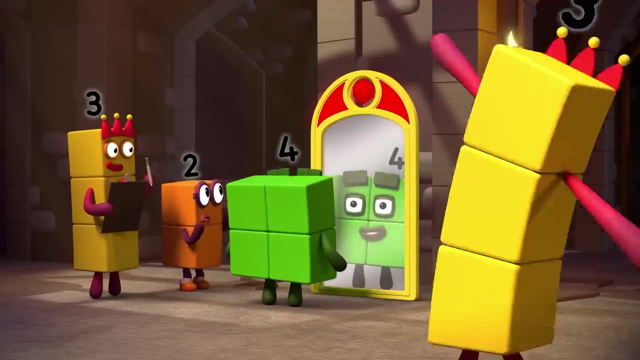 Number six is on the floor. Wait, have I said that before? Two lots of three, Three lots of two. Yay, I was hoping for a five. Maybe I can help. No Two lots, please. Two lots of four is eight. 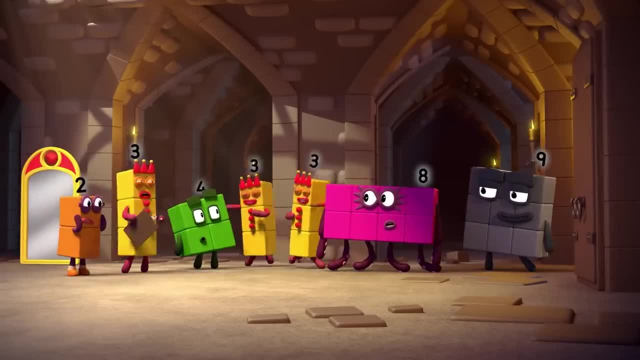 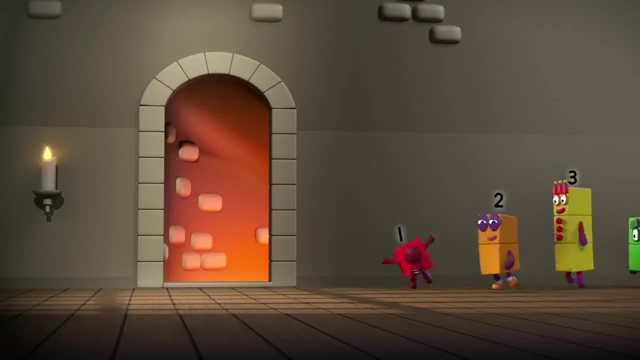 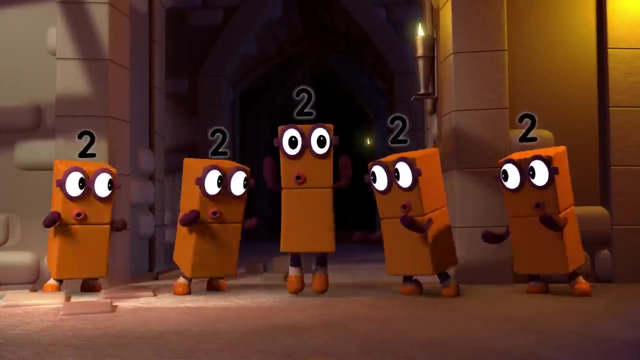 No, no, no. We need a five And we're missing seven and ten. Who wants to try next? Oh, It's a big surprise. Oh, Five, lots of two is ten. That's ten sorted. All we need now is five and seven. 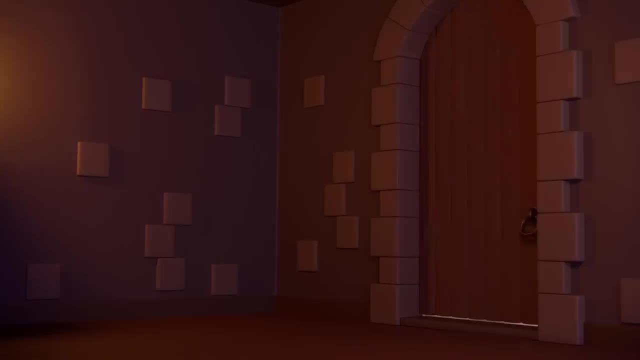 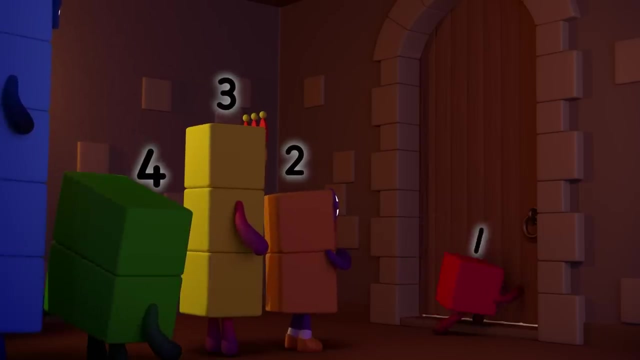 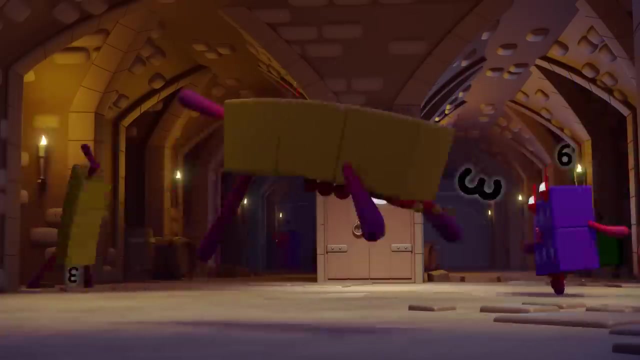 Next: Oh no, Get ready for a really big surprise. Huh, One's coming Hide. Why can't we make five and seven? Oh Oh There, Surprise. Oh Oh Oh, A magic mirror. Some big surprise. 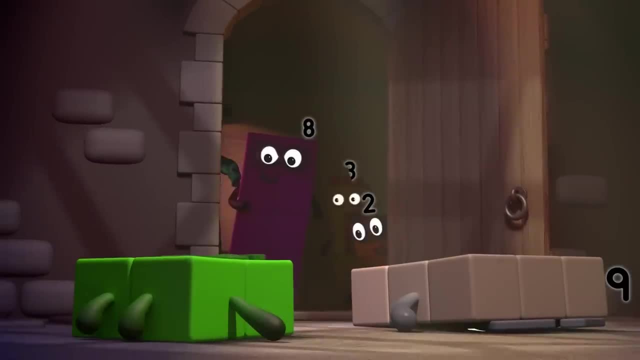 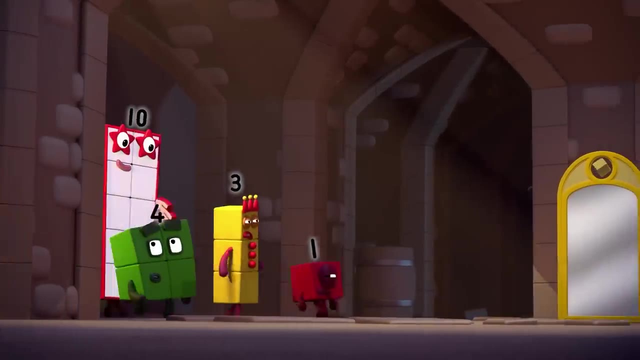 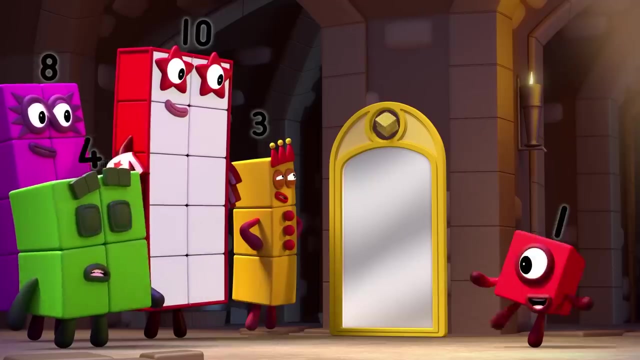 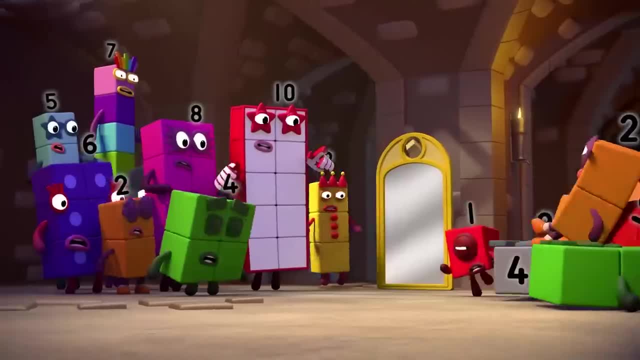 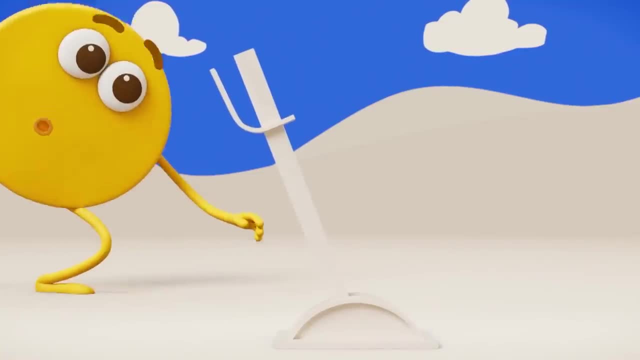 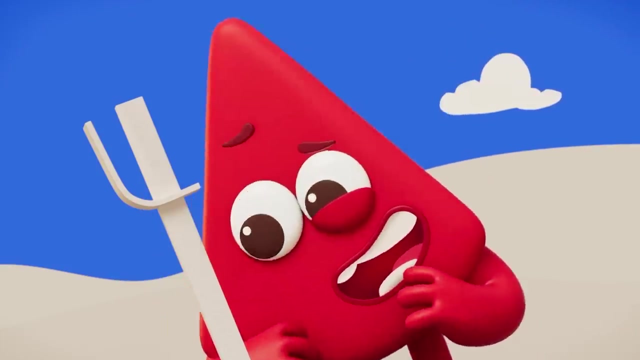 Now that would be a surprise. Oh, Oh, Surprise. Oh, What is it? Hm, I'm sure I've seen one before. It's a A. What do you think? Blip, I think it's a. 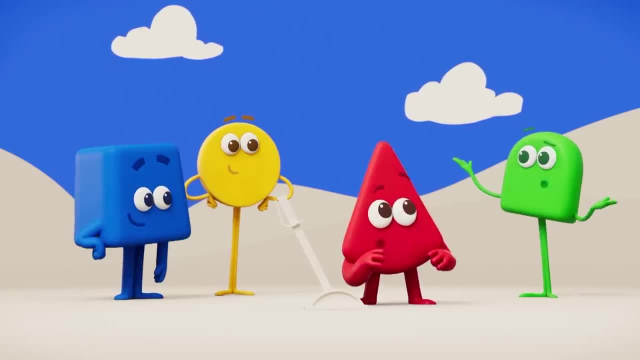 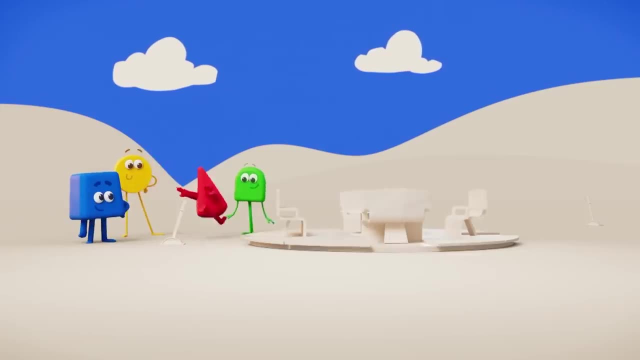 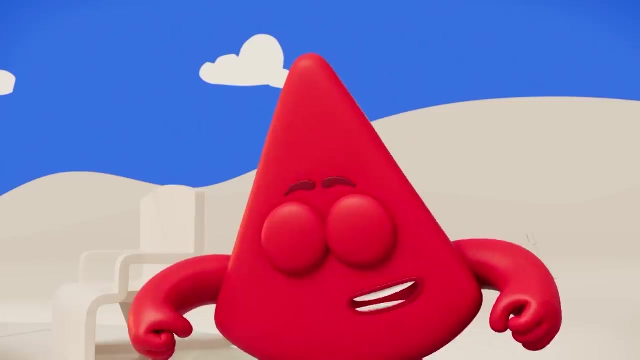 It's a lever, But what does it do? Let's find out. Exciting, But what is it? It's a round and roundabout. Round like a wheel With seats for four colours. It's a colour wheel. OK, everyone take a seat. 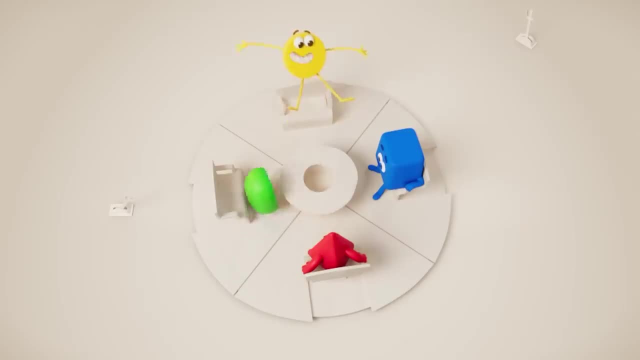 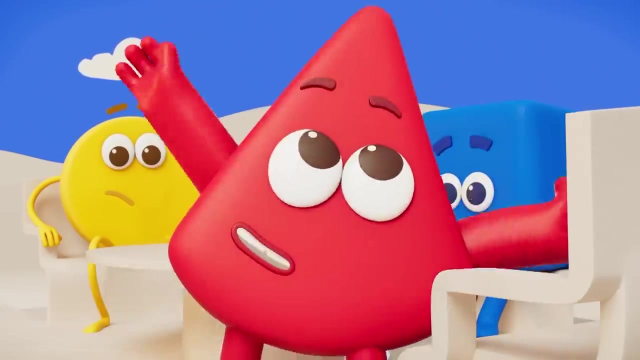 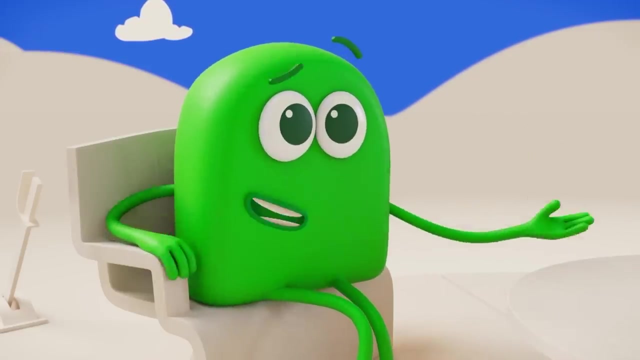 Red, blue, yellow, green. Oh, I thought it would spin round and round and round and round. Hmm, Maybe we're sitting in the wrong seats. Yes, What if the colour wheel only works when we're in the right order? 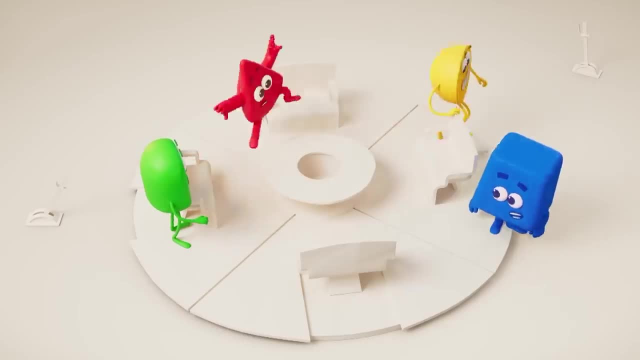 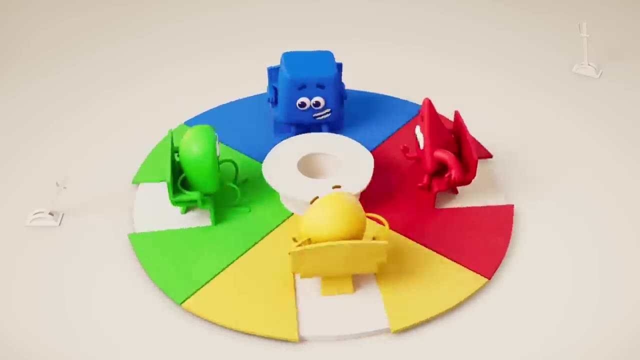 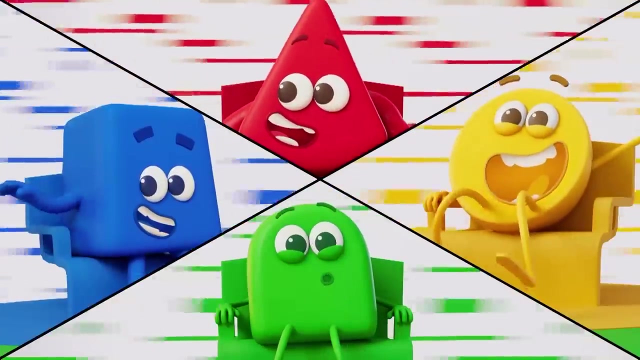 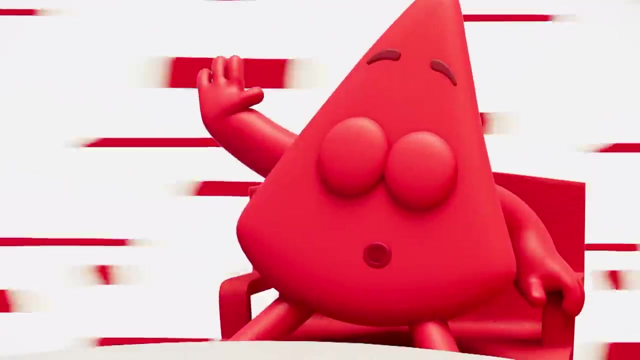 Yay, All change. Red, first Yellow, next Green And blue. It worked Four colours on a colour wheel. This makes me happy. Woohoo, Looks like someone's having fun. Red means stop. I see It's a round thing. 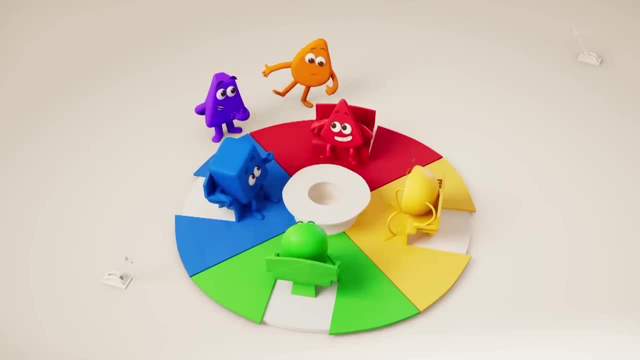 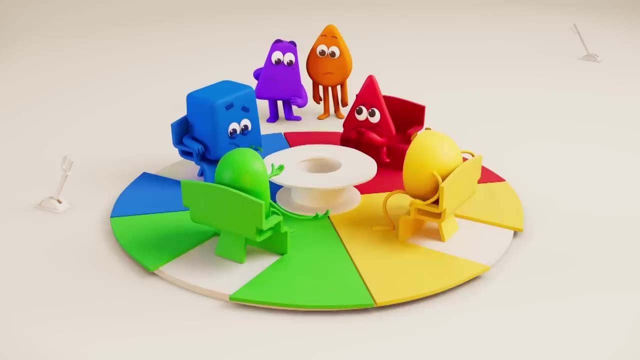 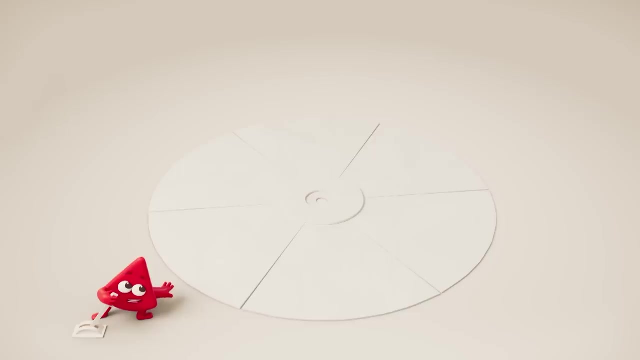 It's a colour wheel: Purple. Any room for us? I'm afraid not. Orange. There are only three. There are only four seats. Oh, Let's try pulling that lever. Here goes Whoa. Imagine that One, two, three, four, five, six. 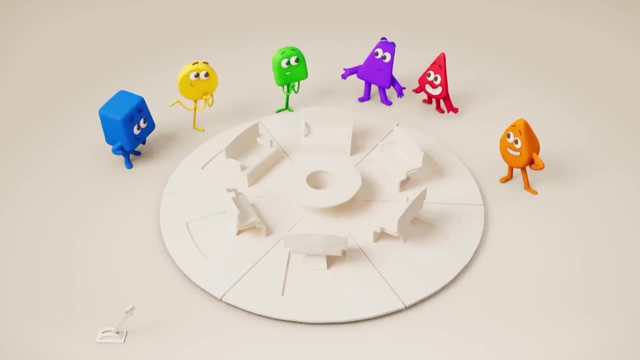 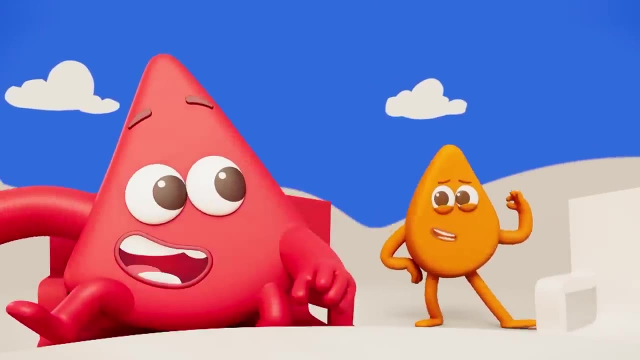 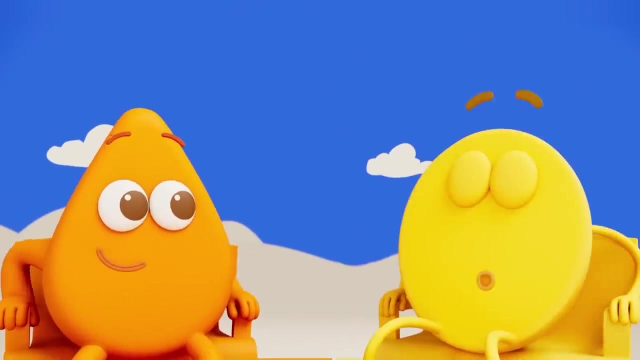 Six seats Room for us all, But we have to sit in the right order. Red goes first. again, Orange is a bit red, so I think it's me. next Woo, And orange is a bit yellow, so now it's me. 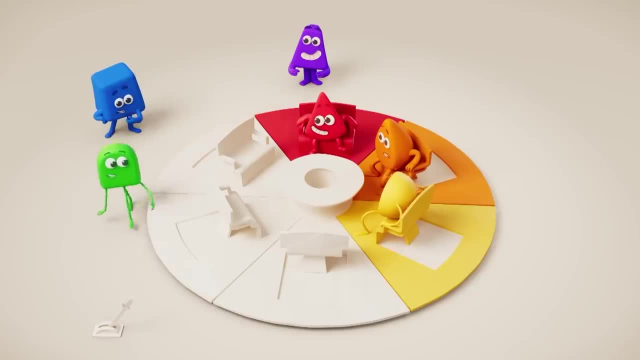 Now who goes next? Green is close to yellow, so naturally I sit here, And green has blue in it, so this seat is for me. We've saved the best till last. Purple goes in between blue and red. Six colours on a colour wheel. 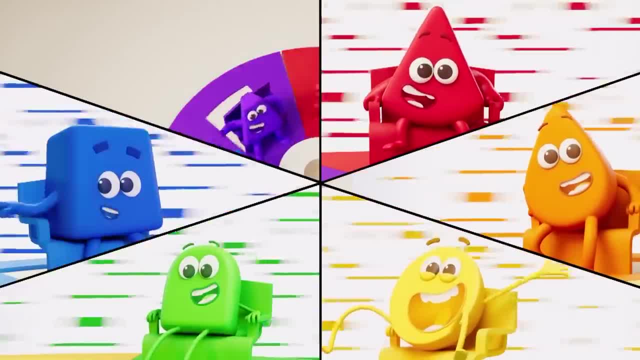 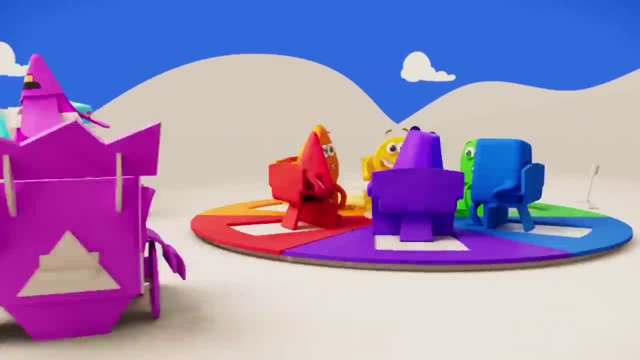 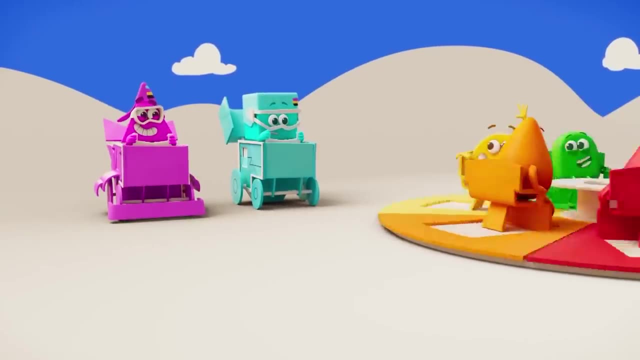 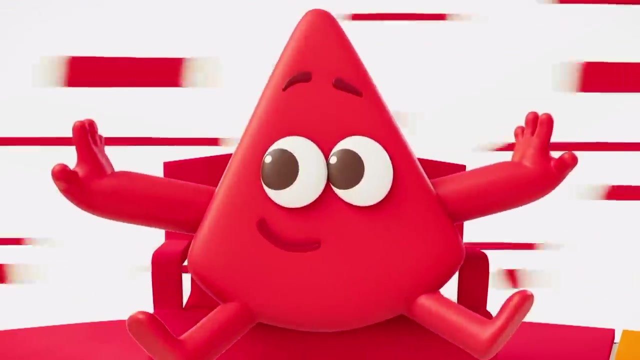 Red, Orange, Yellow, Green, Blue, Purple. Wow, This looks brilliant. Yay, It's cyan and magenta. My printing crew. We love a spin Room for two more. Red means stop, We're going to need a bigger wheel. 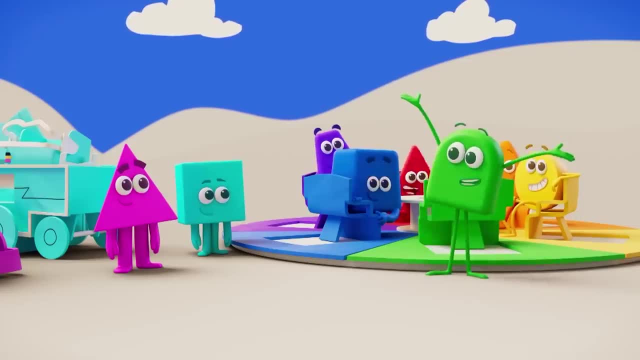 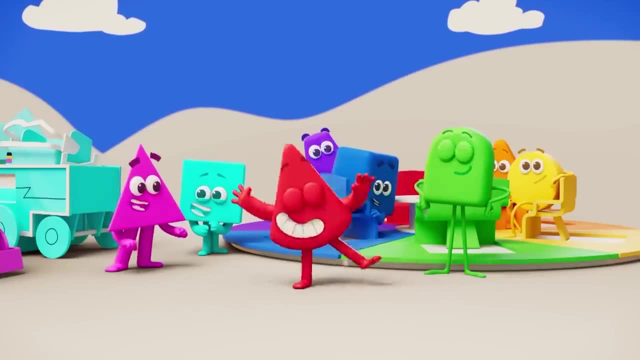 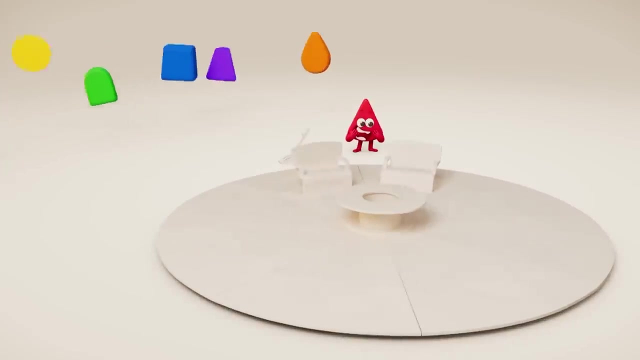 An eight-colour wheel. Look Who wants to pull the next lever. I do, Wow, We have to find the right places for magenta and cyan. Well, I look a bit like Blue, so I should go. Hmm, Yeah. 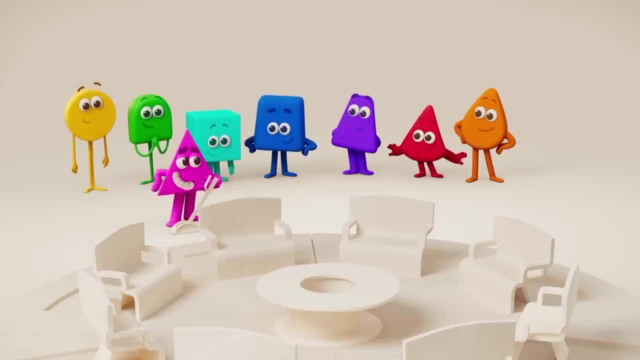 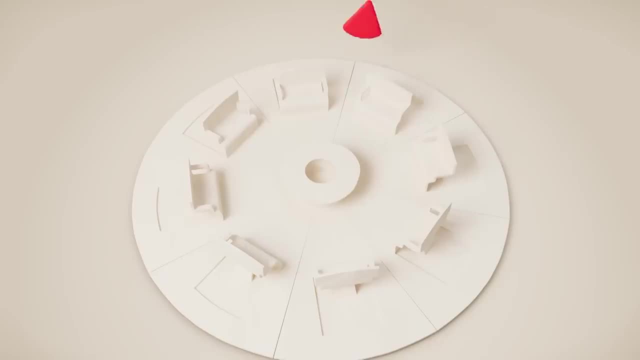 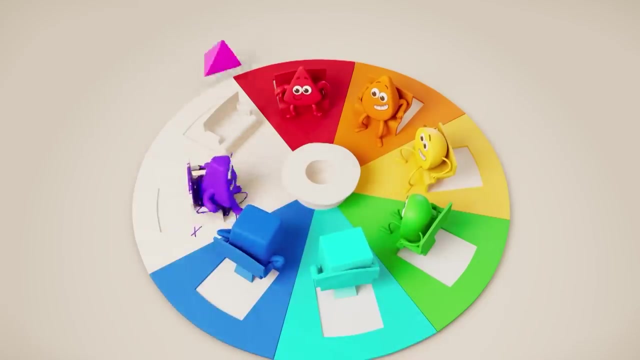 Yeah, And I look a bit red, so I should go Here. Oh, yes, OK, everyone take your seats. Red, Orange, Yellow, Green, Cyan, Blue, Purple, Magenta: Eight colors on a color wheel. 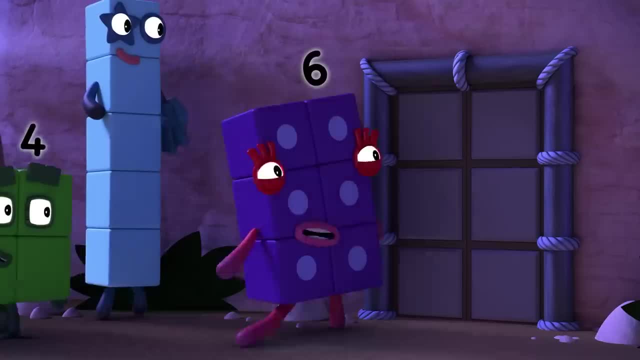 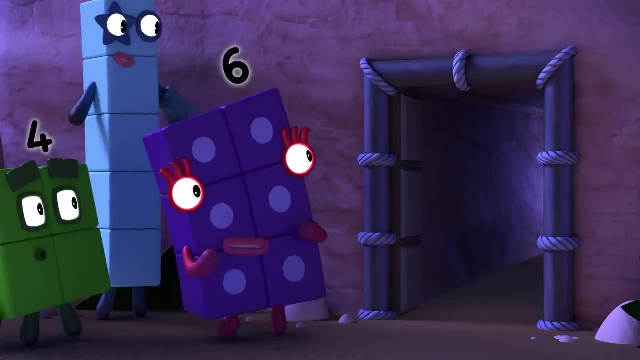 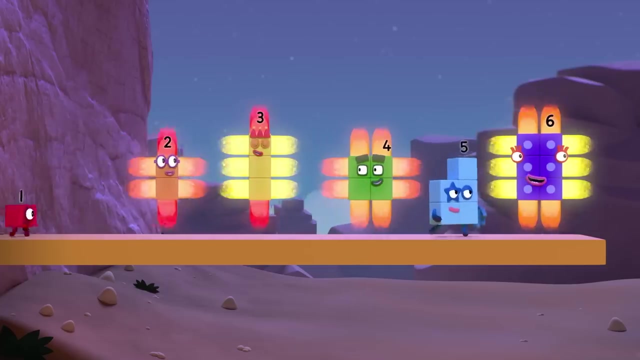 Here it is right where Twelve told us The doors to Ray Canyon. Hmm, I wonder why it's called Oh Oh, Ray Canyon. Oh Oh, Rectangle rays, Oh Hooray. Twelve said if one of you can get to the top. 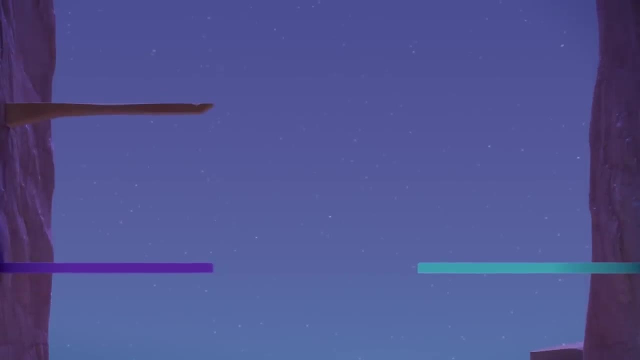 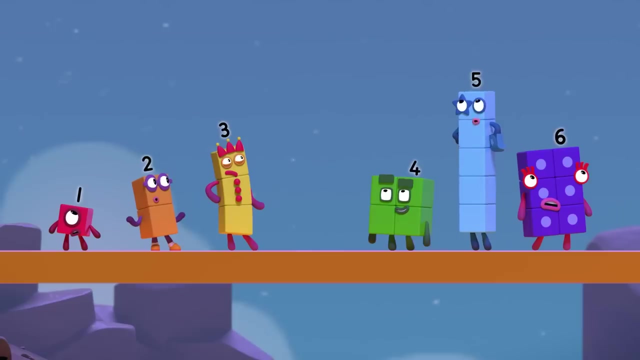 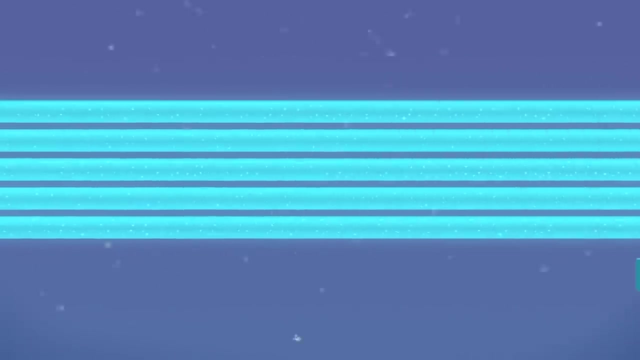 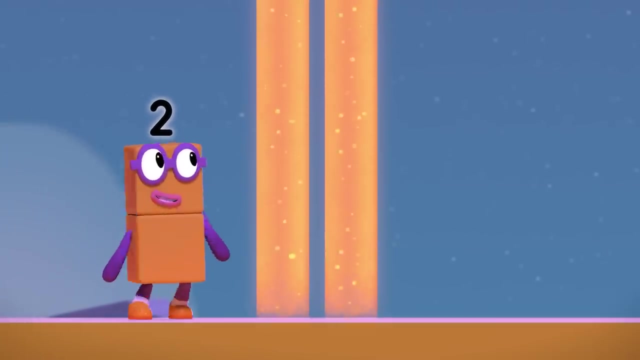 you'll find a big surprise. Oh, Oh, Yes, we knew, But how It's too far to jump. Ride the rays. Ooh, How do we ride them? These are two rays, so maybe Whoa Whee. 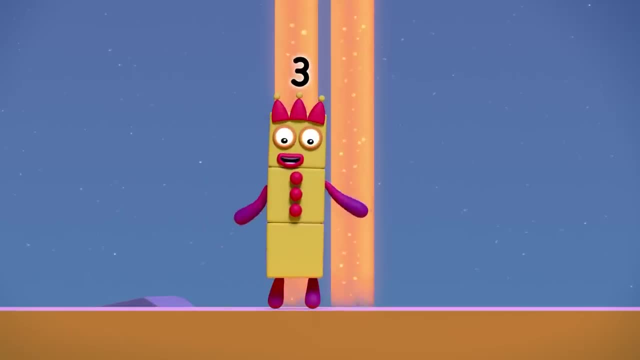 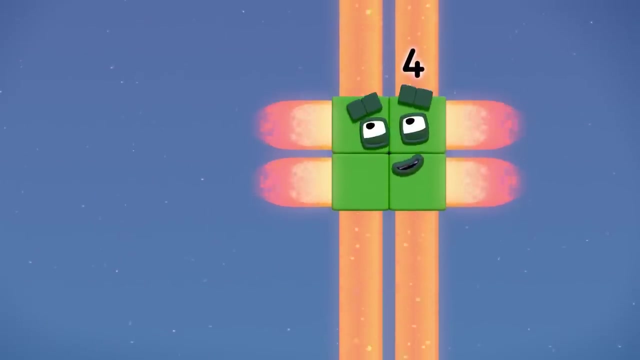 Come up, It's fun. Ooh, Oh, Oh. That's no use. I can't make a rectangle that's two blocks wide. No, but I can. I'm a two-by-two square. Whee-hee-hee-hee-hee-hee-hee-hee-hee-hee-hee. 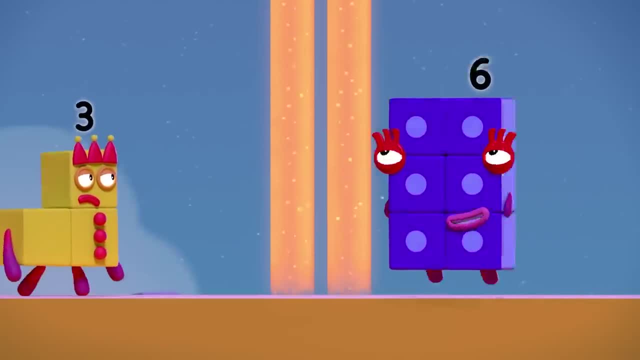 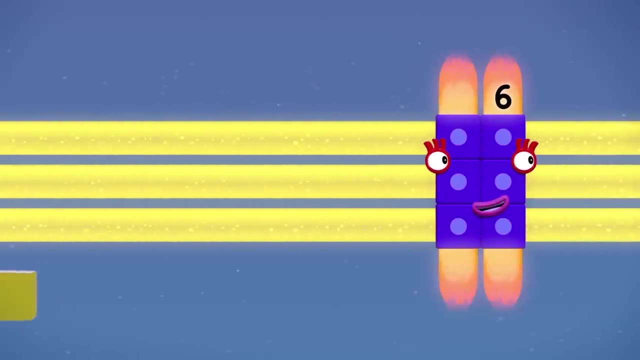 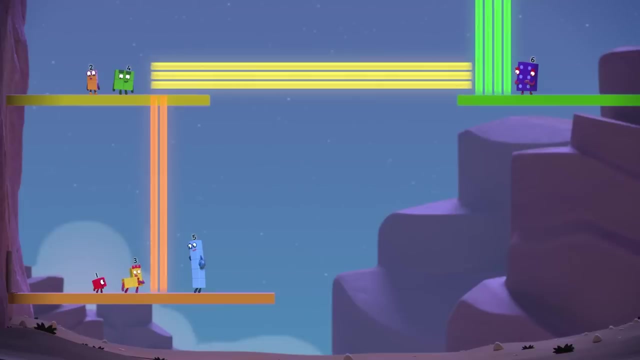 If you think that ride is smooth, wait till you check out this move. Ooh, Wow, I'm two, lots of three. I've got two rays and three rays. Ha-ha Aw, I've got three rays too, you know. 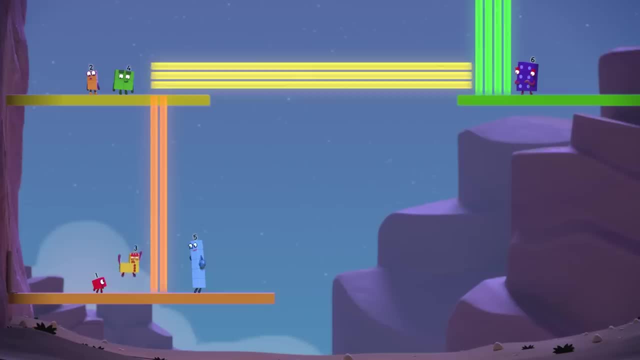 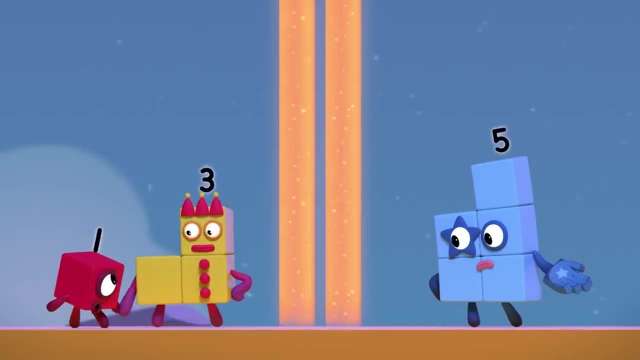 I could ride across, just like six, if I could get up there. Hmm, Odd numbers like us just can't make a rectangle that's two blocks wide. Twelve said only one of us had to get to the top. remember, We can all work together to find a way. 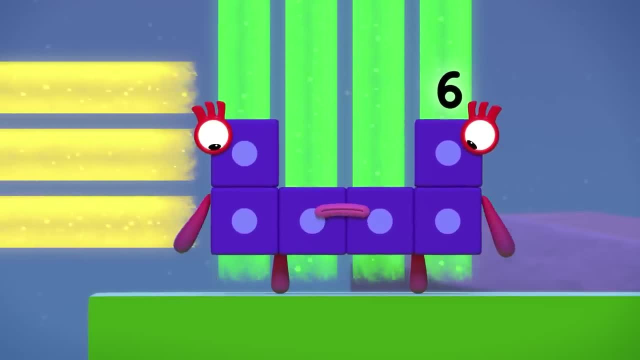 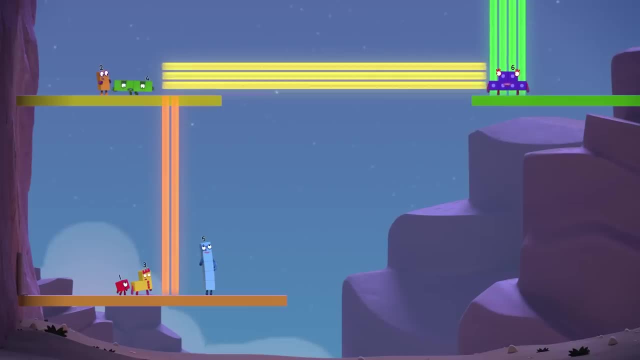 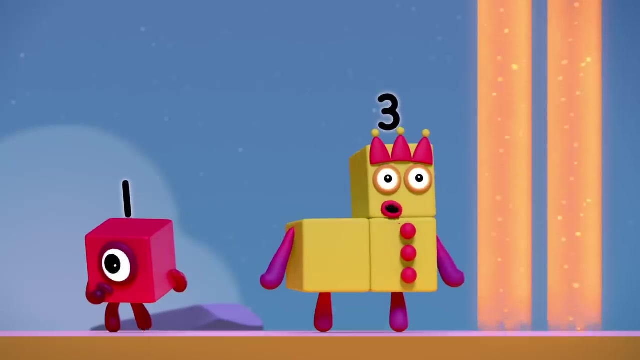 I don't see how We're out of luck. I can't make four blocks wide. I'm stuck. I can, I can, But I'm stuck here. We're all stuck. Twelve must have made a mistake. Wait a moment. 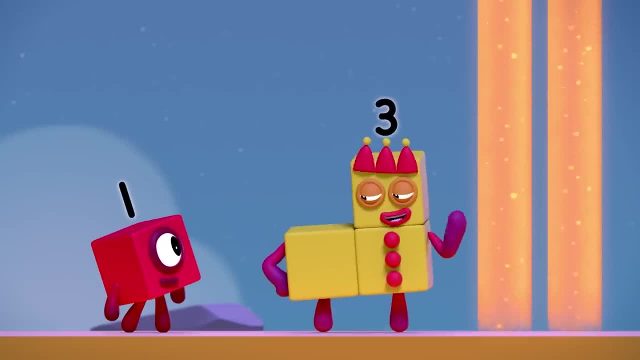 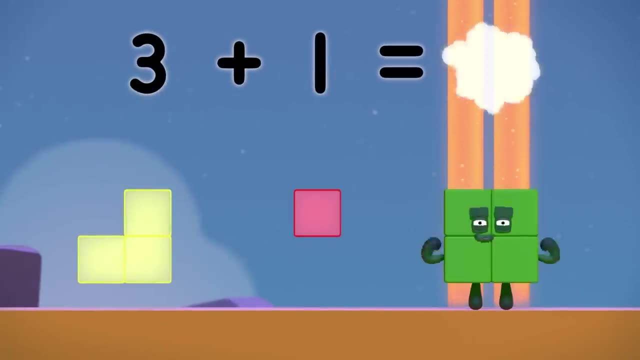 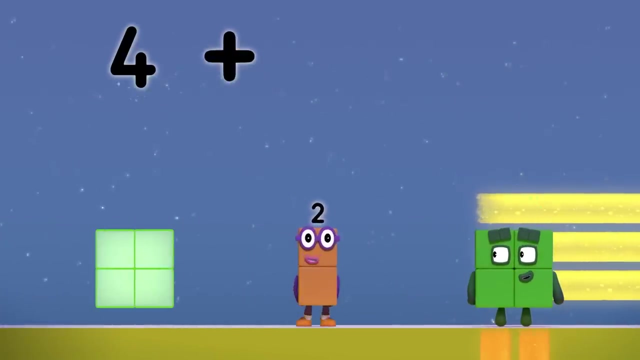 Maybe there's more than one way to solve this problem. Sometimes you need to think round corners: Three plus one equals Four. Ooh, Ooh, Ooh. Four plus two equals Six. I'm so glad I can reach this shelf. 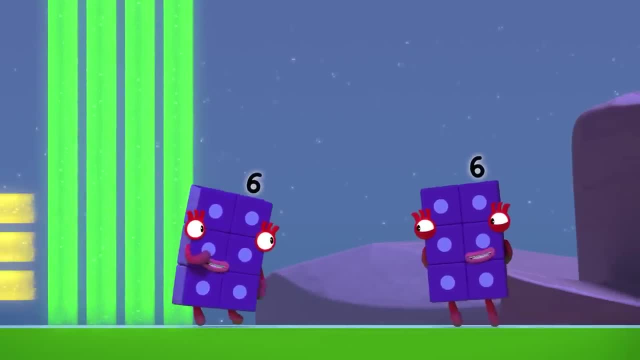 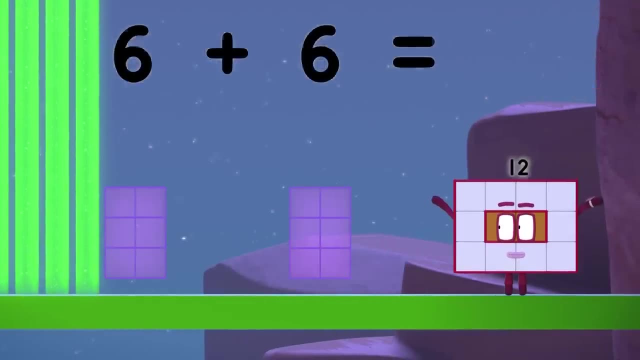 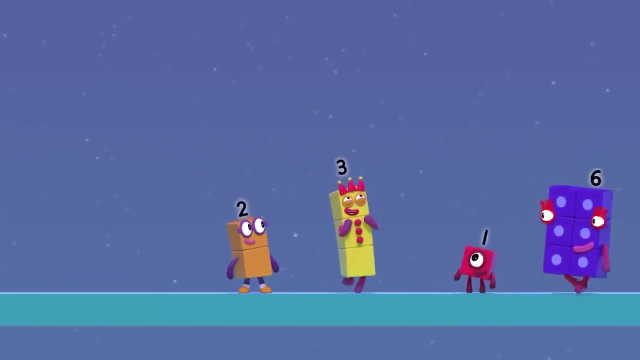 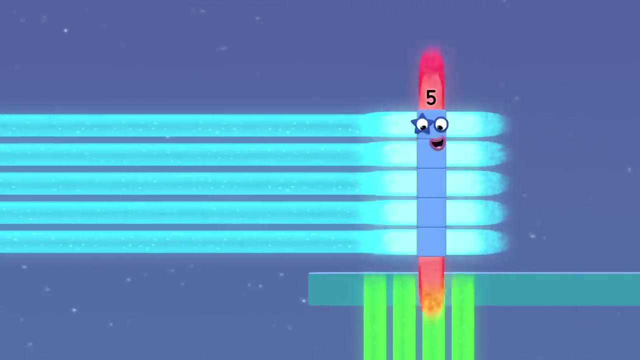 I'm so glad I can reach this shelf, So happy I'm beside myself. Six plus six equals Twelve. Oh well done. Who came up with this idea? Me, me, me. Three plus two equals Five, Hooray. 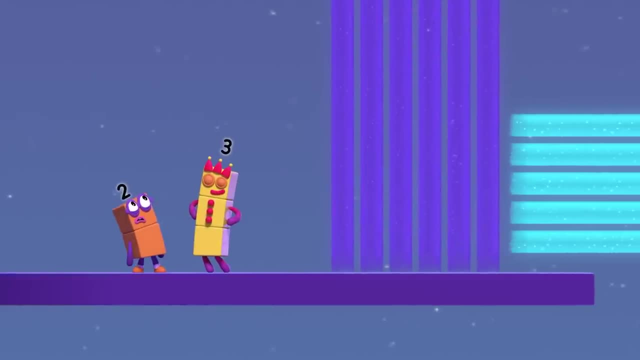 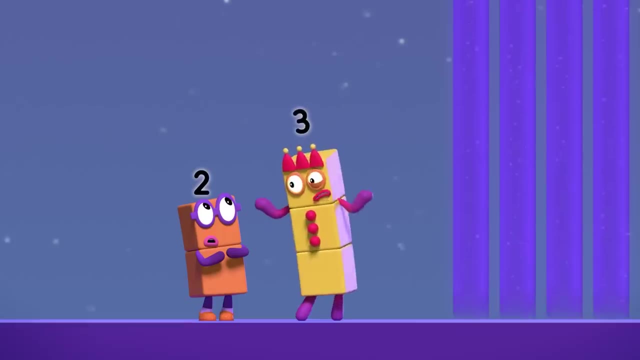 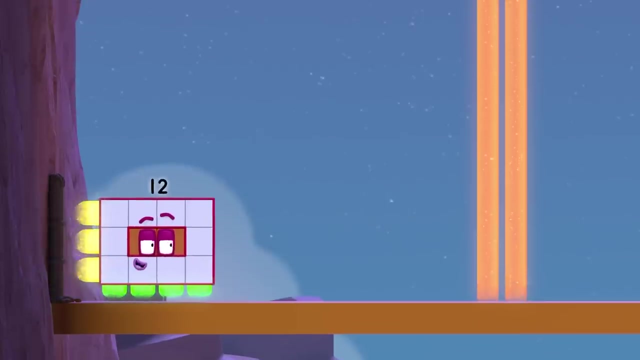 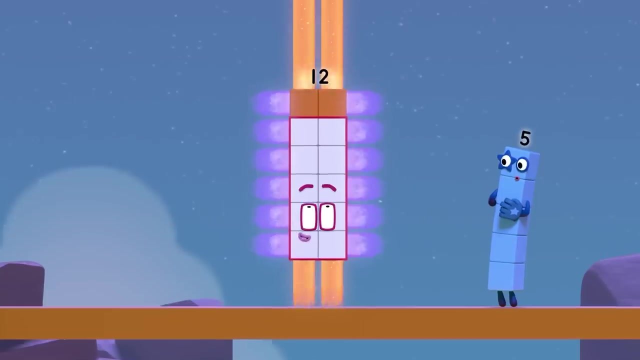 Yeah, Hooray, Yeah, Um, but how do we get up there? We can't make anything. that's six blocks wide. We've only got five blocks between us. Hello, my friends, Twelve Switch. Congratulations on getting so far. 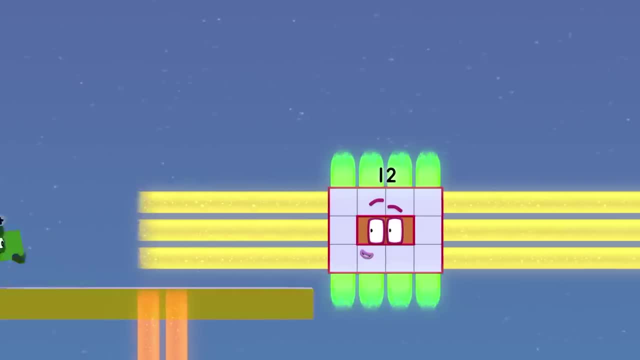 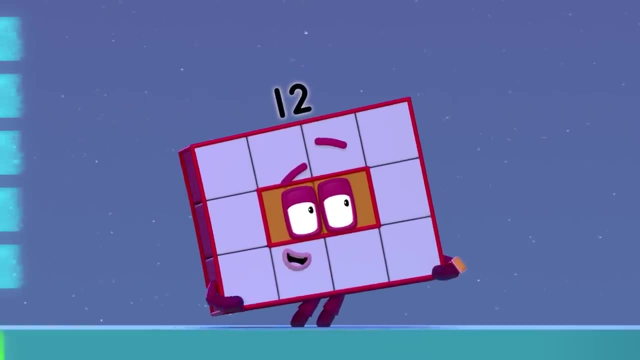 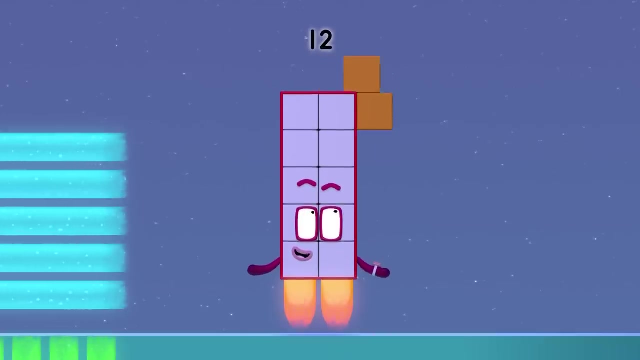 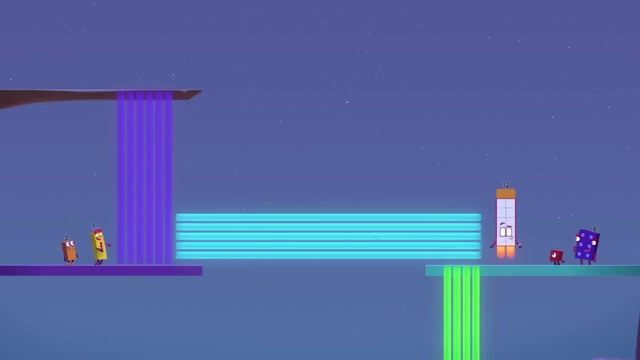 Switch. By working together, you've nearly reached the top. What a super rectangle. But not even I can make every size of rectangle. I can't make a rectangle that's five blocks tall, See, But, like you said, Three. sometimes there's more than one way to solve a problem. 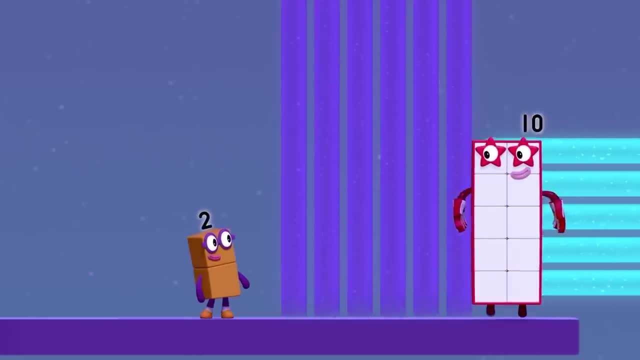 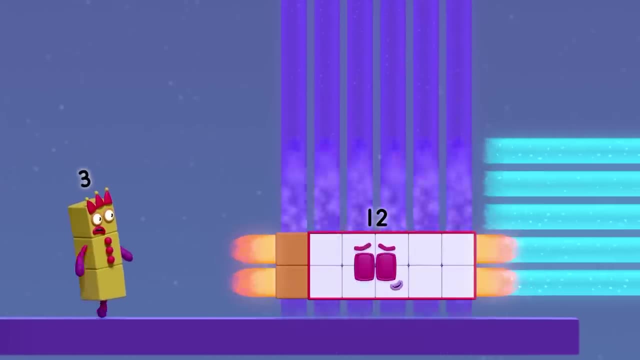 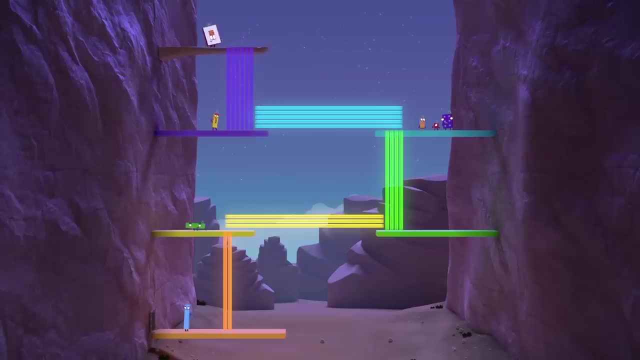 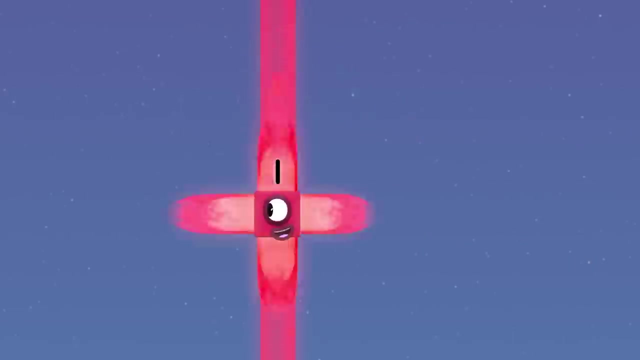 Twelve is ten plus two. Ten plus two equals twelve Ten. I'll drop you a line. What does that mean? Whoa, Woo-hoo-hoo, Whee, Whoo, Hee-hee-hee-hee-hee. 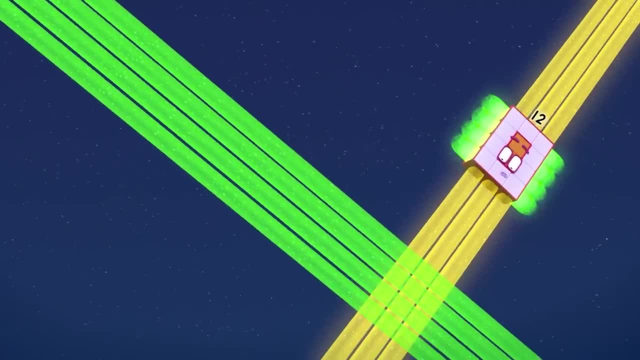 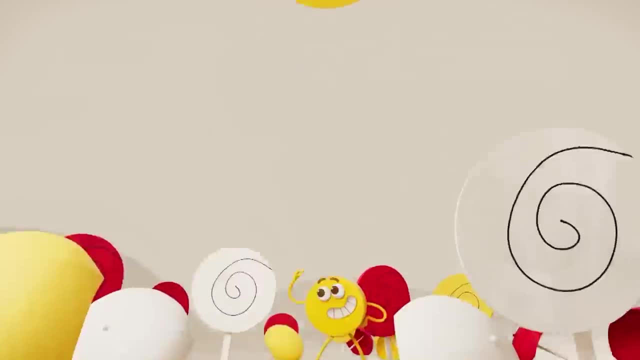 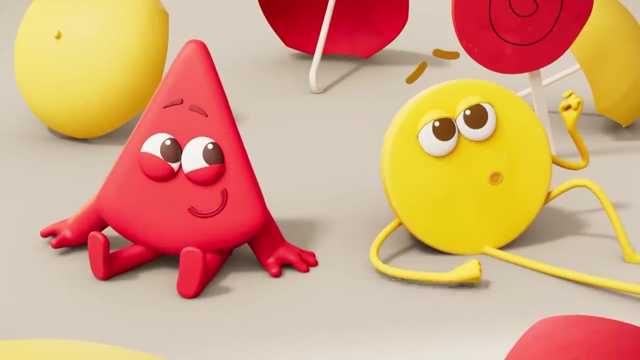 Whoo-hoo-hoo, Welcome to the racetrack. What do you think? I love it. Whoo-hoo-hoo. Red, Yellow, Red, Yellow, Red. Ha, Exciting Phew Colouring makes me so happy. 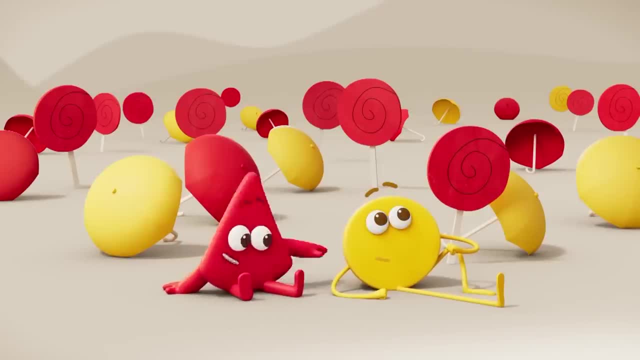 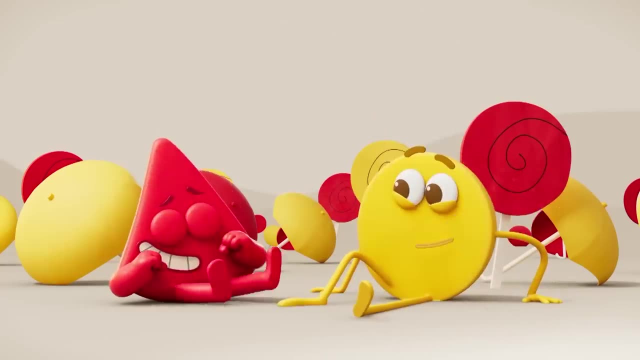 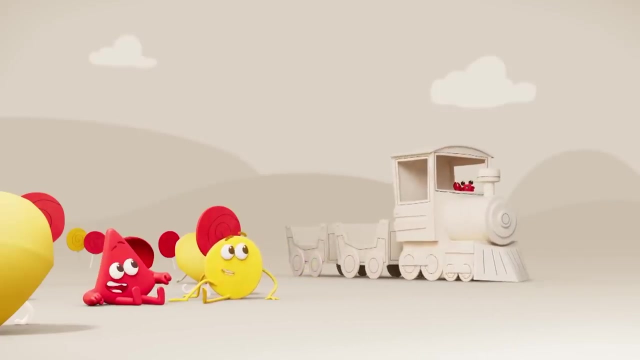 My red things and your yellow things are all modelled up. Ooh, Let's sort them into yellow things And red things. A sorting game. But where are we going to put the things we've sorted? Ooh, A train with two wagons. 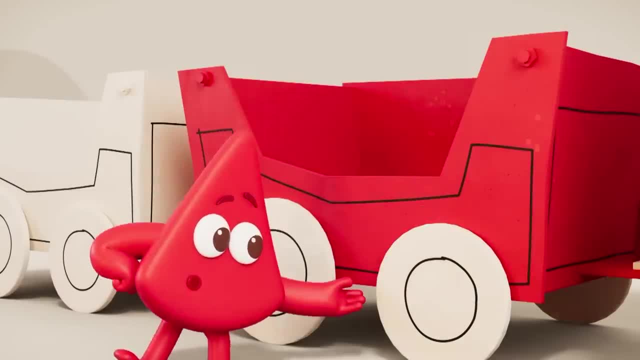 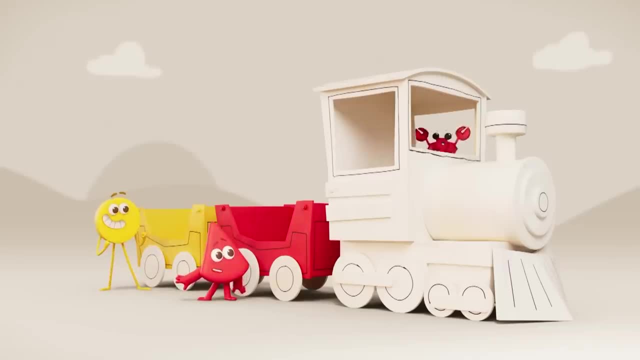 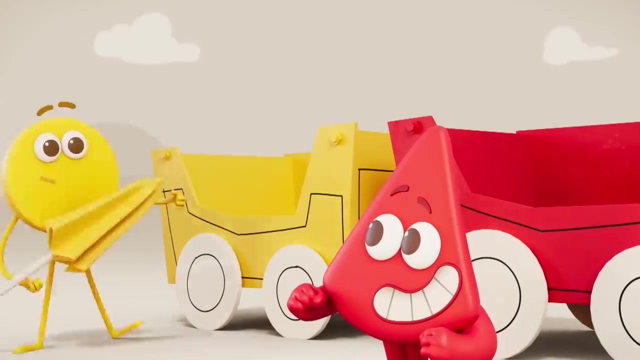 That will help us All. the red things can go in the red wagon And the yellow things can go in the yellow one. Oh-ho-ho, It's the sorting express. This lolly is red And this umbrella is yellow. 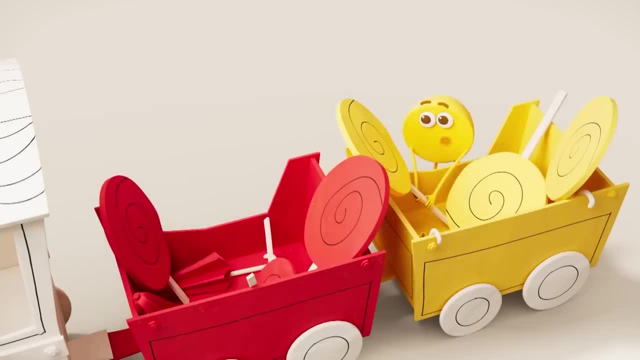 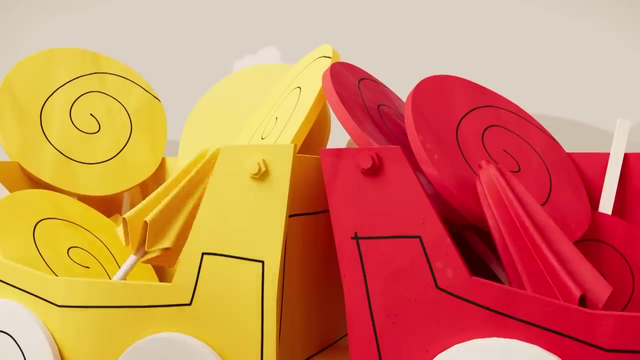 Ha-ha-ha. Red lolly, Yellow lolly, Red lolly, Lello-yolly. I mean yellow lolly, Red frolly, Yellow frolly. Ha, We did it. Everything's sorted into two colours. 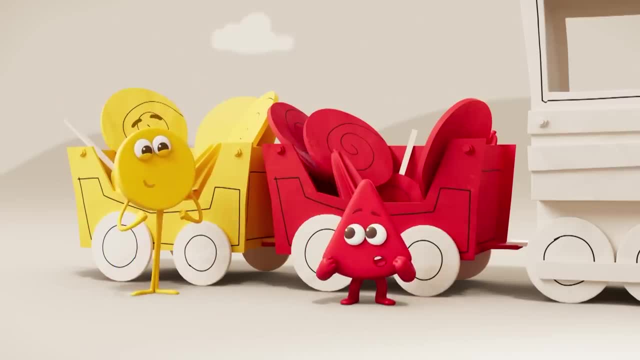 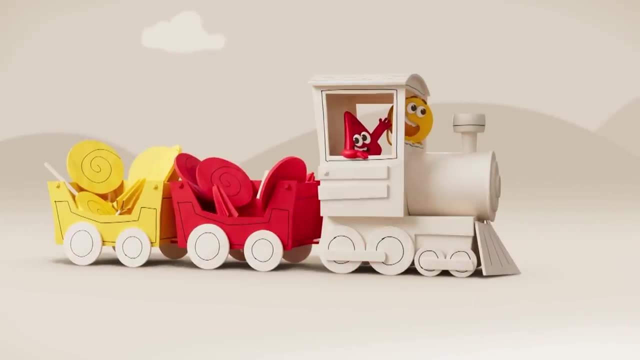 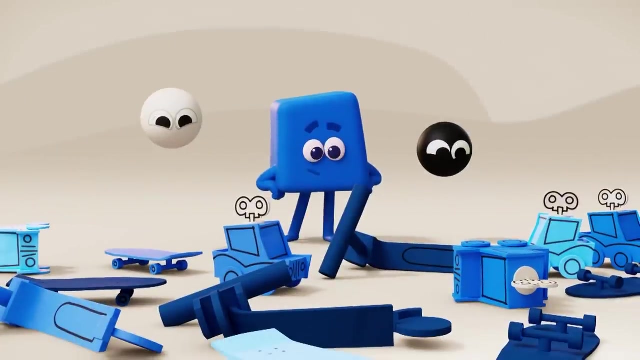 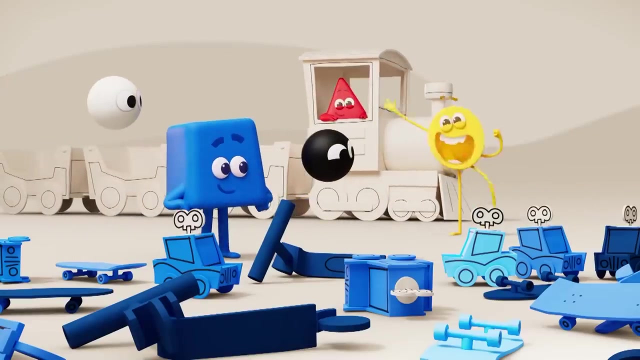 Red and yellow. Let's drop this stuff off and then look for more things to sort All aboard. the sorting express: Yes, Choo-choo, Ha-ha-ha. Red means stop. Hey friends, What are you doing? 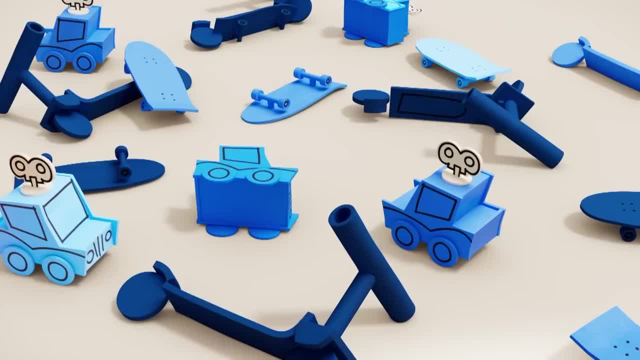 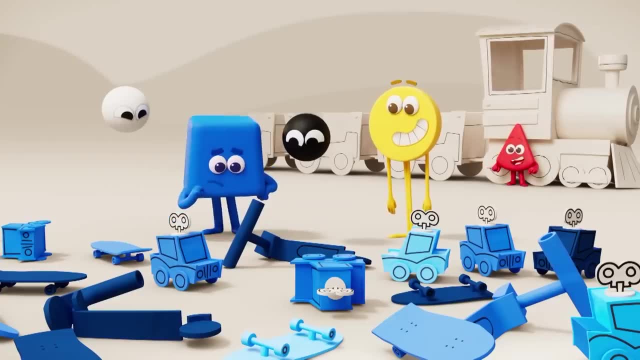 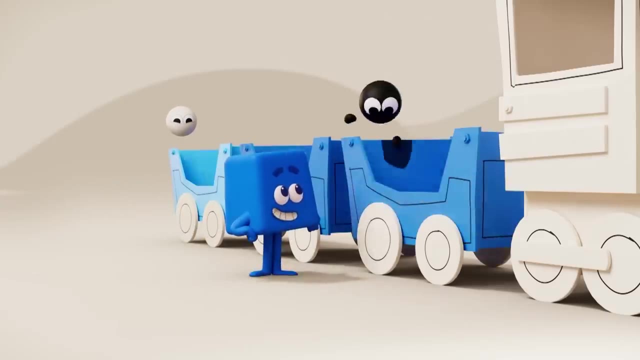 Black and white have been helping me colour my collection of cool things. Now I have light blue things, bright blue things and dark blue things, But they're all muddled up. The sorting express can sort them: Light blue, bright blue, dark blue. 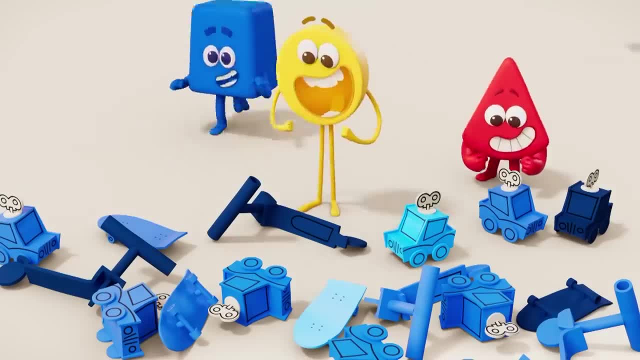 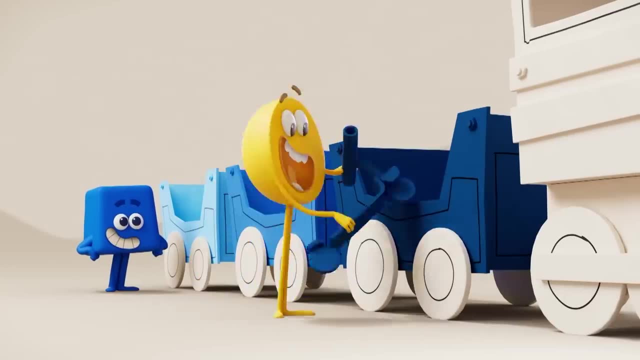 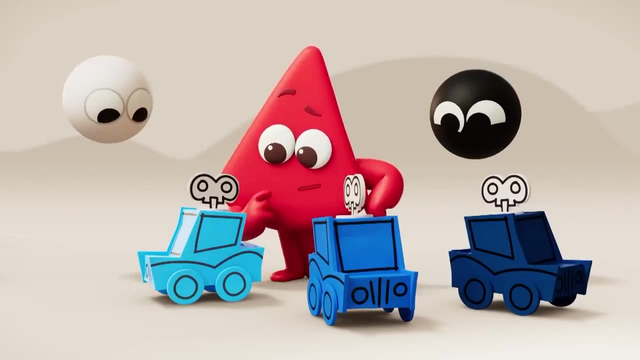 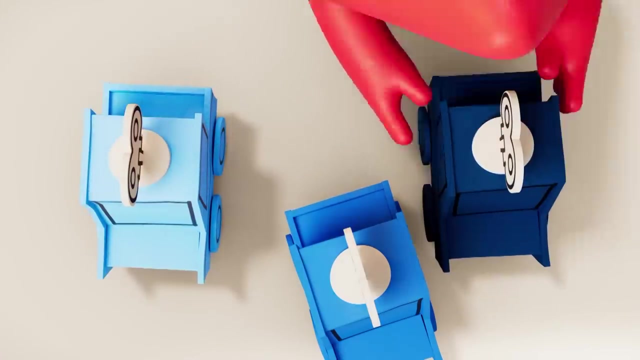 Let's get sorting, Ha-ha-ha. This skateboard is light blue, This scooter is dark blue. Three blue cars, But which one's the bright one? Hmm, This one's light blue And this is dark blue. So this one's bright blue. 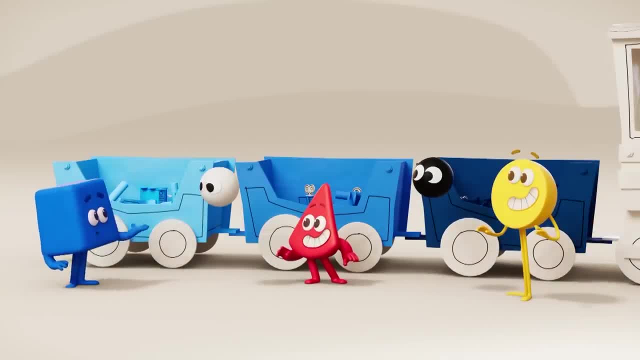 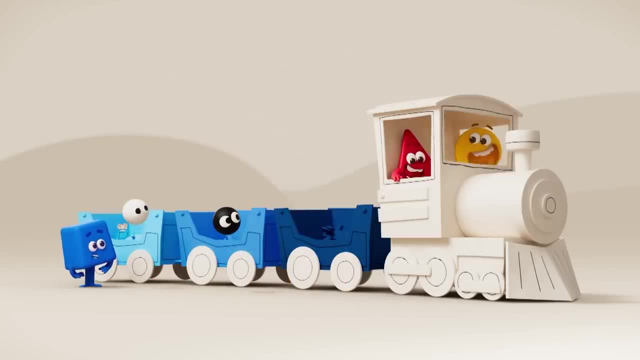 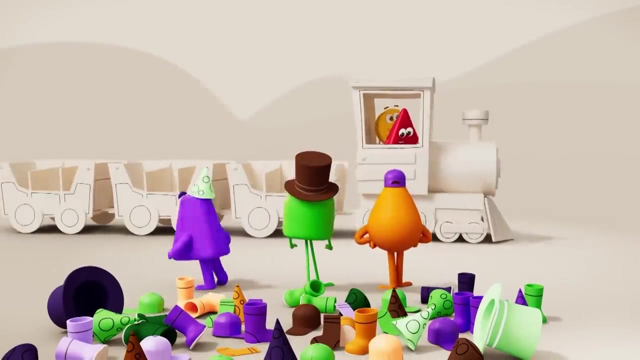 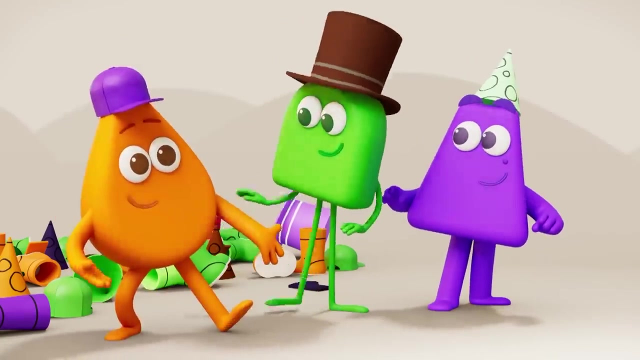 Huh, We've sorted everything into three types of blue: Light, bright and dark. Ha-ha-ha, Let's go. Red means stop. What's the problem, friends? We've had a high-energy dressing-up party: Hats, boots and socks. 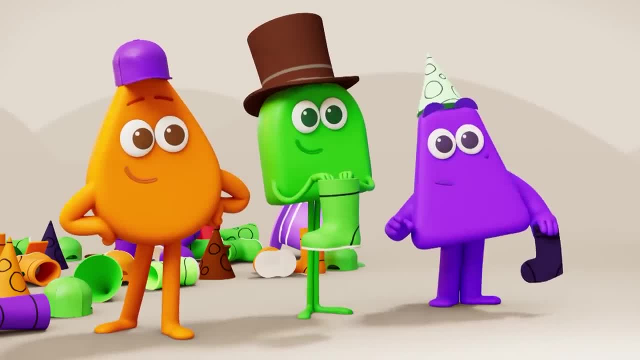 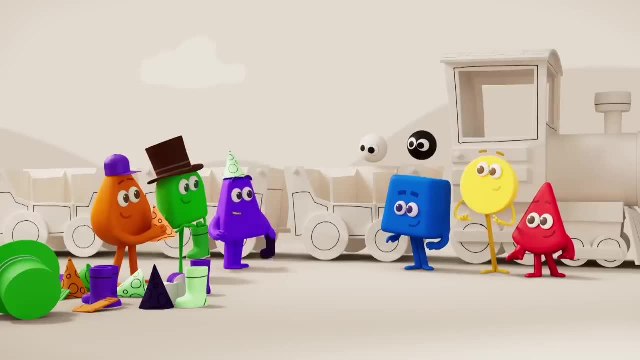 Some orange, Ha-ha, Some green And some purple, Some in light colours, Some in bright colours And some in dark colours. We got them all muddled up. Whoa, That's a big sorting job. A job for the sorting express.